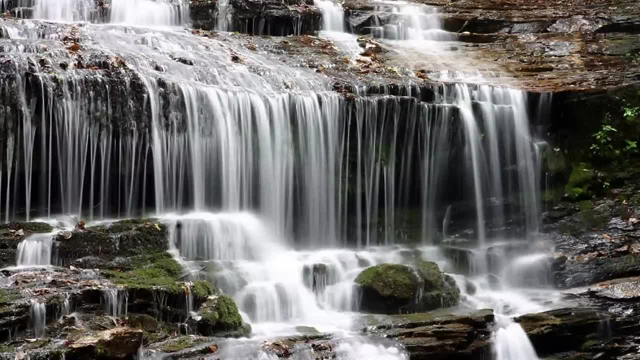 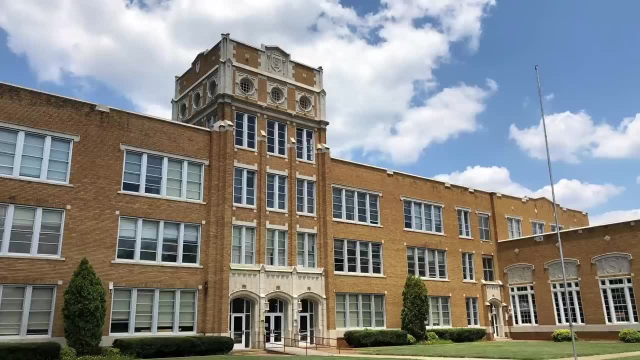 islands in the east, with millions of people living in between. It's home to beautiful scenery, a diverse population, and it is a center of banking, education and research that brings in people from around the country and the world, With its spectacular geography, important history. 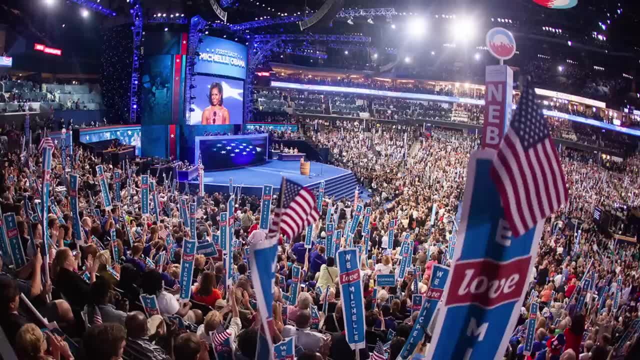 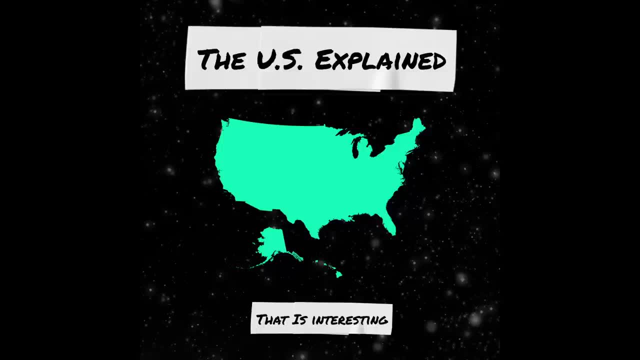 and culture and the major role it plays in the modern United States. North Carolina is a unique and fascinating state and the 12th place I'll cover in The US Explained a 56-part series on every state, territory and federal district in the country by order of admission: Hello, and. 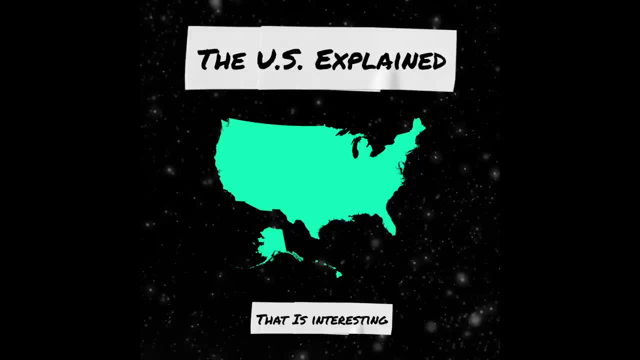 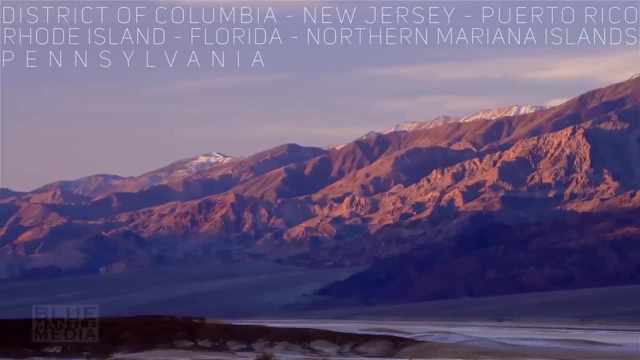 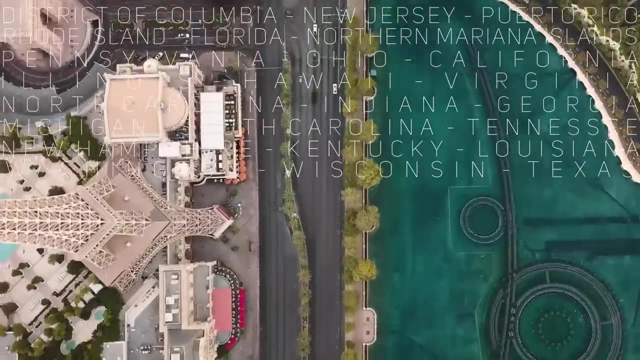 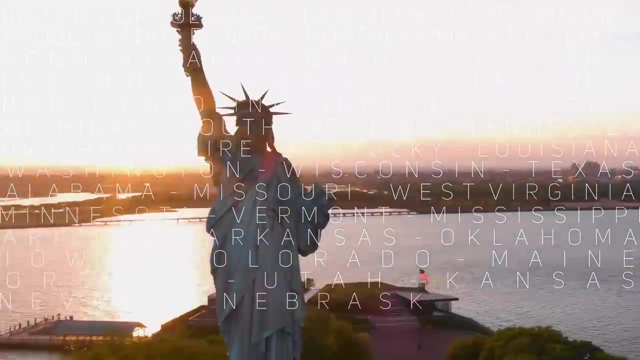 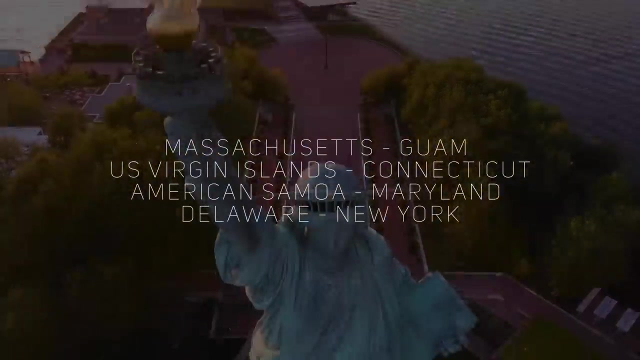 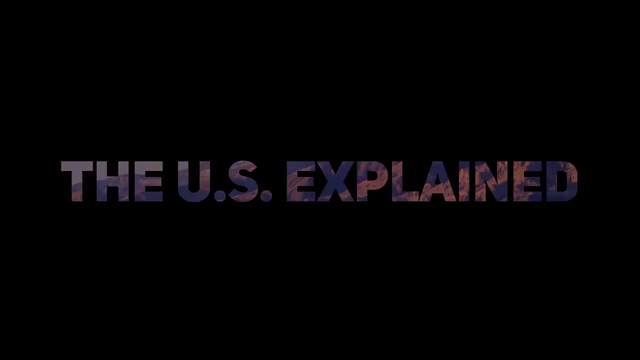 welcome to. That is Interesting. I'm your host, Carter. This is The US Explained, episode 12, North Carolina- wwwtheinvestingmovementcom. wwwtheinvestingmovementcom. According to the Kepin Climate Classification, most of North Carolina sits in a humid subtropical. 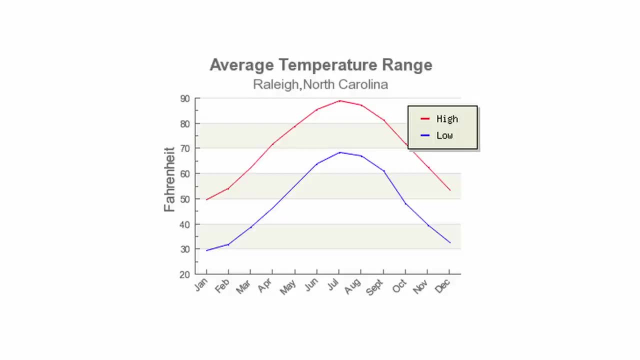 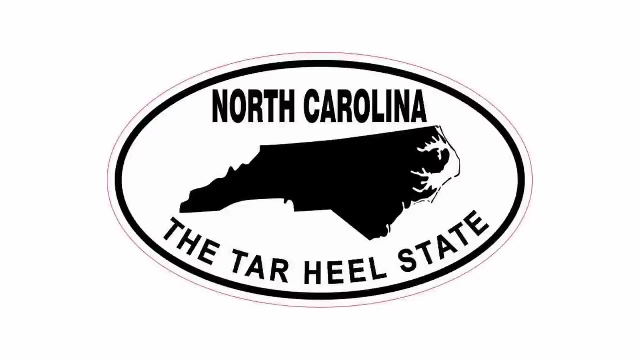 climate zone with hot summers, mild winters and a good bit of humidity. Some of the mountain regions in the west, however, are in the cooler oceanic climate zone. It's nicknamed the Tar Heel State. This unusual nickname comes from when North Carolina was a British colony. 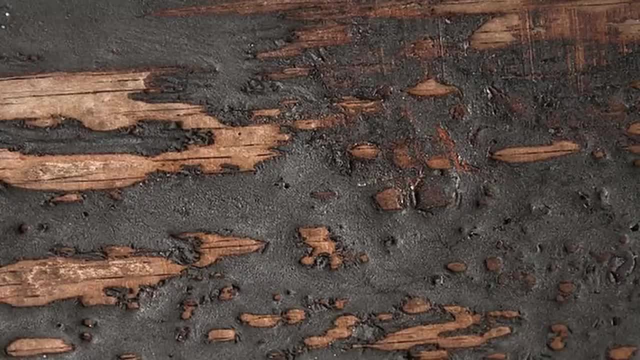 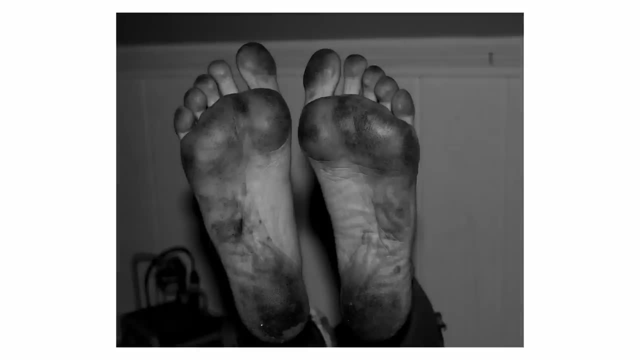 The colony was home to a number of pine forests used to produce tar to waterproof ships. The workers who harvested and produced the tar would often get it on their feet and were sometimes disparagingly referred to as Tar Heels. Eventually, however, this nickname became a term of state pride and the University. 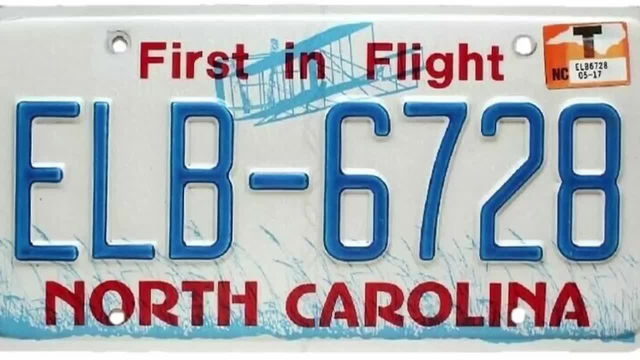 of North Carolina even adopted it as their mascot. Another nickname sometimes used for North Carolina is the subject of a really strange yet friendly feud. North Carolina's license plates have the nickname First in Flight because the town of Kitty Hawk on the Outer Banks, where the Wright brothers flew their first plane, is 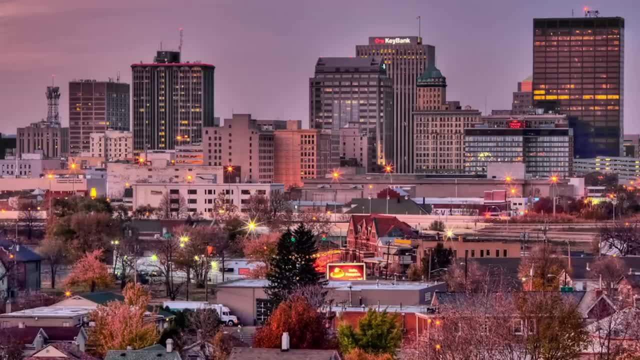 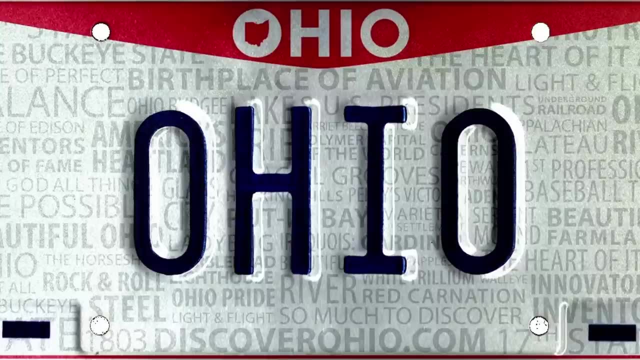 in North Carolina. However, the Wright brothers were from Dayton, Ohio, and that's where their research on the building of the planes was actually done. Because of this, both states claim their legacy as their own, and Ohio's license plates include the nickname Birthplace of Aviation. 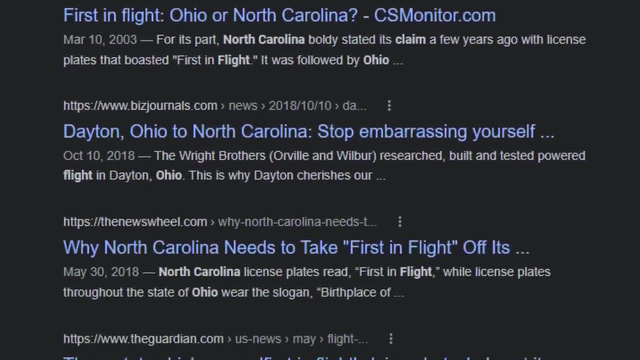 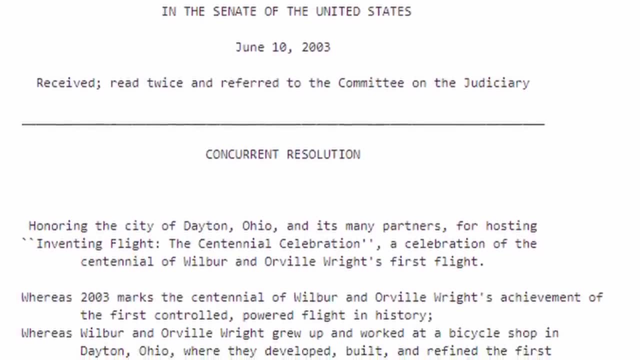 People from each state can take it pretty seriously, and I found no shortage of opinion pieces arguing that one state or the other needs to give up and change their license plate immediately. Congress even stepped in in 2003 and declared Ohio the Birthplace of Aviation. It's a friendly rivalry. 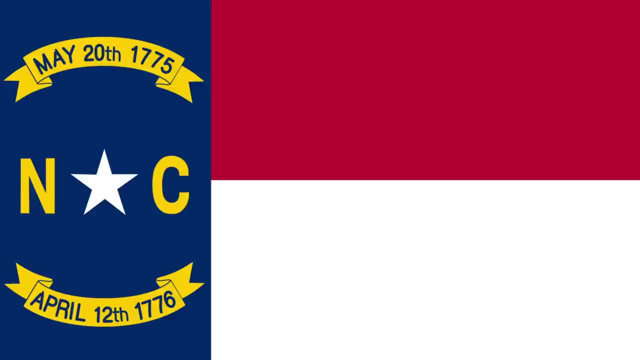 in the middle and that it doesn't go with the classic state seal on blue background design that so many states have taken up. It's not a bad looking design with a blue vertical bar, red and white horizontal bars and a star surrounded by the state's abbreviation and two. 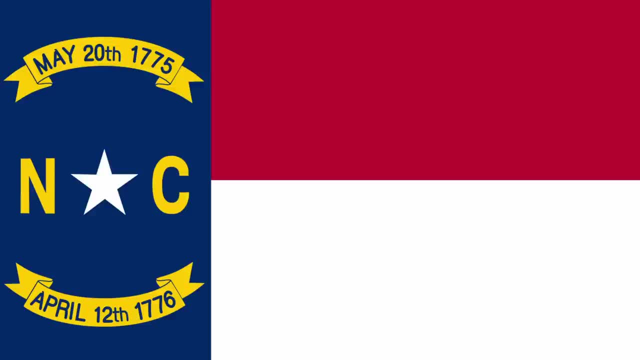 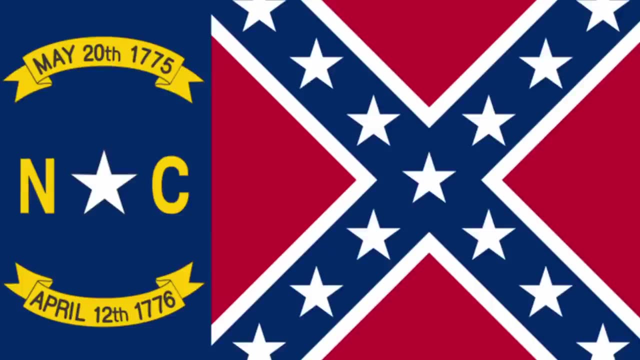 ribbons. My biggest complaint with North Carolina's flag, though, is that it is based off of the flag the state used when it was part of the Confederacy, a trend that is, unfortunately, still very common among southern flags. The two dates on each of the ribbons are pretty significant as well. 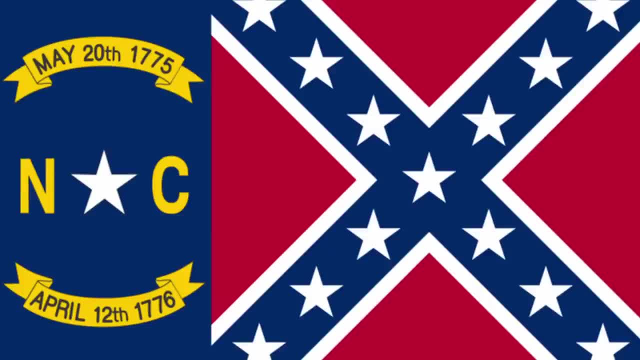 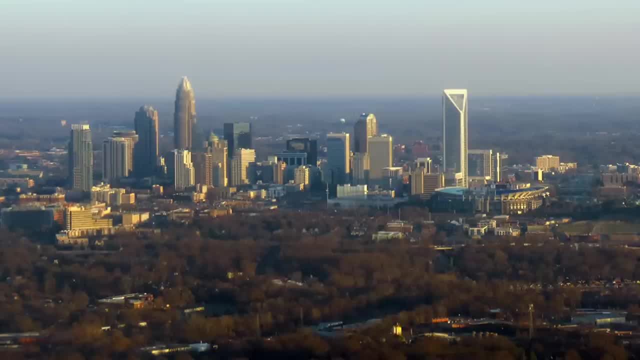 The ribbon on the top bears the date of May 20th 1775, the supposed date of the Mecklenburg Declaration of Independence. Mecklenburg County is the county where Charlotte is located. As the story goes, on May 20th 1775, a group of Charlotte residents who'd heard news of the Battle of 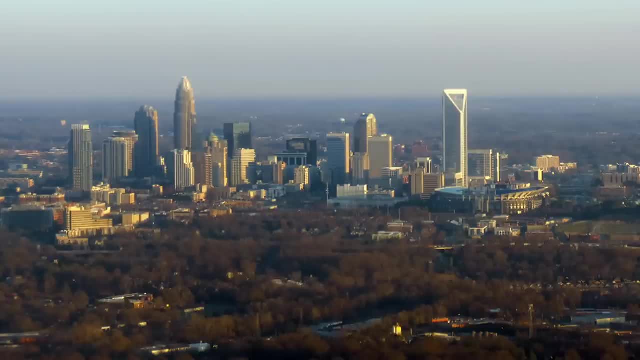 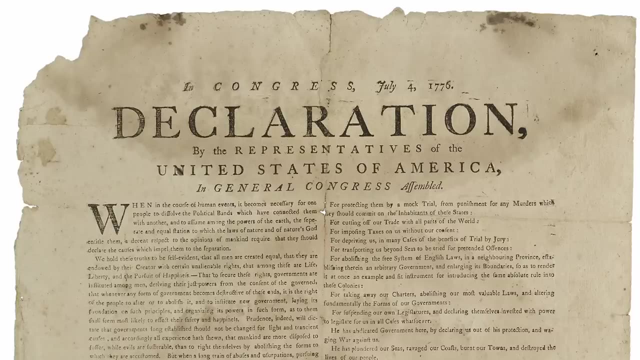 Lexington met and signed a Declaration of Independence. If the story is true, this would mean that the Mecklenburg Declaration of Independence is older than the more well-known Declaration of Independence by more than a year. The only problem is that it was published a good 44 years later, so there's no telling whether the document is authentic or 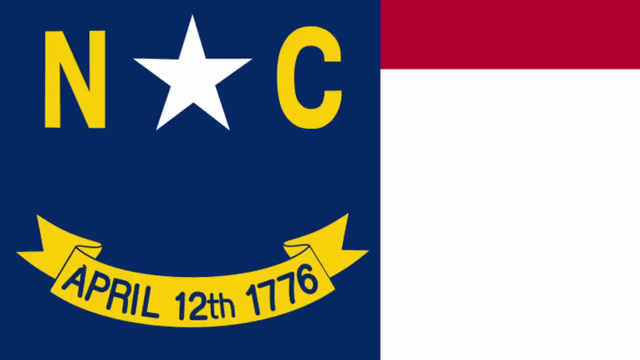 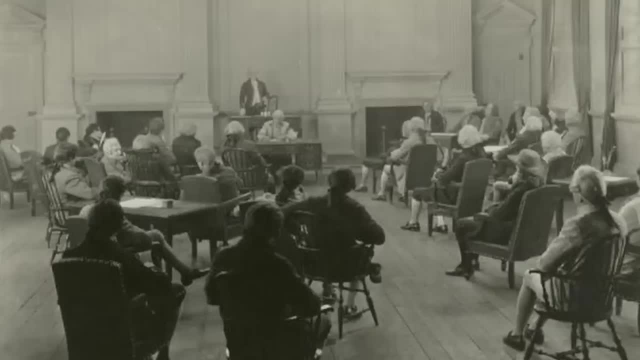 not The bottom date, April 12th 1776, is an event that we do know happened: the signing of the Halifax Resolves. They were signed by the Provincial Congress, essentially a North Carolina rebel government- that met during the lead-up to the Revolutionary War. During one of their 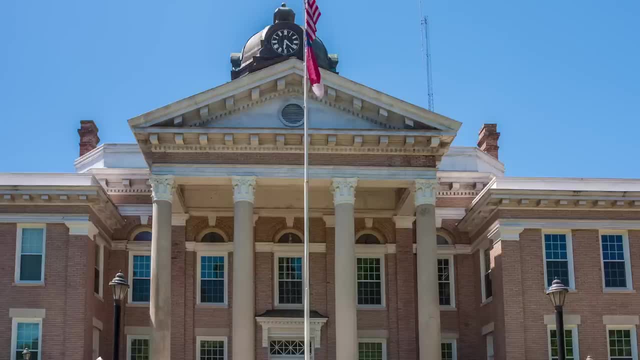 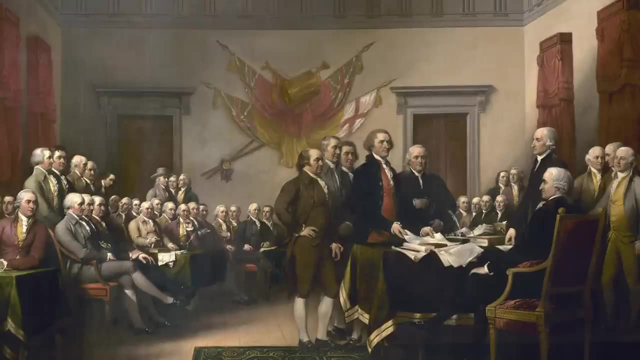 meetings in the town of Halifax. they voted to allow the delegates they'd sent to the Second Continental Congress to vote in favor of declaring independence from Britain. They were the first of any colony to do this, and so it was the first time in the history of the 13 colonies that any sort of government had approved the idea of independence from Britain. North Carolina is on the medium to smaller side of states in terms of area, coming in at number 29, with an area of 48,000 square miles or 126,000 square kilometers. This makes it slightly smaller. 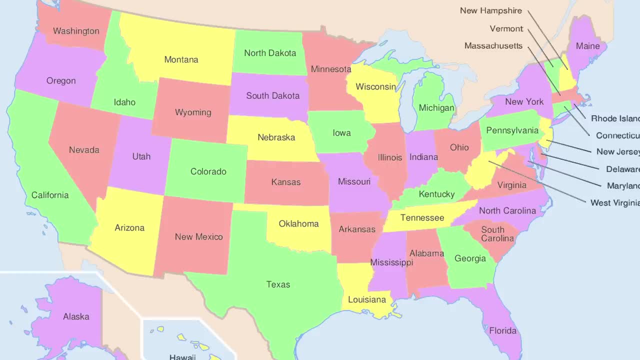 than Alabama, but slightly larger than New York. However, most of the states larger than it are further to the west and, compared to its neighbors, North Carolina seems pretty similar in size or even a little larger. In fact, it's the third largest state on. the east coast, with only Georgia and Florida surpassing it. In terms of population, North Carolina ranks much higher, home to 10.439 million people, making it the eighth most populous state in the entire country and one of just 10 states home to more than 10 million. residents Only. California, Texas, Florida, New York, Pennsylvania, Illinois and Ohio have more people living within their borders than North Carolina. This helps give the state a population density of 215 people per square mile or 83 per square kilometer. a similar population density to Romania, Senegal or Morocco. Due to the state's geography, most of these residents live in the middle of the state, which I'll get to later, giving that region an even higher density and more urbanized feel, whereas the east and west are more rural. 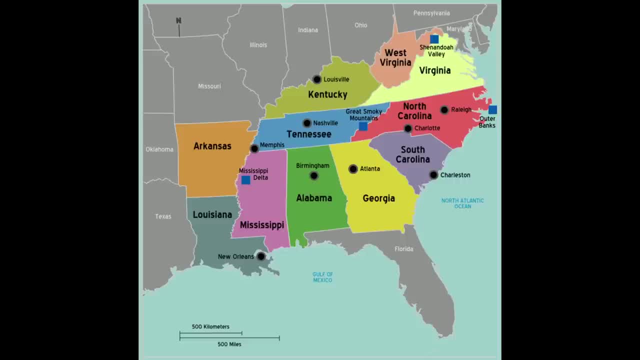 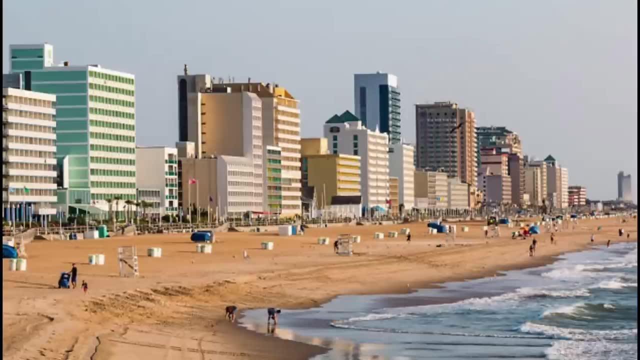 North Carolina is located squarely within the southeastern US, a region known as the South, and borders four other states as well as has a coast on the Atlantic Ocean, and the north sits in Virginia, which it shares a mostly straight 320-mile border with. 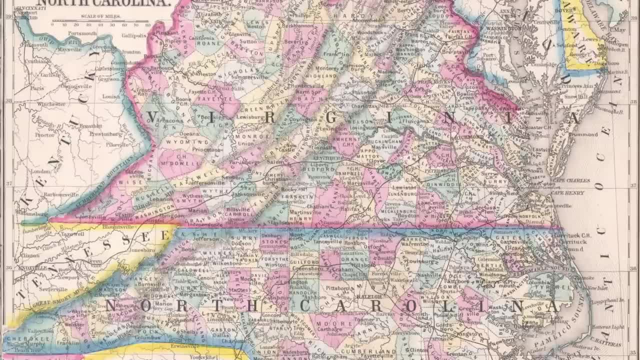 extending east-west from the Atlantic coast on Currituck Banks, a narrow peninsula that makes up the start of the Outer Banks all the way to a point in the mountains in Ashe County where it turns to the southwest and becomes a border with Tennessee. Depending on where you live, they're. 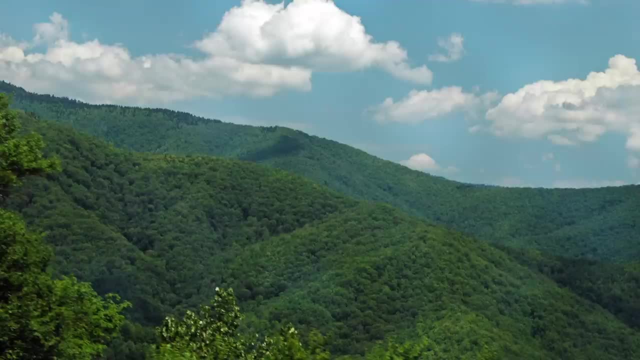 either pronounced Appalachians or Appalachians. It's more of a north-south divide. I'm originally from Pennsylvania, so I've always called the mountains in the region I'm from Appalachian and Appalachia, and that's how I'll be saying it in this video. 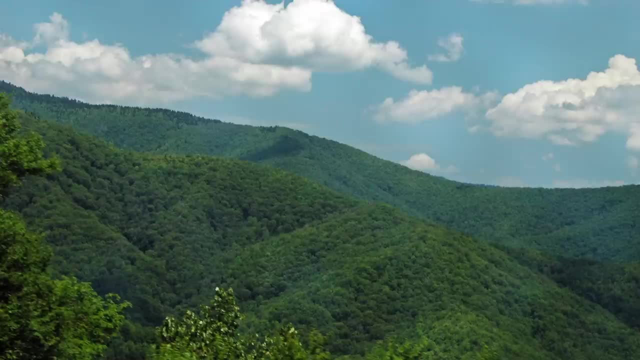 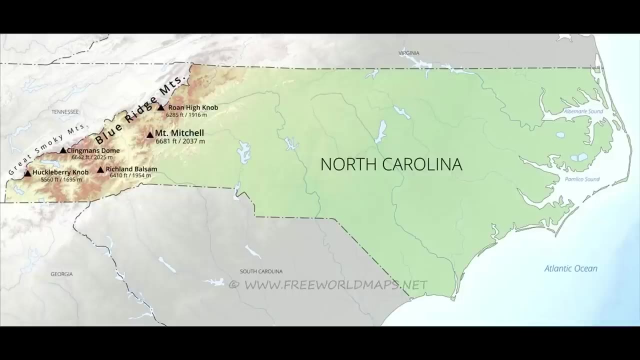 because that's what I'm used to, But in North Carolina most people pronounce it Appalachian and Appalachia. The North Carolina-Tennessee border weaves through the Appalachians, following the general path of the mountain range for around 185 miles to a spot near the town of 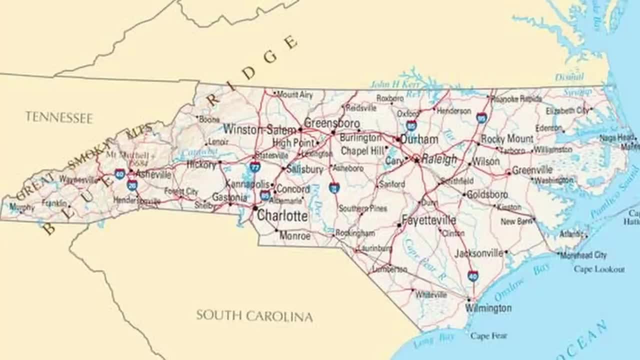 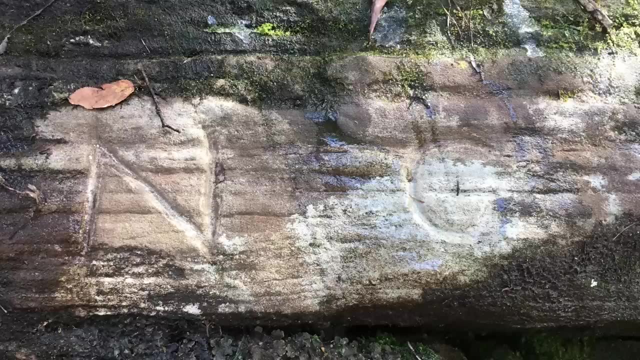 Wolf Creek where it meets the border with Georgia. The border with Georgia is around 68 miles long and follows an east-west line straight to a rock in the Chattooga River called Ellicott Rock. There it becomes a border with South Carolina and heads in a diagonal, somewhat weaving line slightly to. 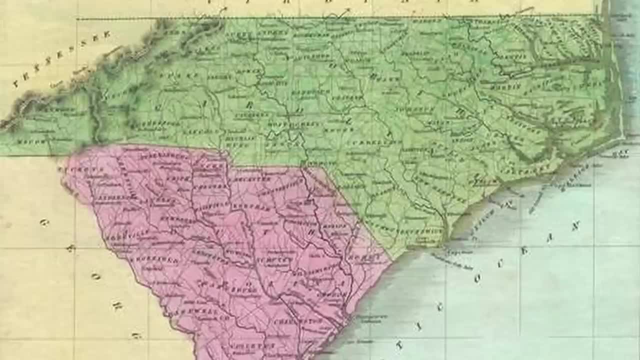 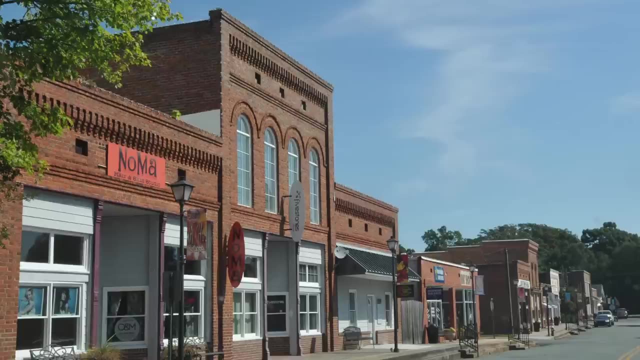 the east. It then becomes a straight line, heading east for 70 miles till it reaches the Catawba River, just outside of Charlotte. It cuts in a strange path, though headed generally southeast, through a region known as the Waxhaws, at times going through the suburbs of Charlotte and placing 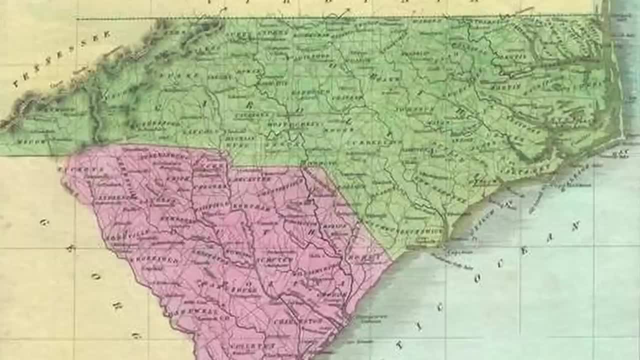 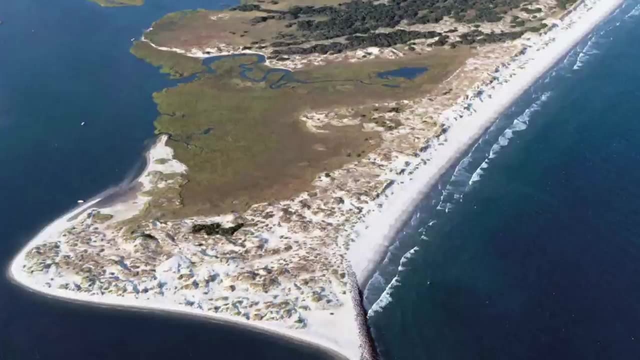 some of them in South Carolina. From there it then heads east for 63 miles and southeast for 92,, meeting the Atlantic at a barrier island called Bird Island, not far from the suburbs of the South Carolina city of Myrtle Beach. The geography of North Carolina is pretty. 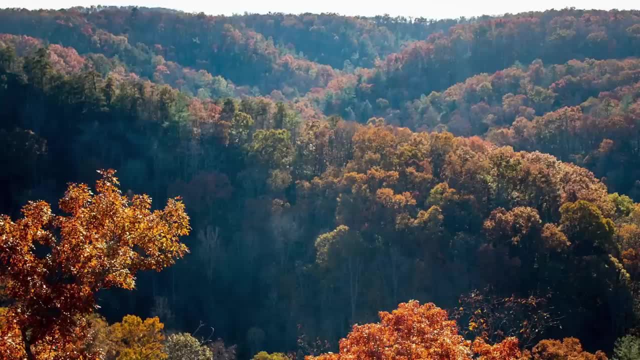 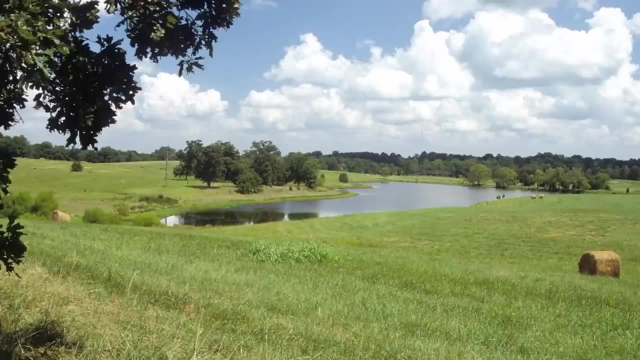 straightforward. It has a natural barrier on each end. The Appalachians sit to the west and the Atlantic to the east. The land in between is the Piedmont rolling hills and flat farmland where most North Carolinians live, with rivers flowing through the mountains to the sea. Further, 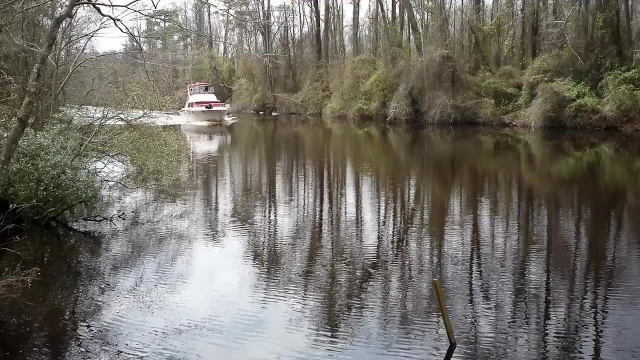 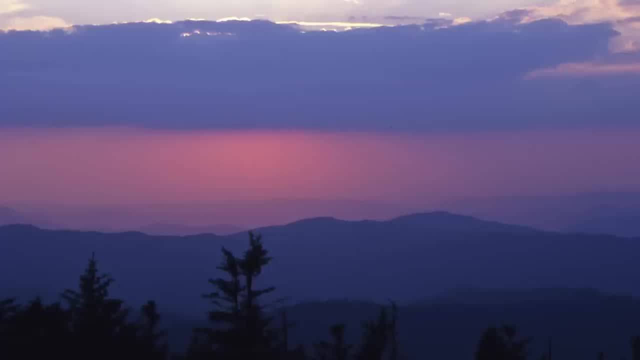 east and closer to the ocean it becomes the flatter, at times swampy, coastal plain. The Appalachians cut all the way from Alabama through the entire east coast, through Maine and into New Brunswick and Quebec. They're the predominant mountain range of the eastern US, but their 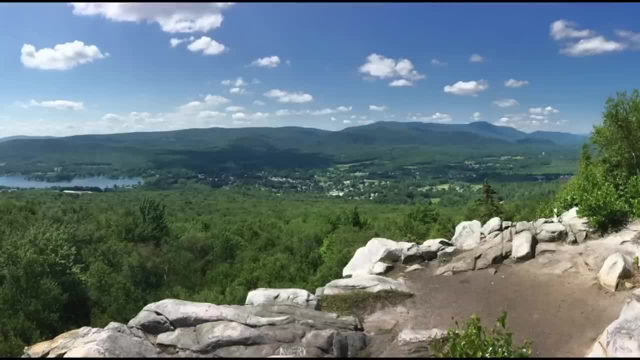 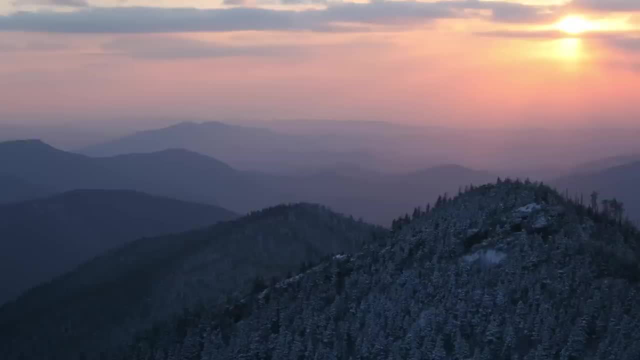 region and, in many places, eroded down. In states like Massachusetts, for example, they look more like rolling hills than mountains. However, in North Carolina, it's a different story. The western part of the state is dominated by the Great Smoky Mountains, or simply the Smokies. 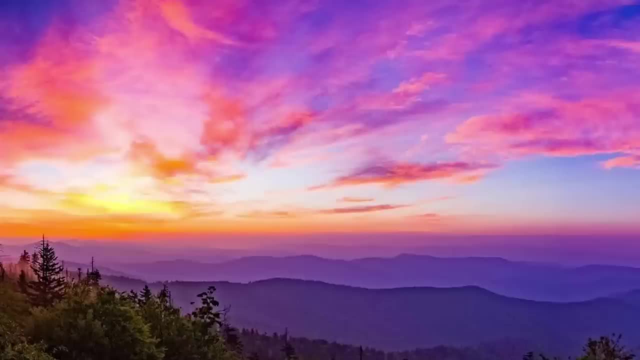 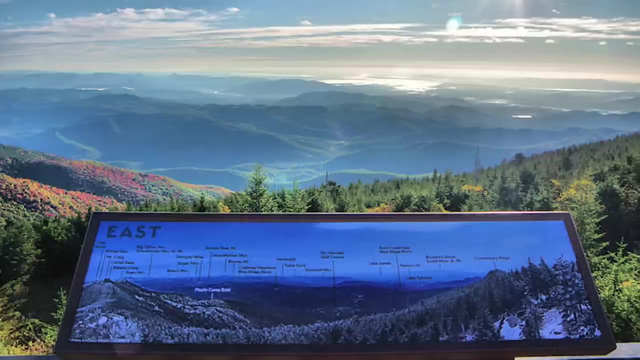 far and away the tallest part of the enormous mountain range. In fact, of the ten tallest mountains east of the Mississippi, nine are located in North Carolina, the one exception not far across the border, in Tennessee. It includes peaks like Mount Mitchell which, at 6,684 feet, is the tallest mountain in the state and the tallest in the Appalachians. as well as the highest point in the US east of the Mississippi, as well as other famous mountains like Clingmans Dome. It's home to one of the few national parks in the eastern US- Great Smoky Mountains National Park, which it shares with Tennessee and is home to a large 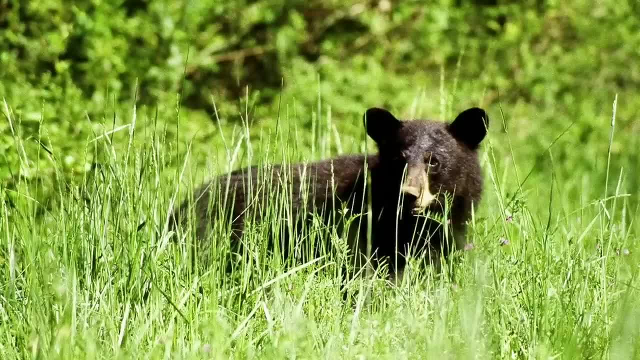 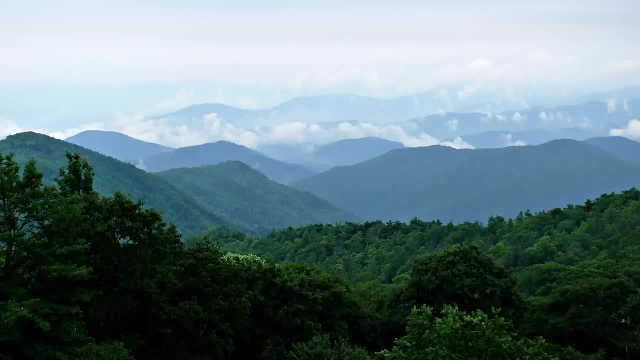 population of black bears. Forested and mountainous, the western part of North Carolina is relatively sparsely populated, Despite taking up a sizable chunk of the state. 1.189 million people live in North Carolina's Appalachians, or around 11% of the state's. 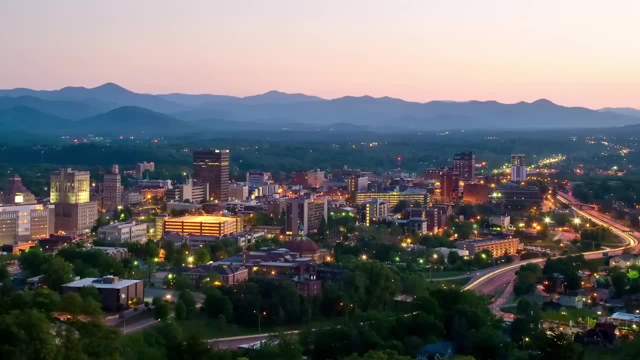 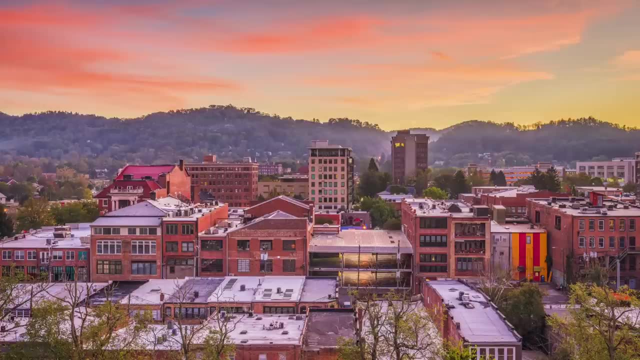 population. Many of them live in Asheville, the state's seventh-largest urban area. home to 280,000 people and tucked in a small river valley in the mountains, Asheville, a popular tourist destination, is one of the rare examples of a city, even a small one. that sits right amongst the Appalachians. For the most part, the Appalachians of North Carolina remain a sparsely populated wilderness. However, that doesn't mean they're empty. Tourists flock to the Great Smoky Mountains, like the Great Smoky Mountains, and the Great Smoky Mountains, like the 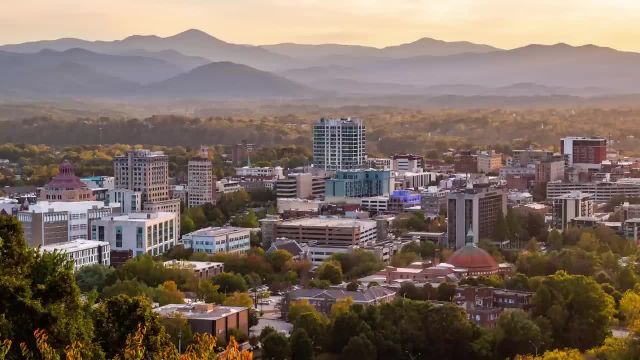 Appalachians, like perhaps no other part of the Appalachians, and their region has built up a tourism-centered economy. Asheville, not even in the 100 largest urban areas in the country, gets 10 million tourists every year- many times the number of visitors than other urban areas of. 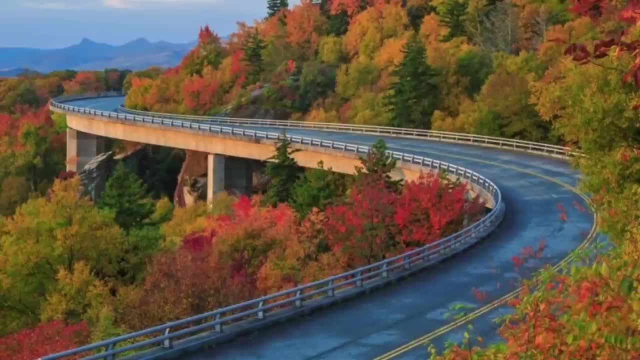 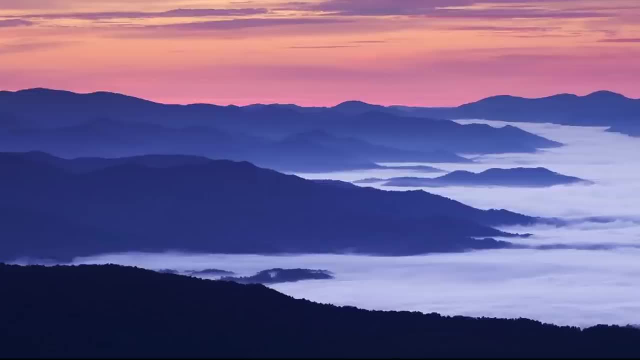 its size, The most visited site run by the National Park Service has consistently been, throughout its history, the Blue Ridge Parkway, a scenic road which runs through the Blue Ridge Mountains from Great Smoky Mountains National Park to Shenandoah National Park in Virginia. 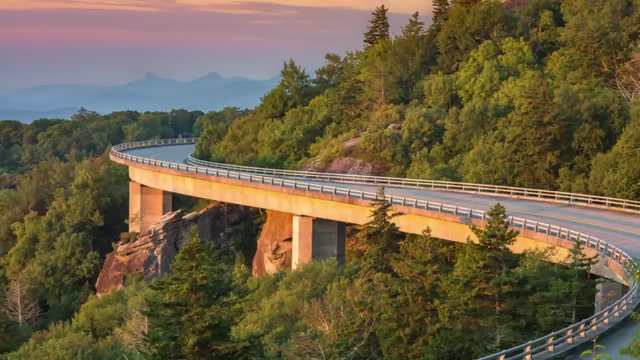 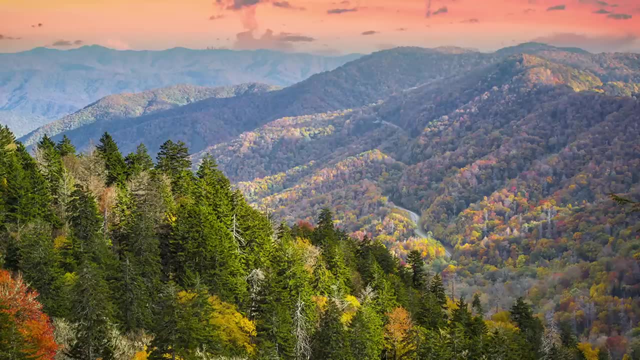 Great Smoky Mountains is one of the most visited national park sites in the country. The Great Smoky Mountains National Park itself is one of the most visited national park sites in the country, bringing in 14 million tourists every year. Chimney Rock, near Hendersonville, is another. 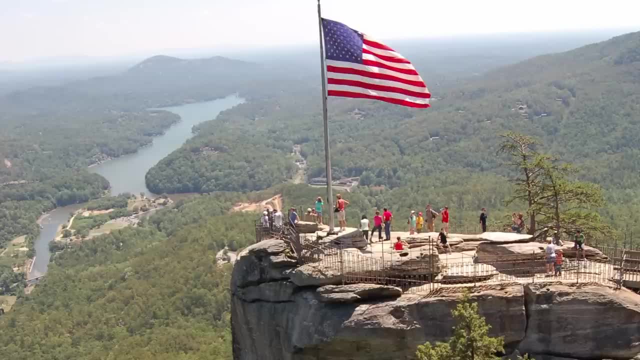 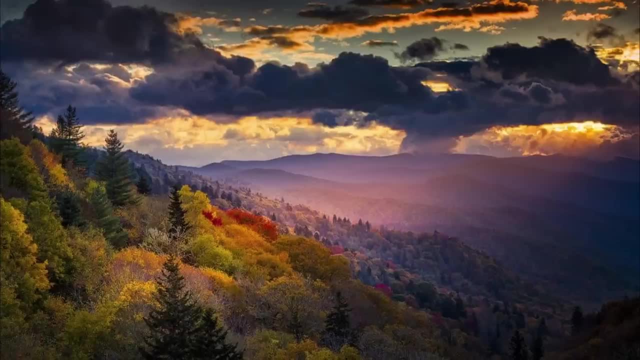 beautiful and popular spot in the Appalachians, and the Appalachian Trail runs through the state, criss-crossing between it and the state of Tennessee. Though not as famous as parks like Yellowstone, Yosemite or the Grand Canyon, the Great Smoky Mountains and the 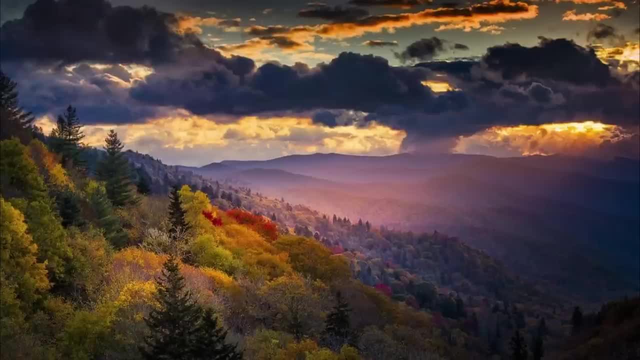 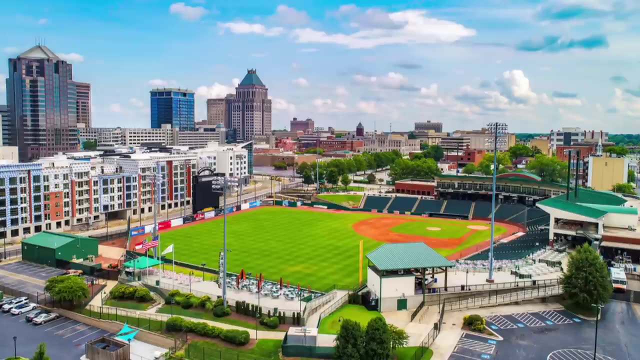 mountains and forests of western North Carolina have the advantage of being a large and protected that still sits just a few hours from the urban centers of North and South Carolina, Tennessee, Virginia, Georgia and other states. This recreational and tourism focus also continues in the Smokies across the border in Tennessee. 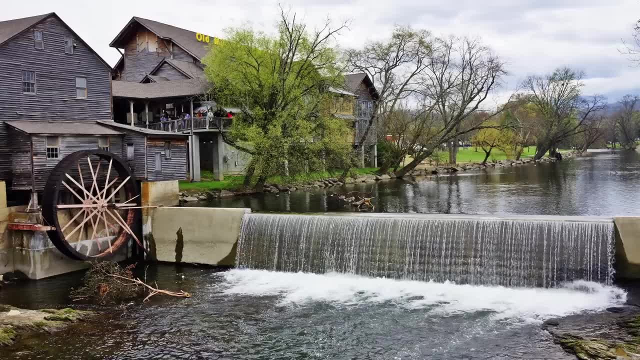 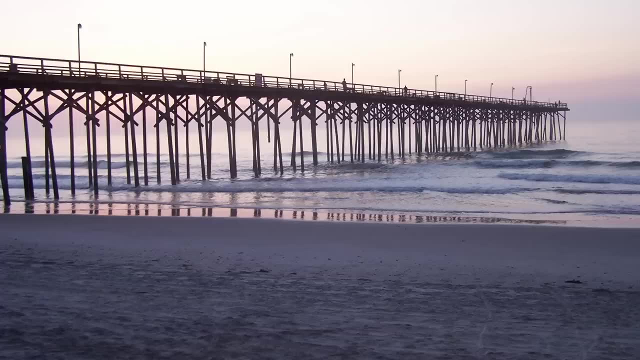 where towns like Gatlinburg and Pigeon Forge are famous tourist destinations that bring in millions of visitors each year. The beauty of the Appalachians, coupled with the large number of visitors who go to the North Carolina coast and the cities of the Piedmont. 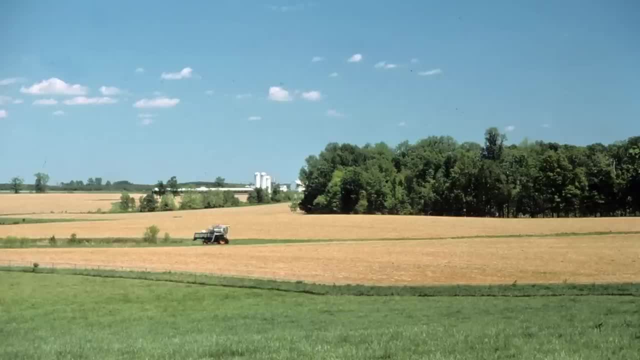 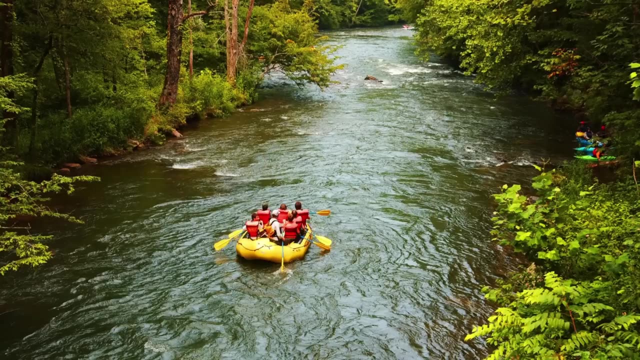 help make North Carolina the sixth most visited state in the country, after only Florida, California, New York, Nevada and Pennsylvania. Some of the rivers in the Appalachians flow west into the watershed of the Ohio River, The French Broad River, for example, which flows through Asheville. 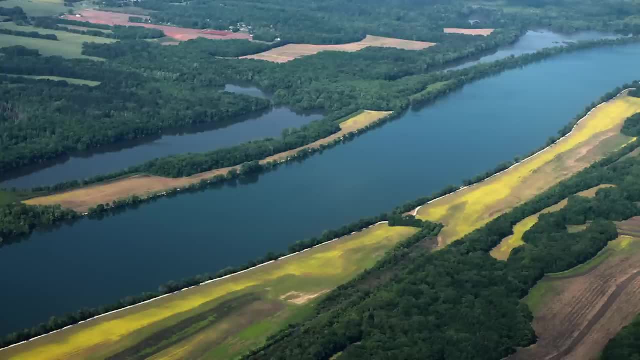 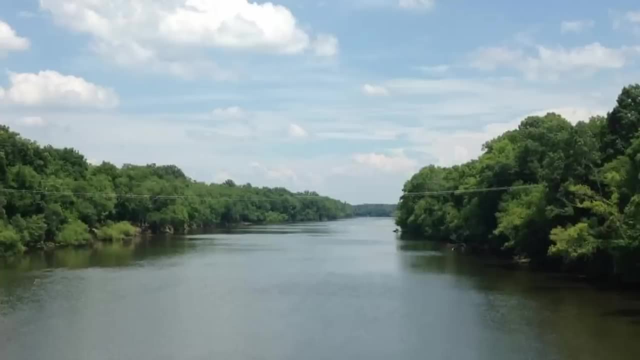 is one of two rivers whose confluence creates the Tennessee River. Most of the rivers in the state, though, such as the Roanoke, Peaty, Neuse, Catawba and Cape Fear Rivers, all flow southeast, from the mountains to the Atlantic. 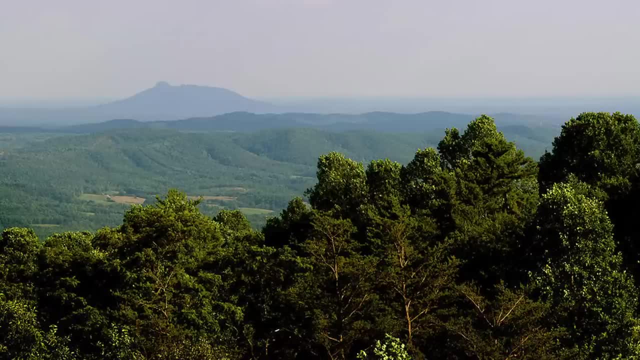 They flow across the Piedmont, a plateau of low rolling hills covered in a mix of farms and forests, where most of North Carolina is populated. Most of the rivers in the state, though, such as the Roanoke, Peaty, Neuse, Catawba and Cape Fear Rivers. 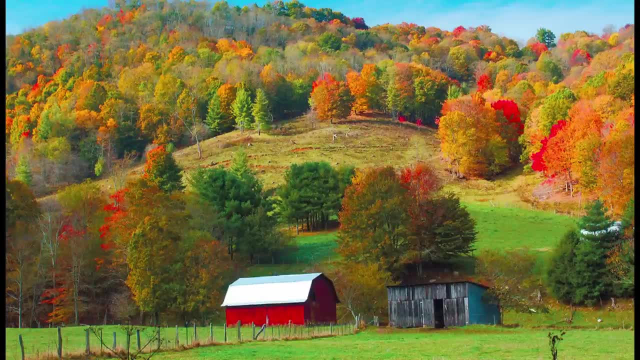 all flow southeast from the Appalachians. Most of the rivers in the state, though, such as the Roanoke, Peaty, Neuse, Catawba and Cape Fear Rivers, all flow southeast from the Appalachians, Though the terrain is mostly pretty gentle, especially the closer it gets to the coast. 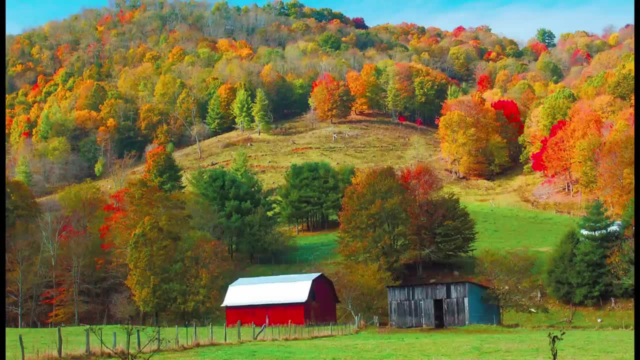 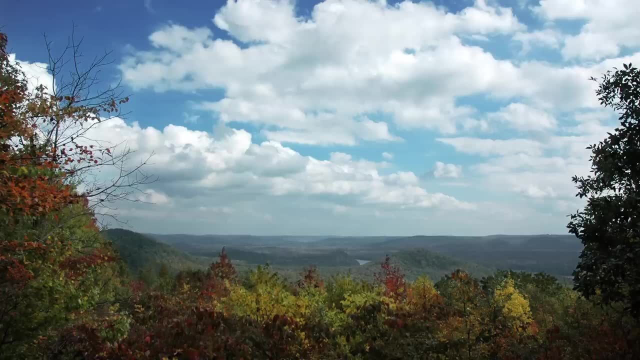 there are a number of small mountains and mountain ranges detached from the Appalachians that seemingly spring up out of nowhere, such as the Sorretown Mountains and the Uwaris, both remnants of ancient mountain ranges. Another strange geographic feature are the Carolina Bays. 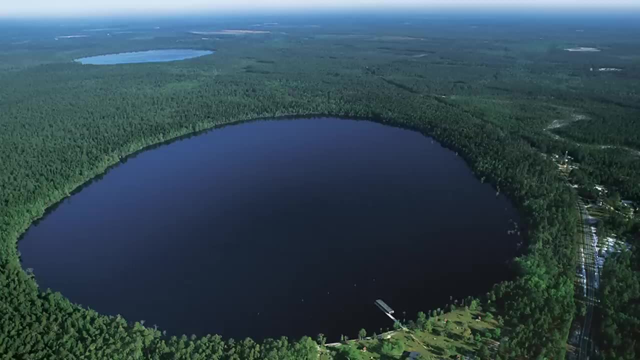 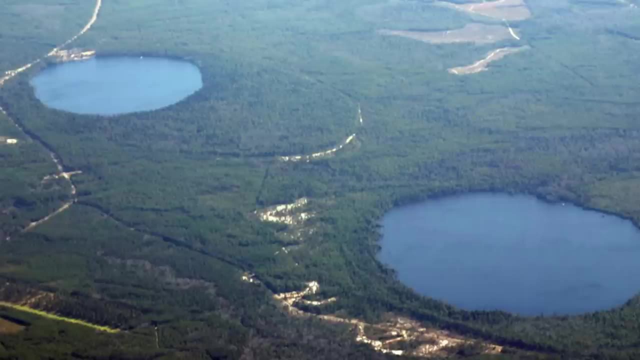 these unusual oval-shaped depressions that you can find everywhere in the flatter parts of the state and throughout other states in the East Coast. There's not a clear consensus on where they come from, and I'll probably make a video on them in the future. 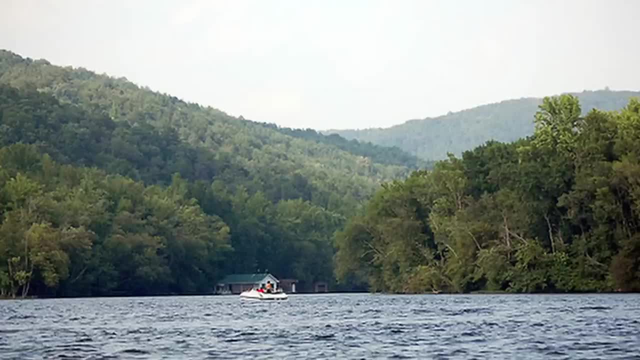 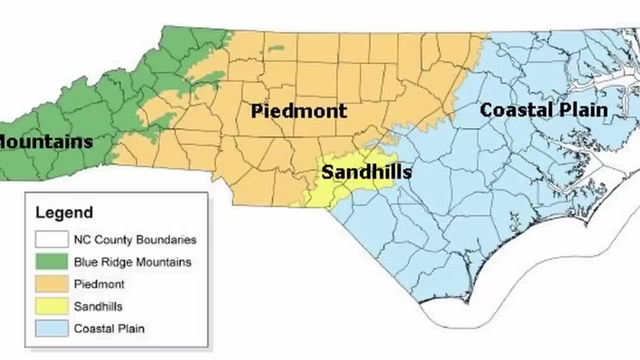 Most people wouldn't think that there are mountain ranges in the US that lie east of the Appalachians, but the Uwaris and Sorretown Mountains are there to prove you wrong. The Piedmont is the heart of North Carolina. Though it takes up only around a third of the state's area, it's home to two-thirds of its population. 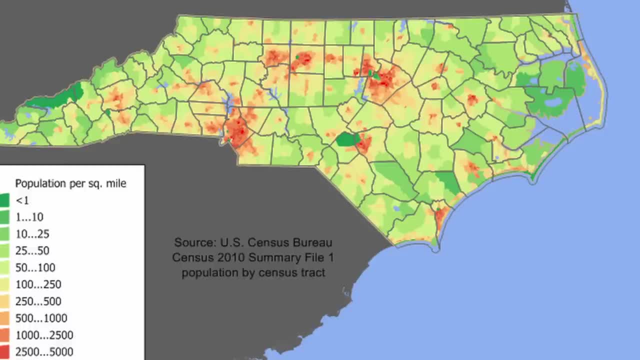 6.862 million people call the Piedmont of North Carolina home, and the six most populous urban areas in the state all lie within it. It has such a large population for a number of reasons. First off, its topography isn't bad. 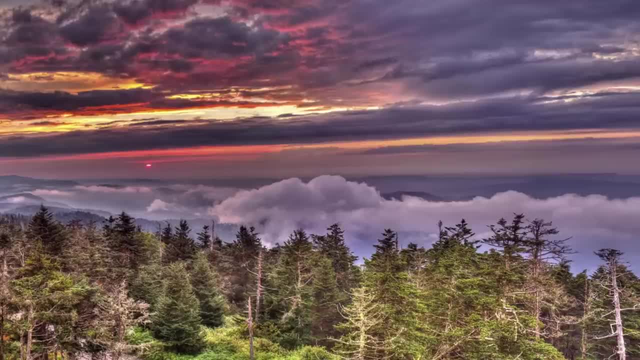 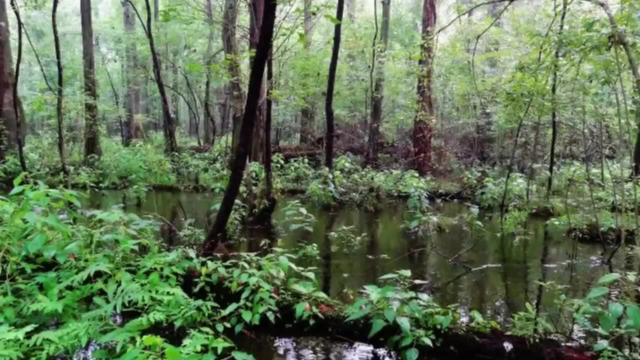 It's a little hilly, but nothing that challenges settlement like the Great Smoky Mountains. Meanwhile, the coastal plain, though flatter, is dominated by wetlands, and because of that hard-scale development isn't a big possibility either. 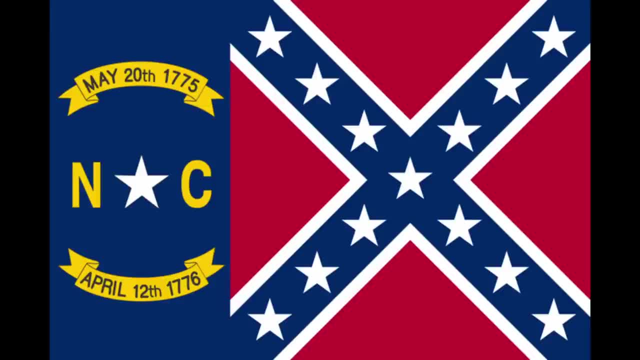 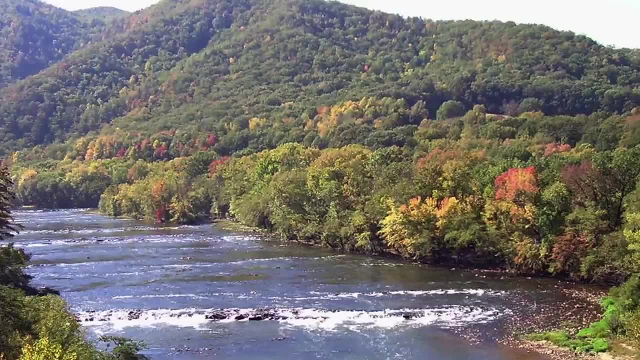 This makes the Piedmont really the only part of the state able to house a large population. In addition, the change in elevation caused by the plateau means that many of the rivers that cross the Piedmont were fast-moving and suitable for milling, especially along the fall line, the spot where the Piedmont drops off to the coastal plain. This, alongside all the farms, makes the region turn the Piedmont into an industrial powerhouse and helps spark its growth. Today, it's home to a number of different industries. Charlotte is the biggest American banking center outside New York and the cities of Raleigh, Durham and Chapel Hill, which sit close together in a cluster. 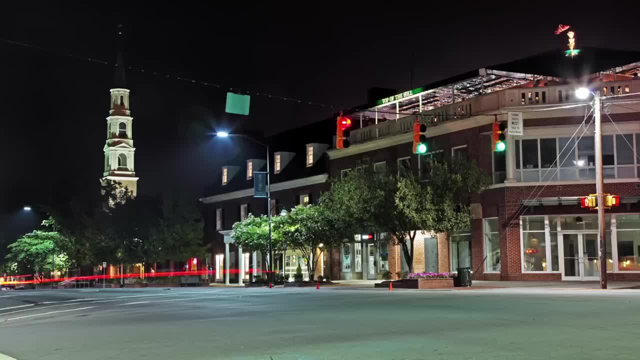 are collectively known as the Research Triangle, Filled with graduates from nearby universities. it's a fast-growing, high-earning tech and education hub that brings in people from all over the country and the world. Agriculture, specifically, the tobacco industry, of which North Carolina is the center. 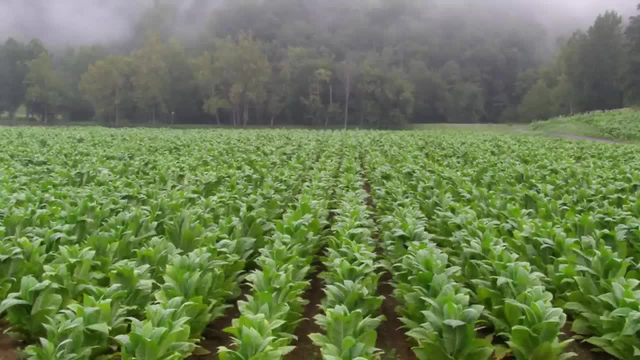 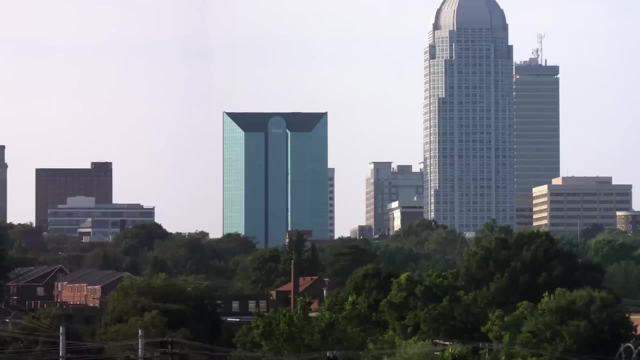 is still huge, and farms alongside forests criss-cross the region. In the north sits a string of four cities, almost in two clusters. Furthest to the west sits Winston-Salem, which, with 391,000 people, is the third-largest urban area in the state. 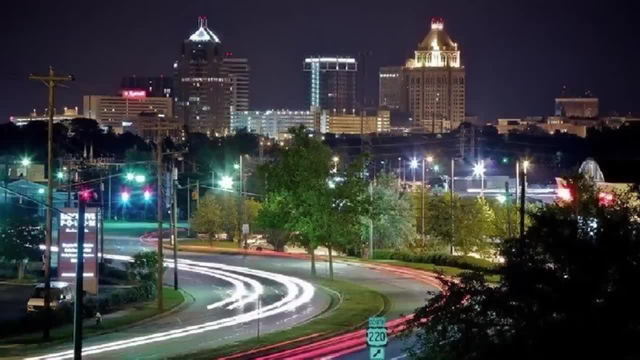 Just to the east sits Greensboro. the downtowns of the two cities just 25 miles apart. Neither city is a suburb of the other and they aren't close enough that they make up a singular urban area like, for example, Minneapolis and St Paul. 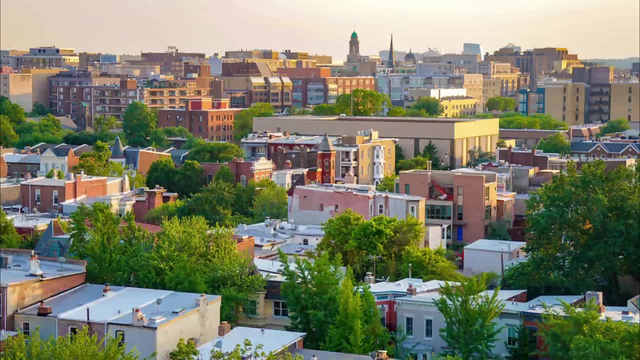 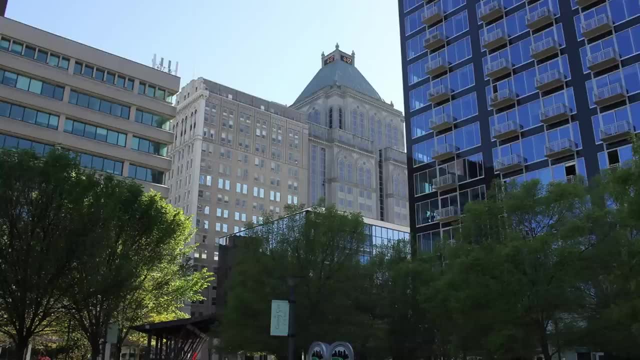 Rather I'd compare them to Baltimore and Washington DC, cities which are separate and distinct but still close by and whose suburbs at times overlap. Greensboro is the fifth-largest urban area in the state, home to 311,000 people. 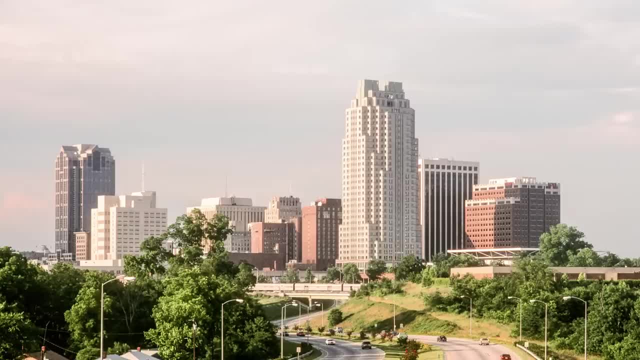 Charlotte and Raleigh, North Carolina's two main cities, are large but not enormous, and North Carolina's huge population can't be attributed to them alone. It's helped in large part by the sheer number of smaller cities like Asheville, Winston-Salem, Greensboro and others. that together give the state so many residents. Another one of these small cities is Denver. Durham, which is home to 347,000 people, is the state's fourth-largest urban area. Similar to Greensboro and Winston-Salem. it sits near and has overlapping suburbs with another city, Raleigh. their downtown's about 20 miles apart. Unlike Greensboro and Winston-Salem, Raleigh, North Carolina's capital, is more than twice the size of Durham, home to 885,000 people, which makes it the second-largest urban area in the state and the 50th-largest in the country. 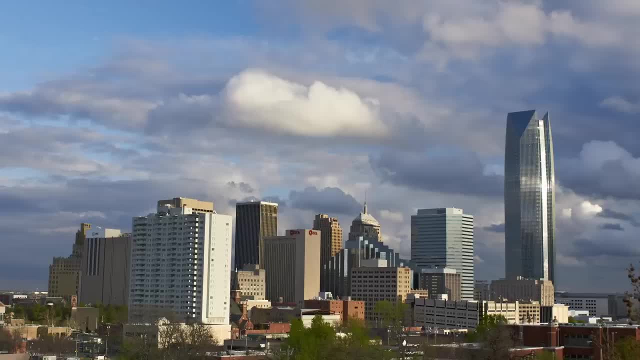 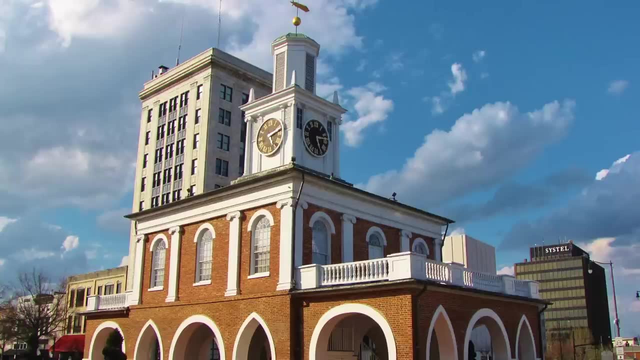 a little smaller than New Orleans and a little larger than Oklahoma City. Southwest of Raleigh, sitting on the fall line of the Cape Fear River, sits Fayetteville, the sixth-largest urban area in the state, slightly smaller than Greensboro with 310,000 people in its urban area. It's best known as the home of Fort Bragg, which, by population, is the largest military base anywhere on Earth, with 57,000 troops, or 10% of the entire US Army, stationed there, more than the active-duty forces of 117 different countries. 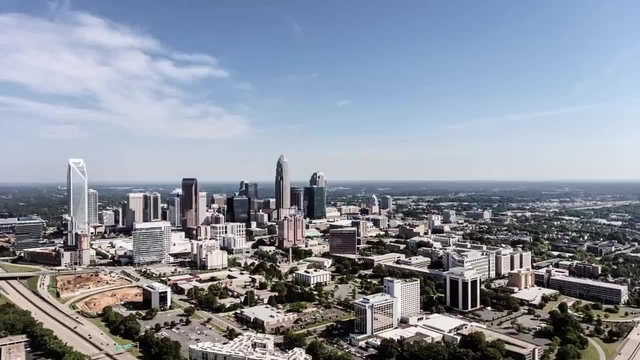 The last major city of the Piedmont is, of course, Charlotte. it sits near the Catawba River and the border with South Carolina, and a decent chunk of the city's suburbs even stretch into South Carolina, Home to 1.249 million people in its urban area. it's the largest in the state and the 38th-largest in the country, home to slightly more people than Providence and slightly less than Austin Altogether. Charlotte and its suburbs are home to more people than all of the entire Appalachian region of the state. 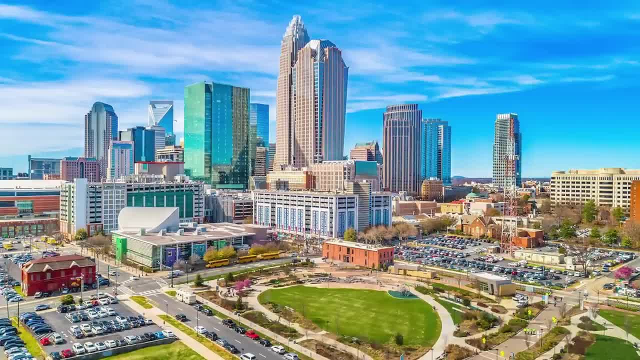 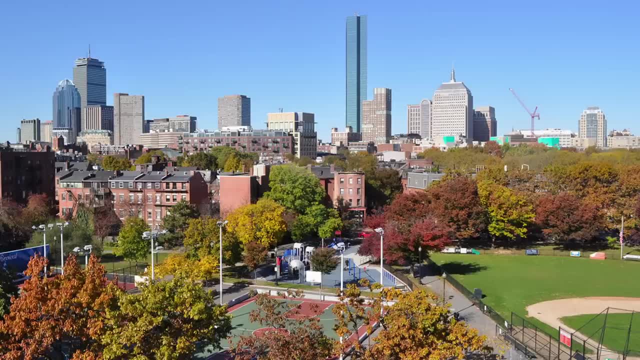 All these Piedmont cities are considered part of a growing mega-region which could one day look similar to the Northeast Megalopolis, the string of near-continuous urbanization that stretches from Washington DC to Boston, Due to the fast-growing population of the South. people believe that these North Carolina cities, alongside cities like Atlanta, Birmingham and the South Carolina cities of Greenville and Spartanburg, could one day comprise a similar urban corridor. Finally, we make it to North Carolina's coastal plain. Many of the states I've covered so far have had large populations on the coast. which tends to have flat land and provides easy access to trade, transportation and fishing. On top of that, most of the British colonies in North America were founded as colonial ports, giving coastal cities the advantage of time. North Carolina, however, only has one prominent coastal city, Wilmington. which, with 220,000 people in its urban area, is the eighth largest in the state and much of the coastal plain in general, is just more sparsely populated. This is for two main reasons, both tied to the region's geography. 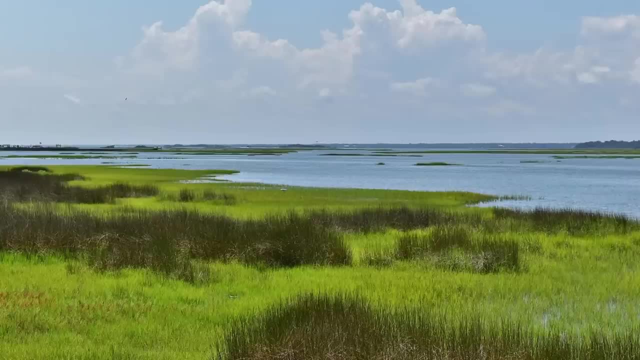 First, as I mentioned before, the land itself contains a lot of swamps and wetlands, especially the closer it gets to the ocean. This makes many areas difficult to settle, and much of the land is a mix of swamps, forests and farms. dotted with small towns and a few larger ones like Wilmington, New Bern, Moorhead City, Greenville and Roanoke Rapids. Altogether, the region is home to 2.388 million people, around 23% of the state's population. 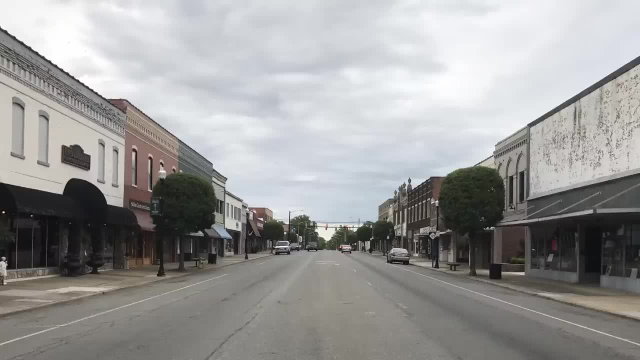 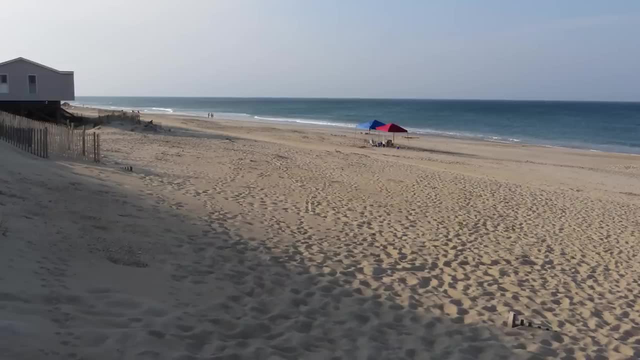 despite being a similar size to the Piedmont, The coast, as is much of the Atlantic all the way from Long Island to Florida, is dominated by a string of sandy barrier islands and peninsulas. In North Carolina, though, these barrier islands are more prominent than in any other state. 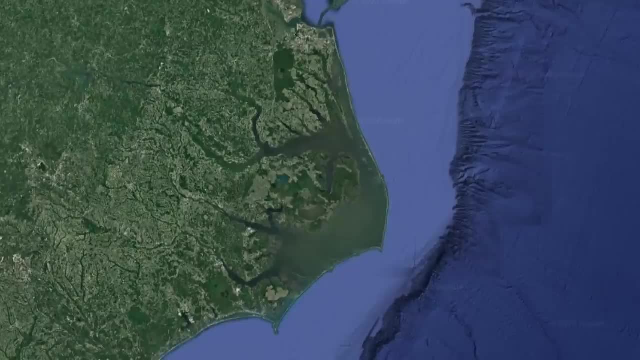 They shape the shoreline into three curving bites, separated by sandy capes that jut out into the sea. In the northern half of the coast, two enormous bays cut inward, some of the largest in the country: the Pamlico and Albemarle Sounds. 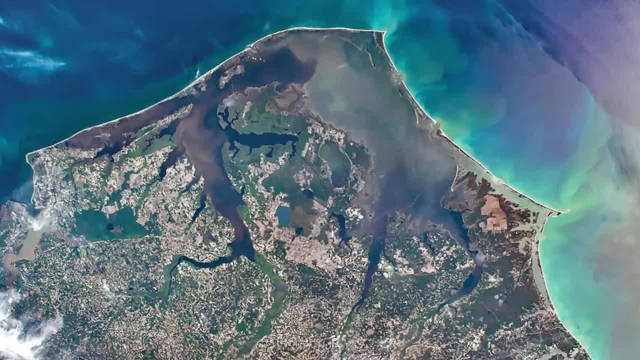 connected by a strait that the famed Roanoke Island sits in the middle of. The barrier islands continue around the Pamlico and Albemarle Sounds, separating them from the mainland by at times as much as 30 miles In the northern half of the coast, the Pamlico and Albemarle Sounds. 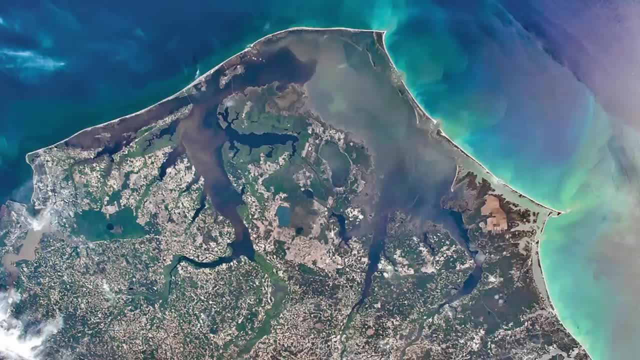 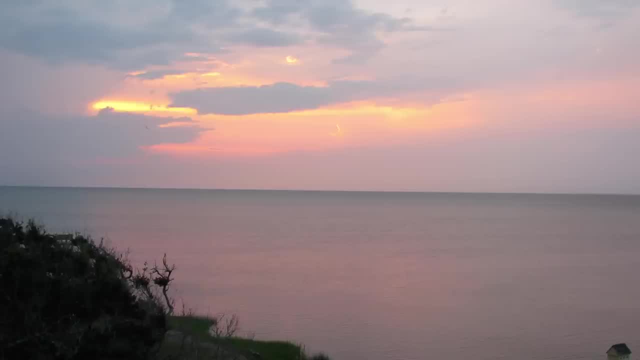 are more popular for banks. save for the area in the north around Kitty Hawk, they're pretty sparsely populated, although, just like the Appalachians, they get millions of tourists every year. Bays and sounds tend to be huge population centers. 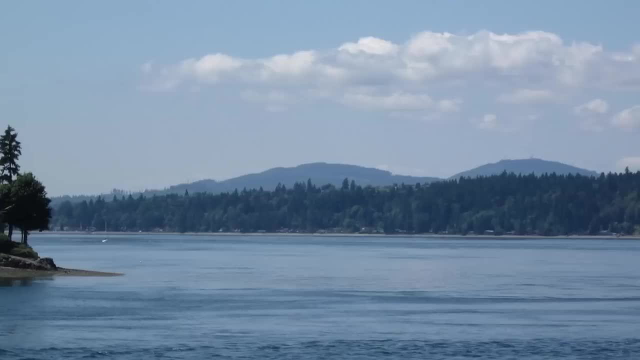 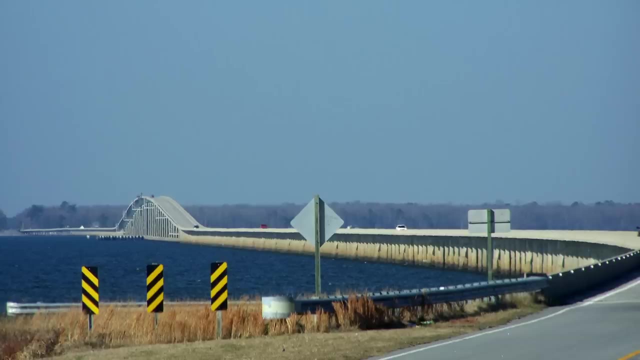 providing calm waters that shelter ports and make it easier for cities to develop. The San Francisco Bay, San Diego Bay, Puget Sound, Chesapeake Bay, New York Bay and Massachusetts Bay, just to name a few, all saw huge cities develop around them. 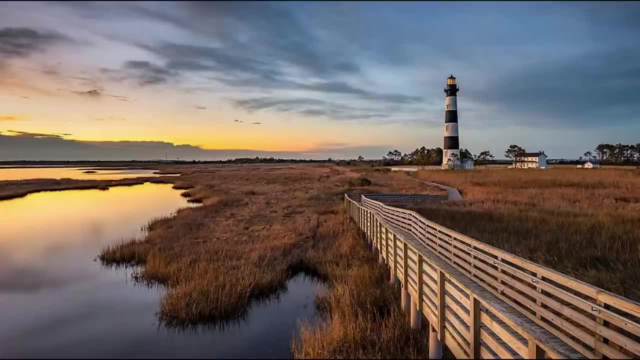 The San Francisco Bay is too shallow for ships to navigate and the outer banks sand dunes, which are always shifting, moving and splitting apart, make it difficult to enter. On top of that, the North Carolina coast is very dangerous for boats. 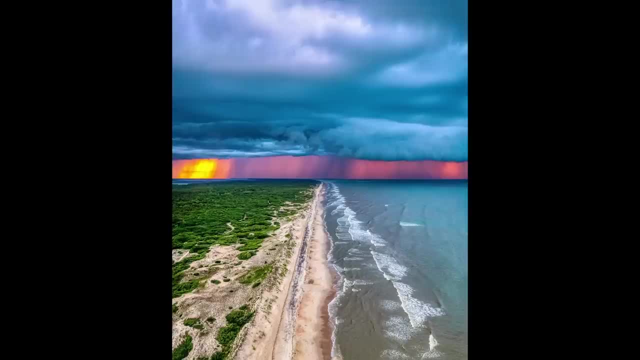 Each of the capes has dangerous shallow shoals that continue for miles and miles. further underwater, Flat, low-lying and jutting out far from the mainland, the outer banks have been the cause of a shocking 5,000 shipwrecks. 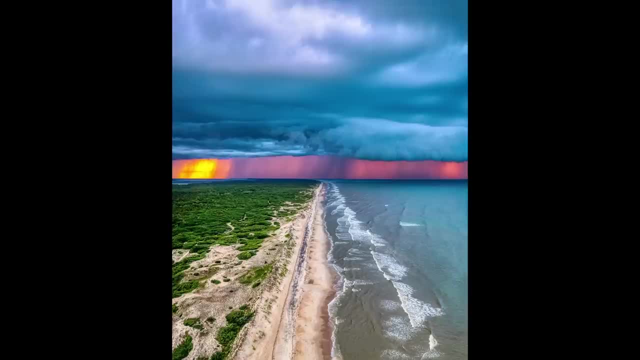 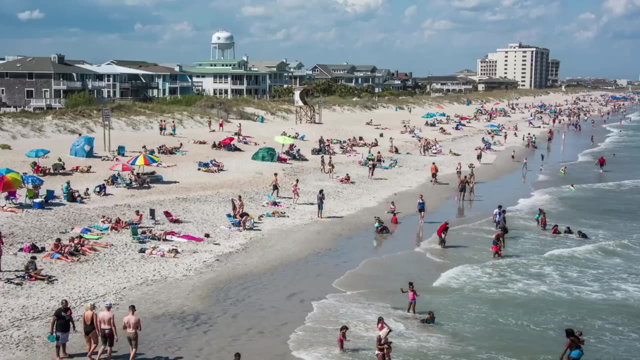 and it's been given the nickname the Graveyard of the Atlantic. Some of the place names along the outer banks- Cape Lookout, Cape Fear and others- show exactly what sailors thought of the North Carolina coast. Even Blackbeard couldn't survive the outer banks. His ship, the Queen Anne's Revenge, sank there in 1718, and he was captured and killed on one of the islands not long after. The outer banks are home to a unique accent and dialect of English, often referred to as hoitoider. 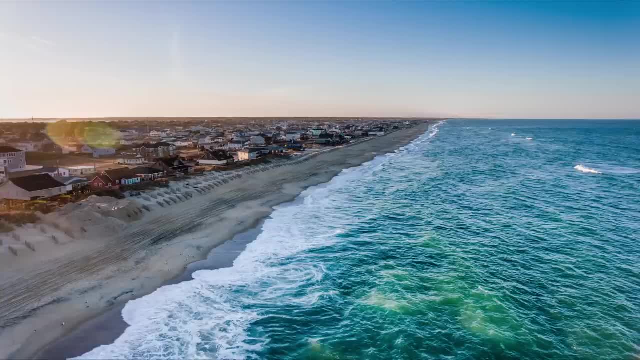 that's found on the islands, as well as in a number of marshy, isolated islands in the Chesapeake Bay. Due to the isolation of the islands, it develops completely separately from American English and has an accent that sounds more similar to what you'd expect to hear in Britain or Ireland than the United States. 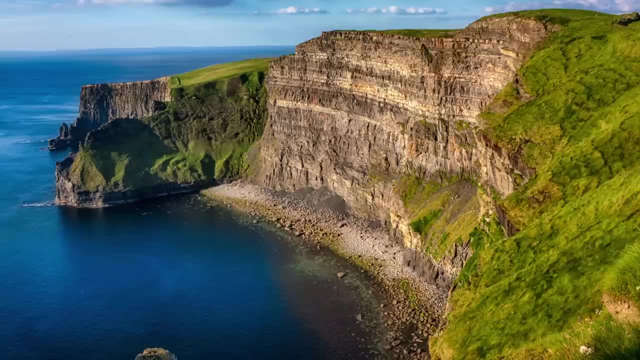 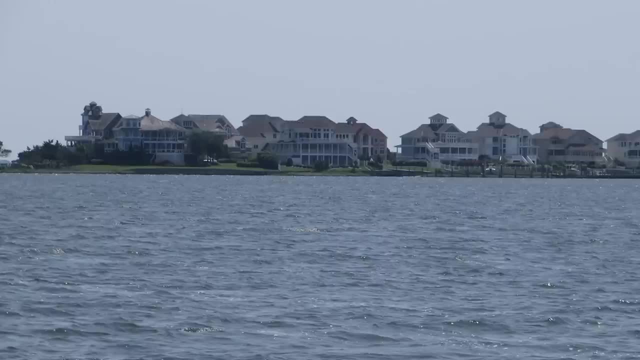 There's plenty of videos in this unique dialect and I'd definitely recommend you watch some, because it is very interesting. Roanoke Island was the site of the famous Roanoke Colony, the first British colony, and would become the United States that then seemingly disappeared without a trace. 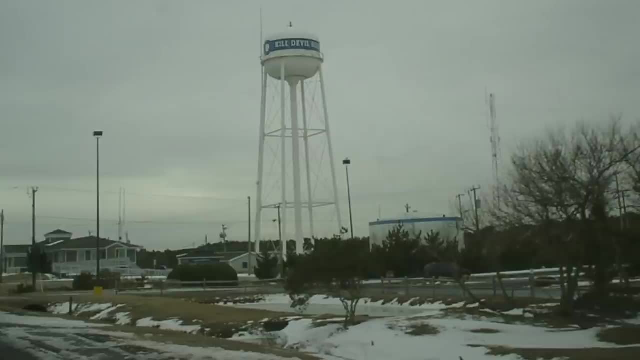 and Kill. Devil Hills, near Kitty Hawk, is where the Wright brothers flew the first ever airplane. North Carolina was originally home to many different indigenous peoples. In the coastal plain along the Pamlico and Albemarle sounds lived dozens of tribes who spoke Algonquian languages. 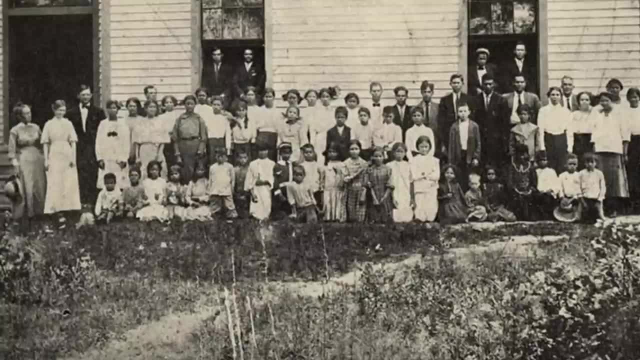 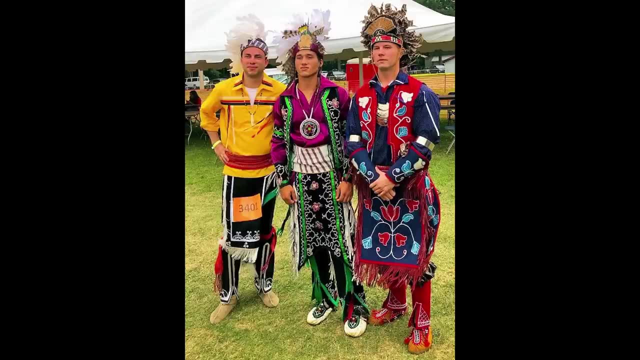 such as the Roanoke, Croatan and Pamlico. Much of what is now the central east part of the state, from the border with Virginia to South Carolina, lived the Tuscarora. In the Piedmont a number of peoples, including the Cheraw, Catawba and Yeson, lived. 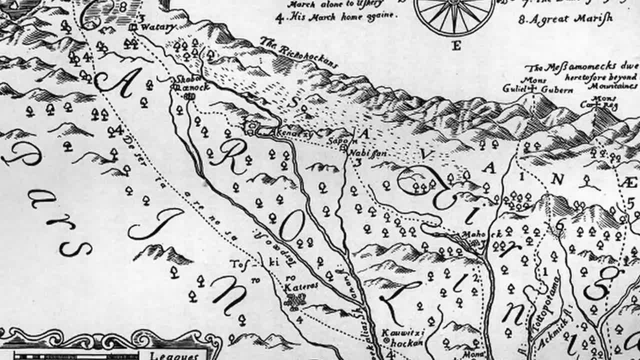 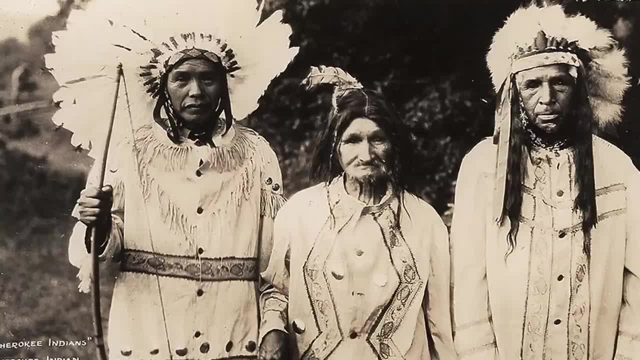 In the Appalachians, the Miccosukee lived in the south, the Monotone in the north and the Uchi and Cherokee throughout the entire region. With the arrival of European colonists in the Americas they brought with them diseases that 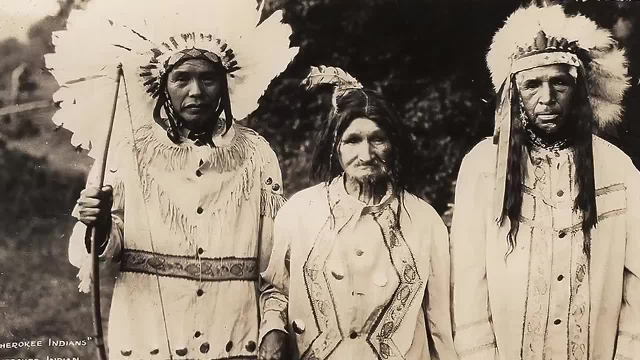 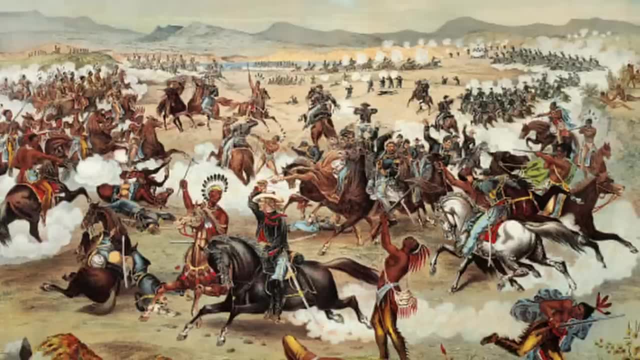 the indigenous peoples had not yet been exposed to, such as smallpox. These diseases ended up decimating the continent's indigenous peoples, killing 90% of them. Those that survived often died at the hands of the colonists as European settlements pushed further westward. encroaching on their land and pushing those that survived west. Though Jamestown was Britain's first successful colony in what would become the United States, the first colony they established was in what would become North Carolina In 1585, 22 years before the founding of Jamestown. 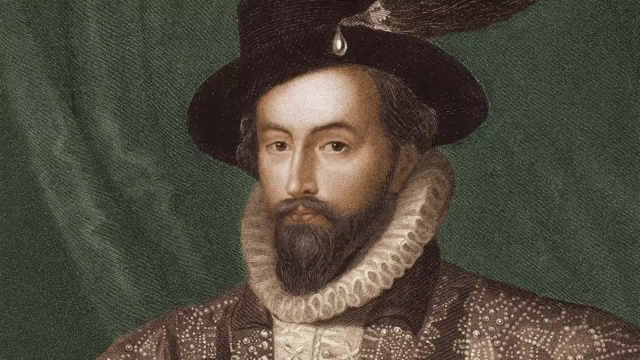 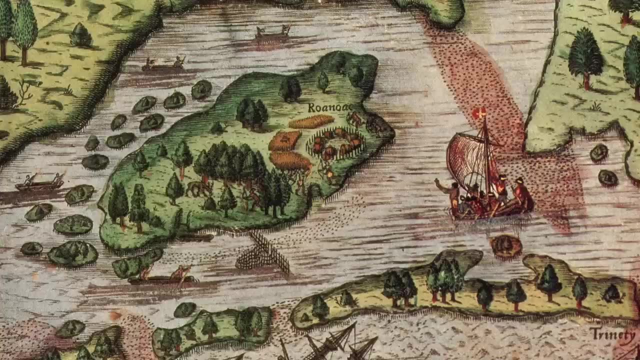 a wealthy Englishman named Sir Walter Raleigh funded the creation of what he hoped would be England's first permanent colony in the New World. It was called the Roanoke Colony, located on Roanoke Island, which sits between the Albemarle and Pamlico Sounds. 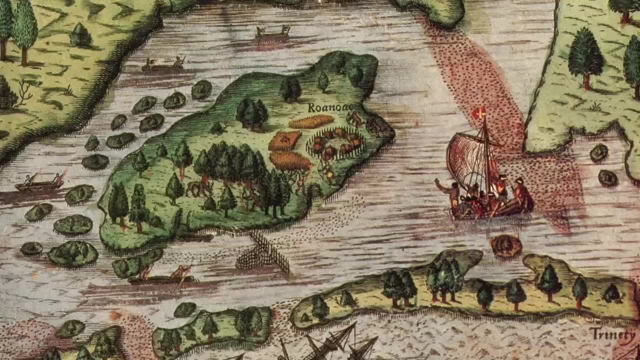 and between mainland North Carolina and the Outer Banks. Raleigh's first attempt failed, but his second try at establishing a settlement seemed promising. Raleigh never went to Roanoke himself. Instead, he picked an artist named John White to set up the colony and serve as its governor. 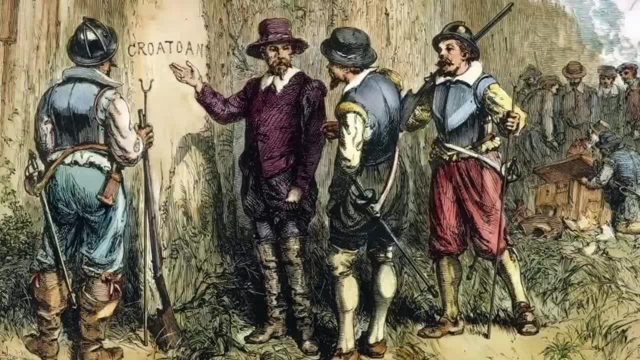 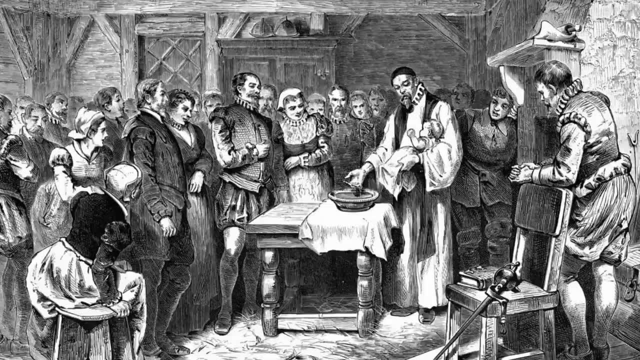 White brought with him 115 other people, including his own family. His granddaughter, Virginia Dare, was born there and became the first English child born in the New World. However, the colony was low on resources and thinking of relocating, and soon after White went back to England to resupply and get assistance. 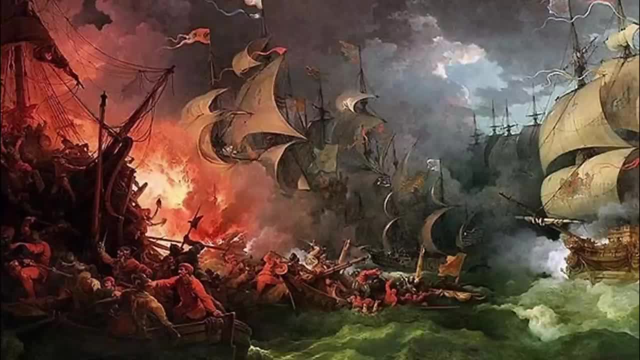 The timing, however, could not have been worse. England was at war with Spain and every ship was ordered to remain in England to help with the war effort. By the time White finally returned, three years had gone by. When he got back to Roanoke he spotted smoke from the island. 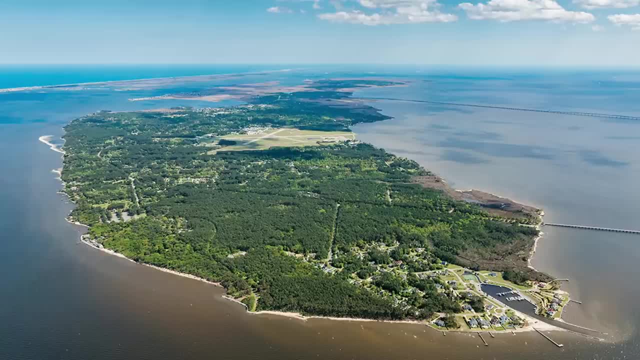 but arrived to find that the colony and all its inhabitants had vanished. Most of the buildings had been completely dismantled and taken away, and the only clues to what had happened were two carvings, the letters CRO in a tree and the word Croatoan in a fence. 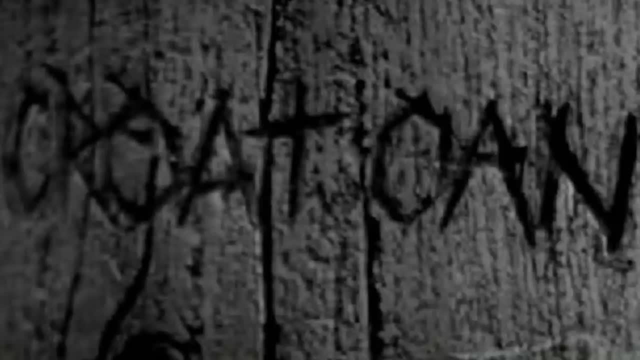 This has led to one of the most prominent unsolved mysteries in American history, and Roanoke is often known as the Lost Colony. People will often just end the story there with the carvings, making Croatoan out to be some mystery word, but it's not. 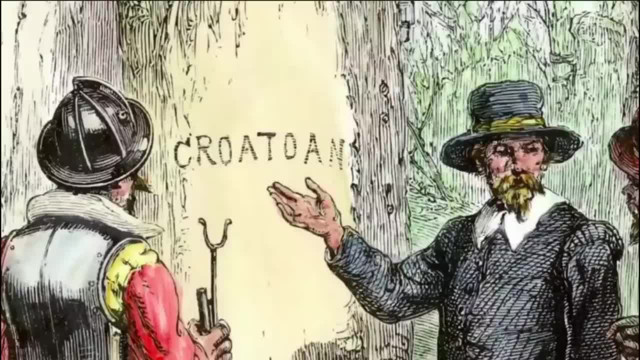 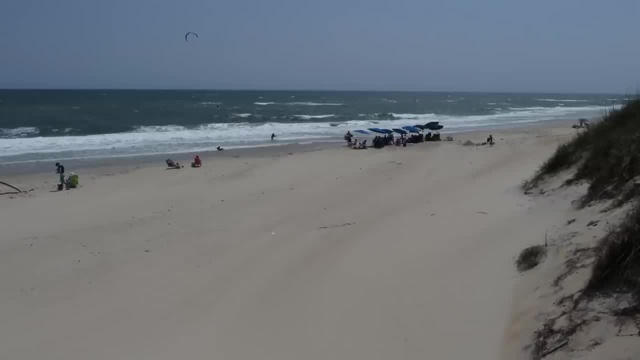 It could have referred to either two or three things: The Croatan native people who lived in the area and who the Roanoke colonists had a good relationship with, or Croatoan Island, now known as Hatteras Island, an island in the Outer Banks that was often the landing point. 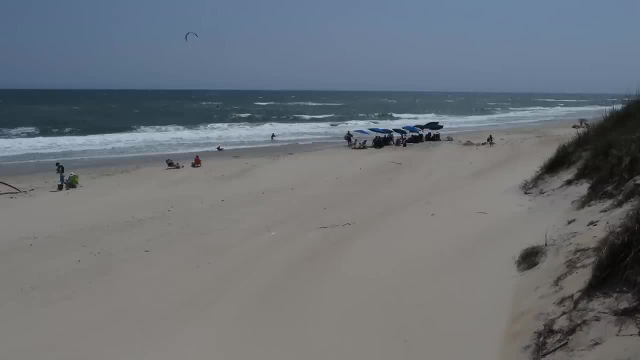 for the colonists to get to Roanoke. While it's unclear what happened to the colonies, the subject of countless theories and speculation, I think the most compelling theory is that they relocated somewhere else, If the message referred to an attack by the Croatan. 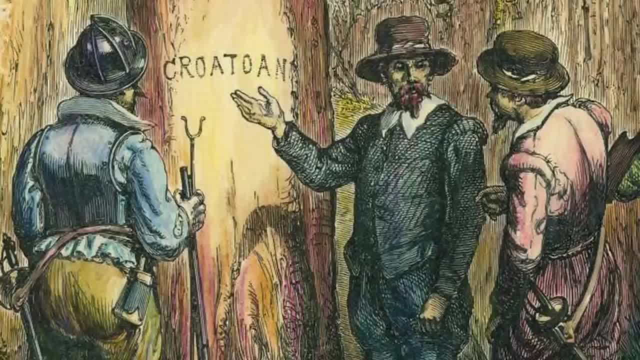 which I think is unlikely because they had a good relationship. there would have been signs of a conflict and the colony would have been hastily abandoned, Not completely disassembled, and moved. Also, the colony was down to its last straw and was thinking about moving anyway. 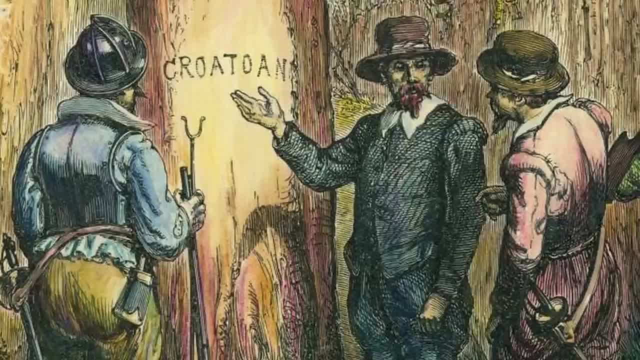 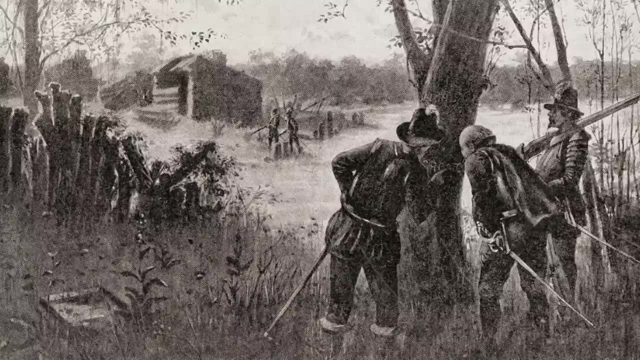 That's why White left in the first place. In fact, their situation was so serious that they had agreed before he left that if they moved they would leave behind a message, so he'd know where they went. Though the word carved in the tree might seem mysterious to us, 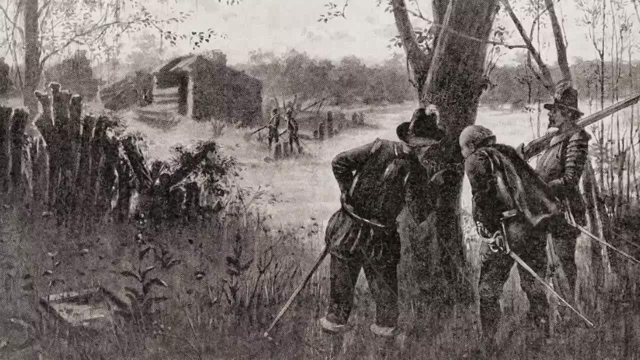 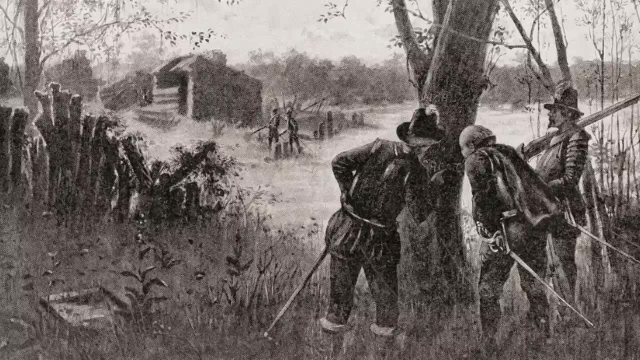 it probably wouldn't have been to White, signifying that the colonists had either gone to Croatoan Island or had been taken in by the Croatan. In fact, both are a possibility. The island was within the territory of the Croatan. 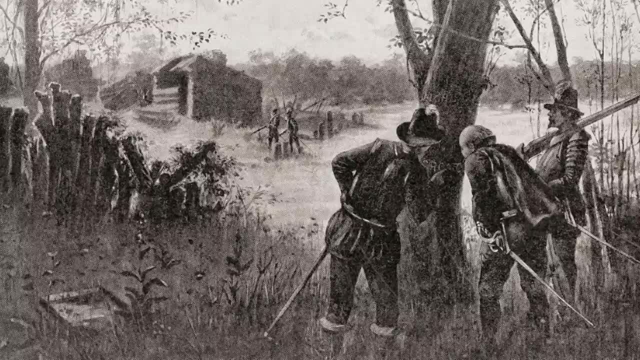 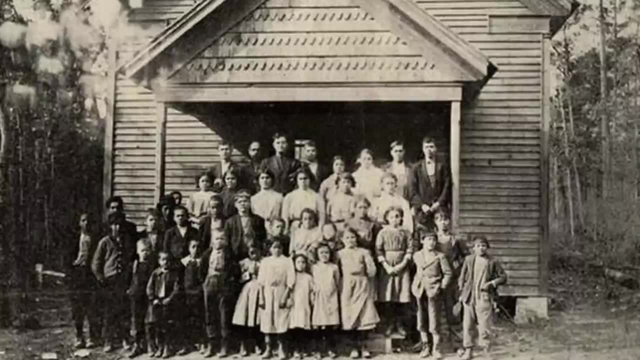 Possibly. they'd tried to resettle there for a time and, with no sign that White was coming back and lacking enough resources to survive on their own, they abandoned the idea of a colony and moved in, with the Croatan adopting and assimilating into their way of life. 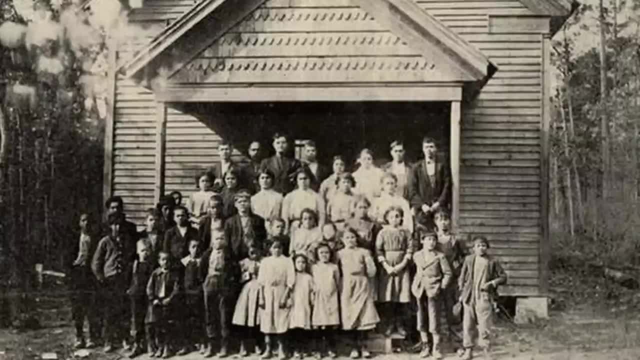 White tried to go to Croatoan Island and find them, but bad weather forced him back to England, where he always held out hope for his family's survival. What exactly became of the colony still remains a mystery, and though claims that it has been solved will inevitably pop up on the news every once in a while. 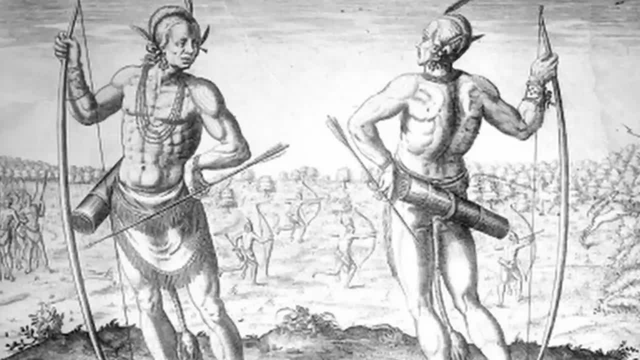 exact evidence of the colony's fate has never been discovered. However, the idea that they assimilated with the Croatan is one of the most popular theories and personally I find it the most plausible. It would have made the most sense for the colonists. 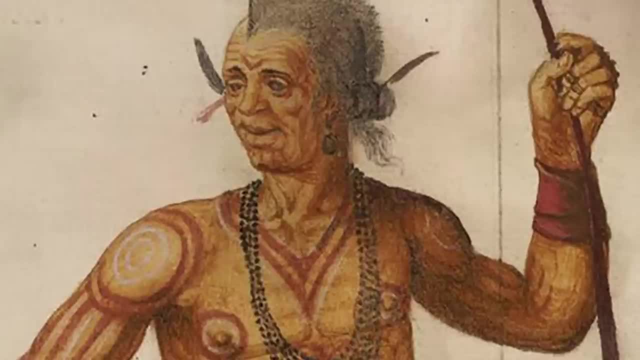 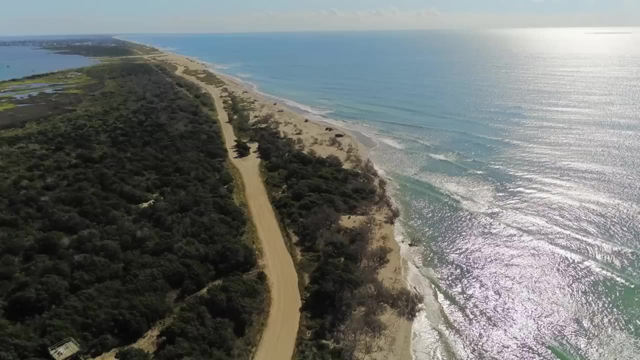 They were good friends with Manteo, a prominent Croatan who had built a strong relationship between the colony and the tribe. Jamestown colonists in fact reported meeting a tribe on Hatteras Island who had some European features and claimed European ancestry. 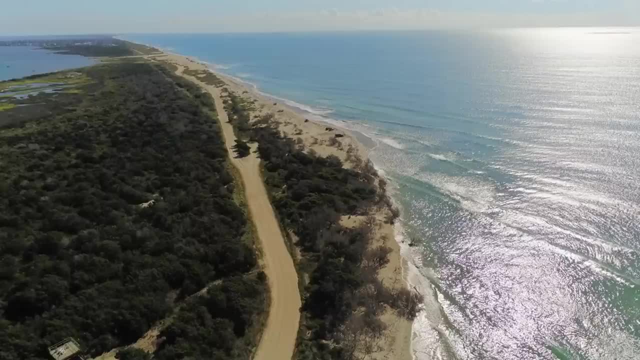 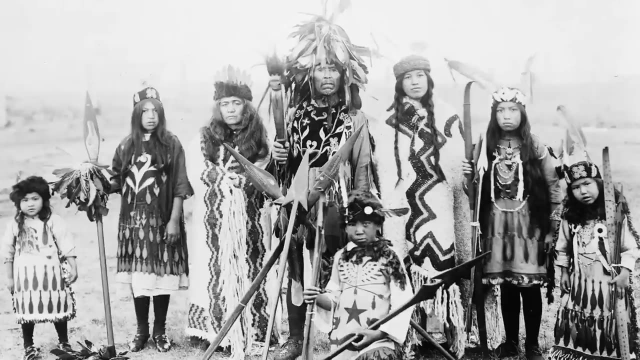 Remember, Hatteras Island was the same Croatoan island that White thought they had moved to. There's even a theory that the modern Lumbee people are descended in part from the Roanoke colonists. The Lumbee are a tribe that formed 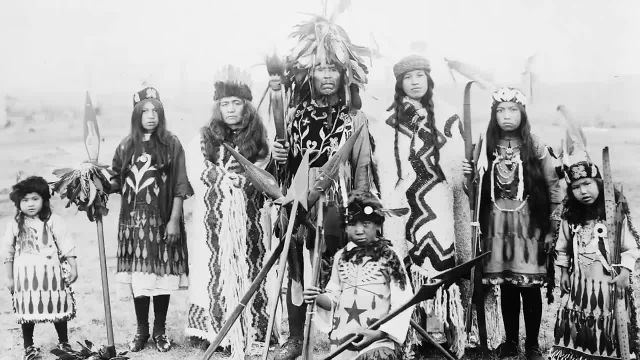 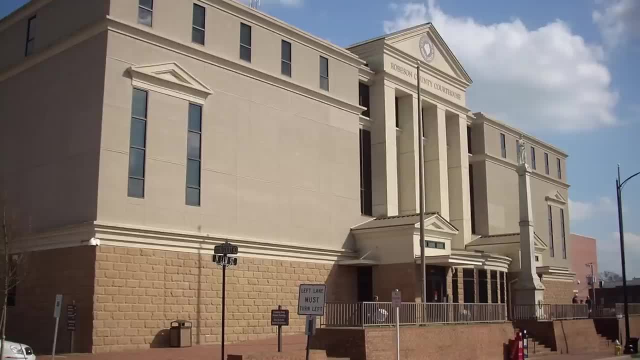 from many indigenous peoples from a number of different tribes. Decimated by disease and conflict, their societies torn apart, they fled to Robeson County, a swampy part of the state that European settlers had, for the most part, been uninterested in. They became known as the Lumbee and, though unrecognized at the federal level, 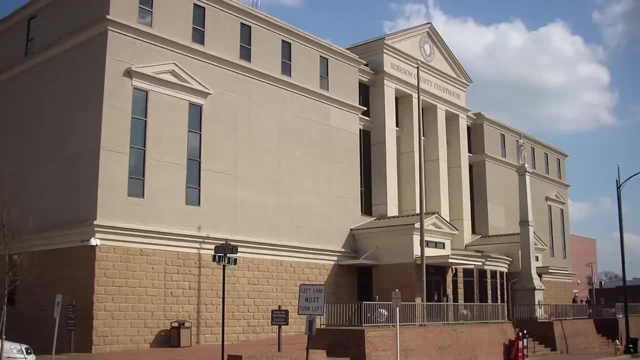 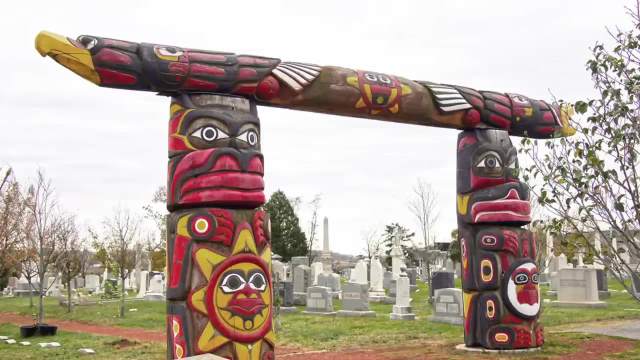 they're the largest Native American tribe in North Carolina, the East Coast and west of the Mississippi altogether, with 60,000 Lumbee living in and around Robeson County and helping give North Carolina the largest Native American population in the eastern half of the country. 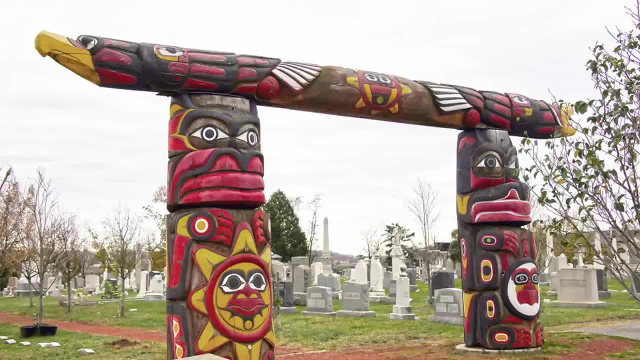 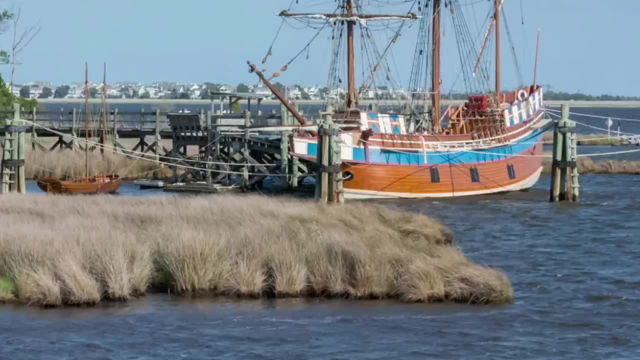 They have a unique society and culture that's been shaped by a number of different influences from many different Native tribes, as well as likely Black and White ancestors as well. After the failure of Roanoke, European settlement in the region didn't occur for around another 70 years. 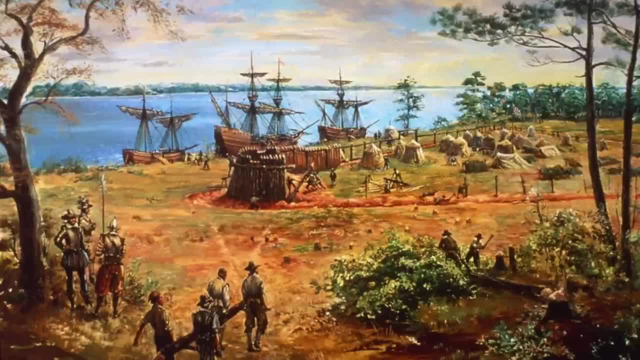 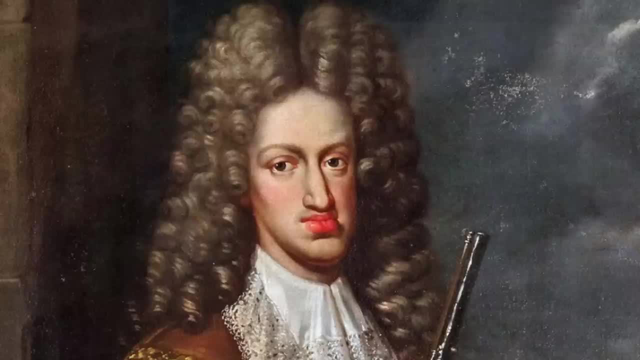 The colony of Virginia to the north had become quite successful and some settlers began moving south, outside the colony, to what is now North Carolina, along Albemarle Sound. In 1663, British King Charles II regained power following the English Civil War. 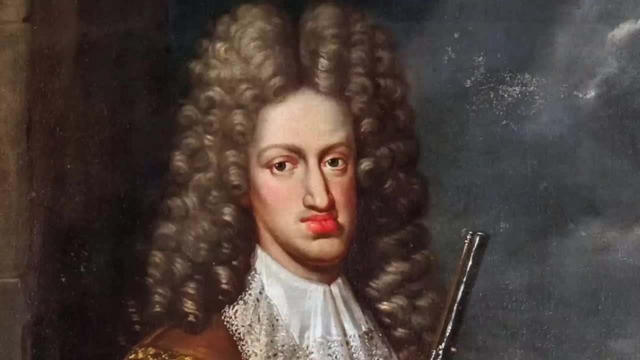 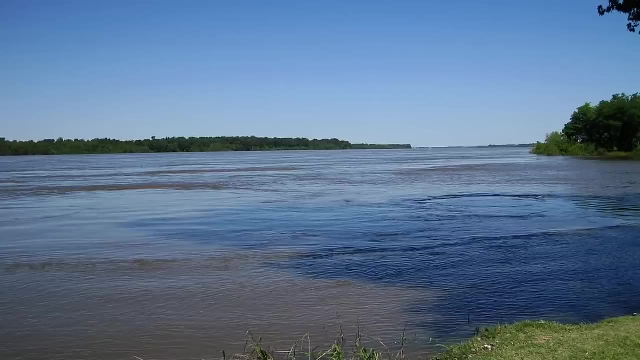 and he granted a large swath of the south he called Carolina to eight noblemen who had helped him take back the throne. It was huge, stretching from the Mississippi River in what is now Tennessee and Mississippi, all the way to the Atlantic, from Virginia to Florida, which was controlled by Spain. It was meant to be almost a buffer zone to prevent Spain from coming close to the far more populous British colonies to the north. Carolina was a huge colony. In the north most people lived just south of Virginia on Albemarle Sound, while in the south- the capital of Charlestown, later Charleston. 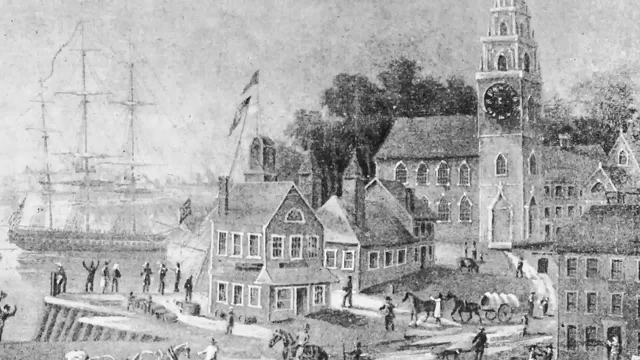 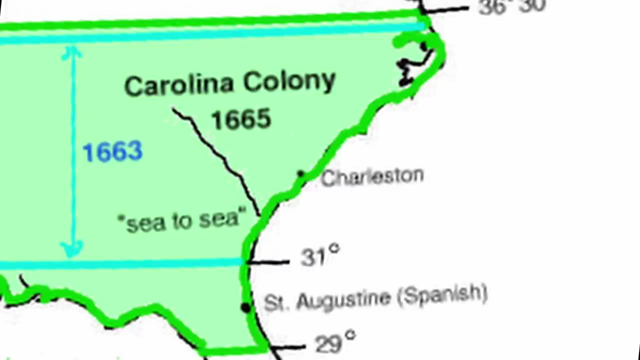 was the center of population, an increasingly prosperous port city. These population centers were separated by almost 300 miles of wilderness and as such it was difficult for the colonial government in Charlestown to govern the northern part of the colony effectively, Eventually to make governing easier the remaining one colony. 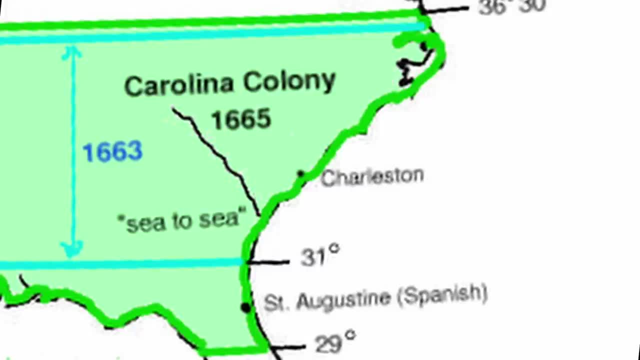 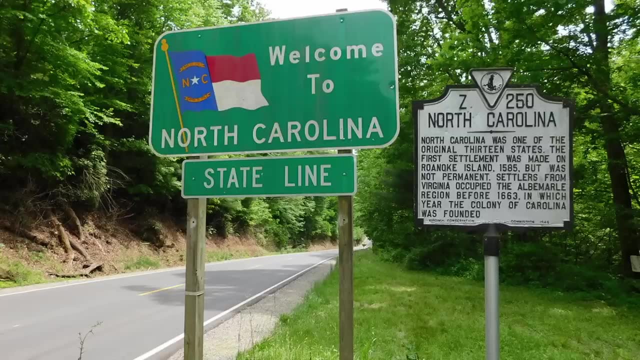 the northern and southern parts were split into two self-governing provinces, Albemarle and Clarendon, People eventually began referring to Albemarle as North Carolina and Clarendon as South Carolina In 1712, unable to maintain a single government over such a large distance. 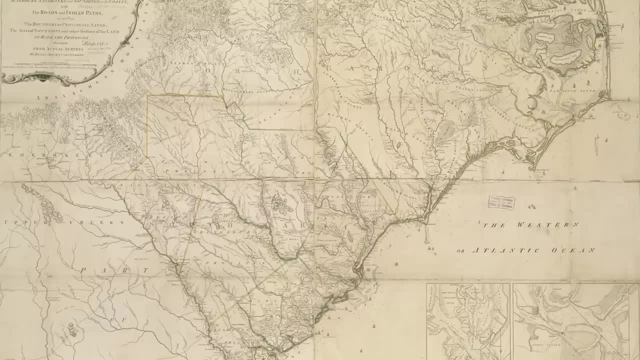 and significant social and economic differences. North and South Carolina split into two separate colonies with separate governments. Indentured servants made up much of the population, some immigrants from England and others forcibly brought over from Africa. Eventually, a system of race-based slavery solidified in the colonies. 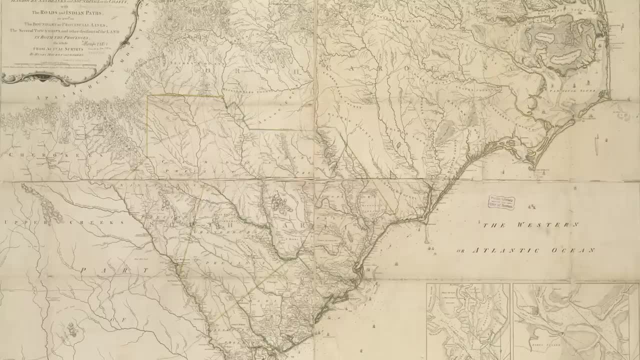 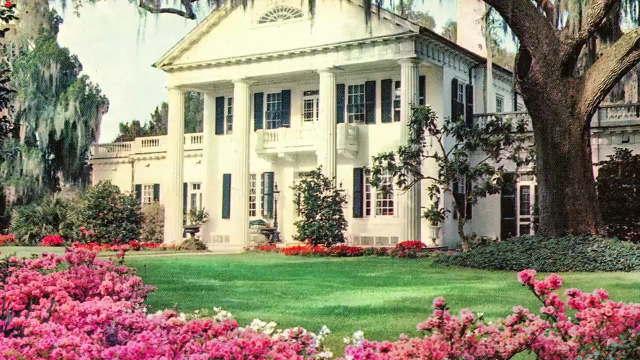 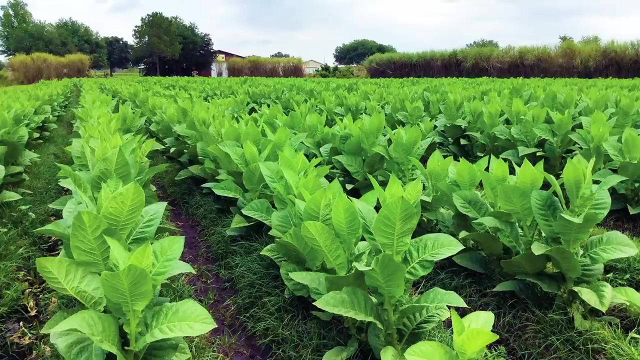 and tens of millions of people forced into slavery were brought into the 13 colonies and later the United States, but primarily the agricultural south from Africa. They were forced to work on plantations, often growing cotton and tobacco, throughout North Carolina, and the colony quickly became the center of tobacco production in the 13 colonies. 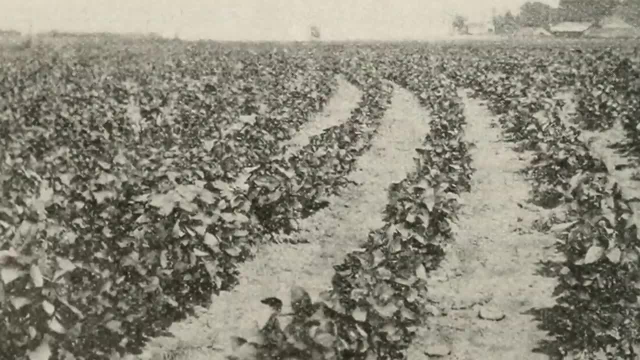 Its population remained very small Due to its agricultural nature. no major cities began developing for quite some time and it remained, despite its large area, a very sparsely populated colony. However, in the decades leading up to the Revolutionary War, its population skyrocketed. 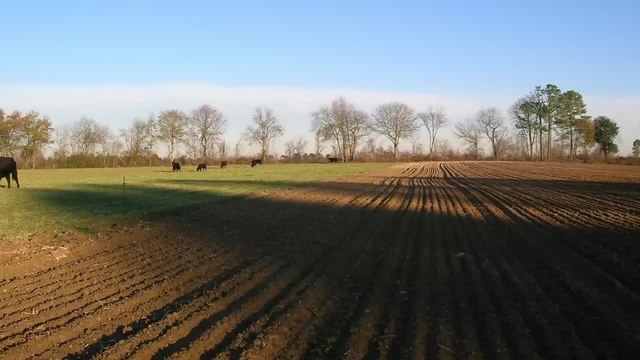 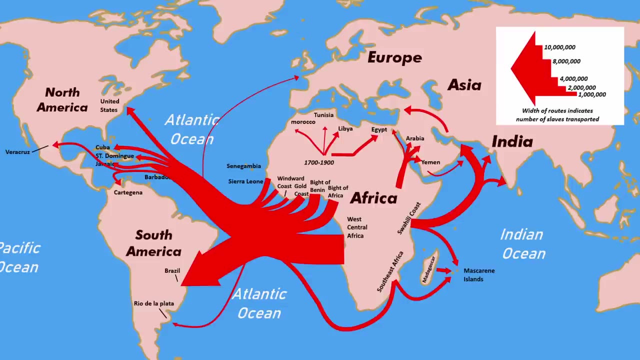 People began moving to the emptier and agriculturally successful colony from the more populous colonies to the north. Hundreds of thousands of enslaved people were brought in from Africa and immigrants began flocking there from Europe. English people continued settling the colony, but so did a large number of Germans. 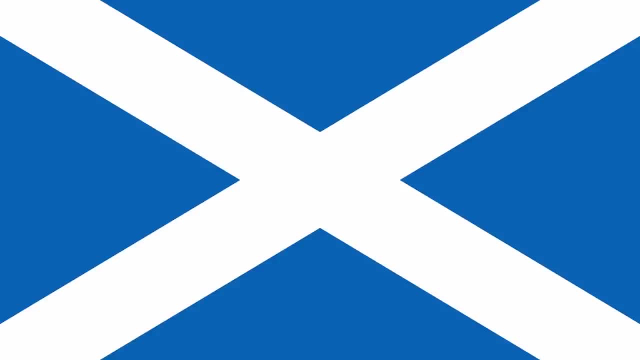 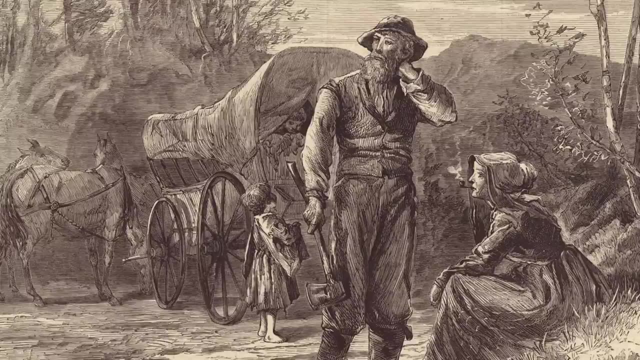 many of whom were members of a religious group called the Moravians and Scottish people, as well as Scots-Irish, an ethnic group from Northern Ireland whose ancestors had moved there from southern Scotland and northern England as part of the British colonization of Ireland. 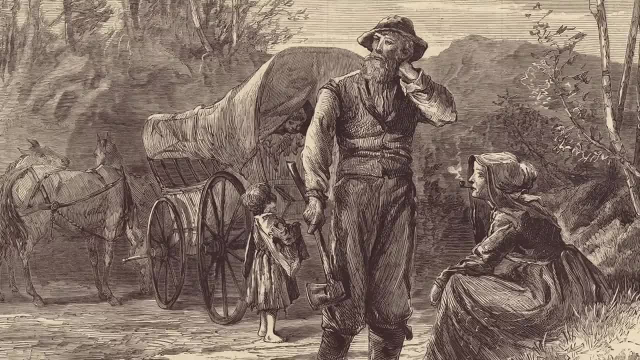 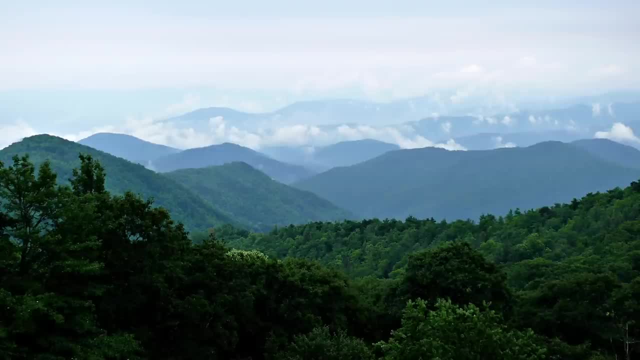 Poorer immigrants, mainly Germans, Scots-Irish and lowland Scots, went to the Piedmont and Athens colonies, where it was more hilly and mountainous and agriculture was more difficult, whereas wealthier immigrants such as Highland Scots settled the agriculturally rich coastal plain. 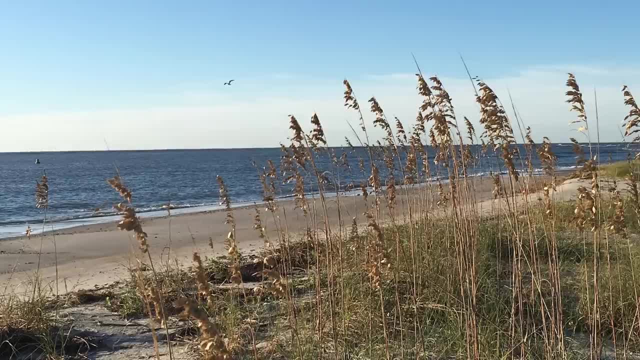 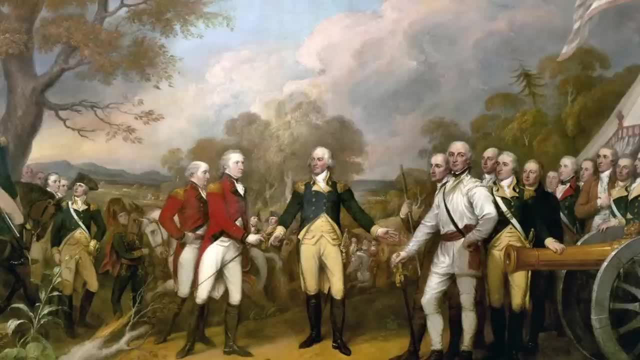 Because of all this, by 1790, North Carolina was surpassed in population by only two other states. Significant fighting took place during the Revolutionary War in North Carolina. Many poorer North Carolinians in the west wanted independence, whereas wealthier ones in the east wanted to remain with Britain. 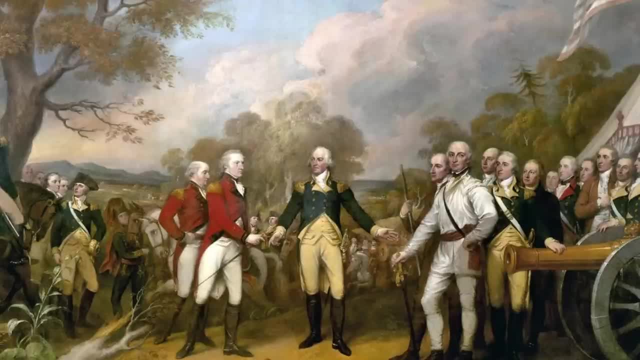 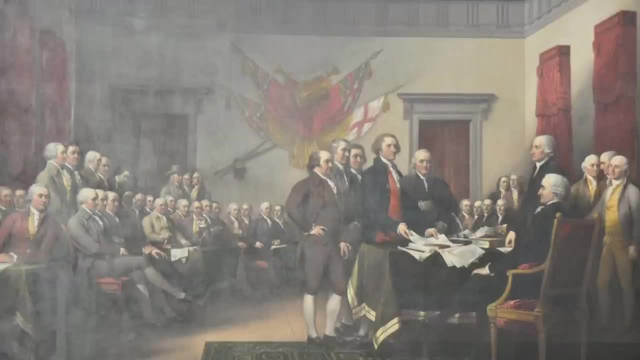 As war waged on, supporters of the Revolution and supporters of the monarchy formed militia groups waging war against one another throughout the state. On November 21st 1789, North Carolina ratified the Constitution joining the United States and became the 12th state to do so. the second to last of the former 13 colonies. Before the war, North Carolina had stretched all the way across the Appalachian to the Mississippi River. The settlers of this vast western half of the colony often wanted nothing to do with North Carolina, and parts of it had tried to split off several times. 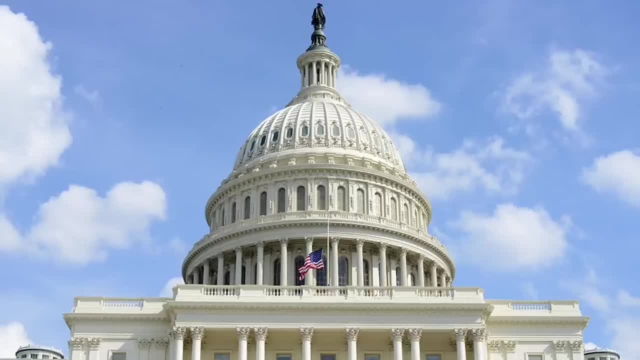 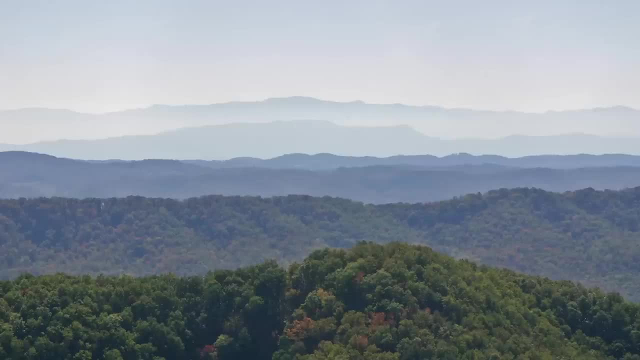 After the war and independence, North Carolina owed the new federal government money and gave up this western half of the state in 1790 to pay it off. It became a territory called the Southwest Territory and later became the state of Tennessee. The Cherokee inhabited a territory stretching from Kentucky to Georgia and Alabama. As they watched other native tribes disappear from existence due to war, disease and genocide at the hands of the colonists, the Cherokee, along with four other prominent tribes in the south, decided to adopt the lifestyle and customs of the European settlers, in the hopes that they would not meet the same fate. 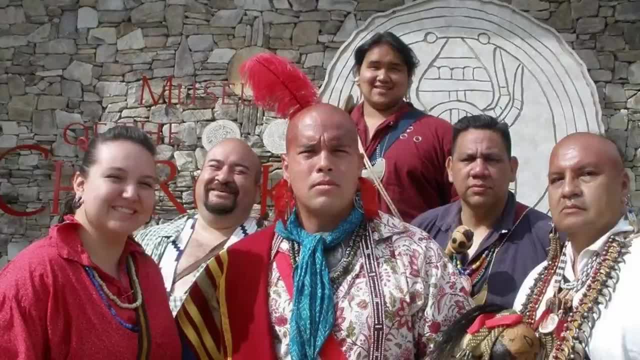 as so many other native peoples, They created a written form of their language, formed a centralized government with a capital, adopted similar styles of architecture as well as European systems of land ownership, and many converted to Christianity and learned English. Some even adopted the horrible practice of slavery. 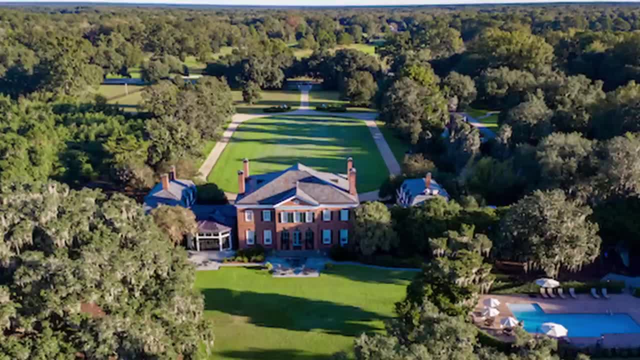 and many black people were forced into slavery by the Cherokee For a while. adopting the lifestyle of the colonists and later the early Americans was successful and they maintained a good relationship with the US. This changed under the presidency of Andrew Jackson. 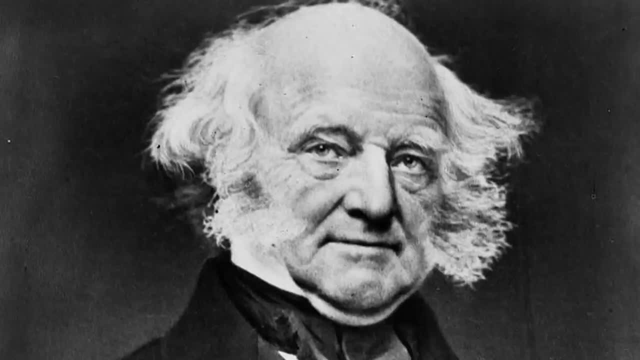 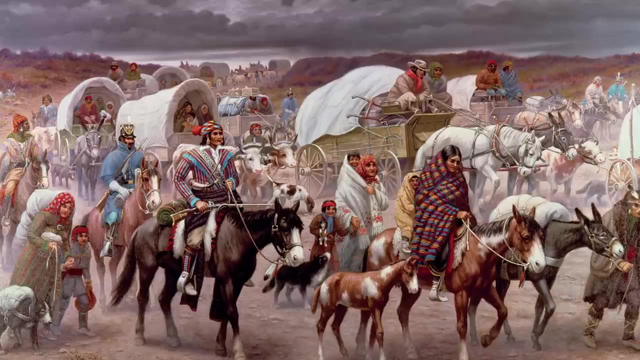 and his successor, Martin Van Buren. As the populations of the south continued growing, they wanted more land, opened up for American settlement and the expansion of slave plantations. Despite the Supreme Court ruling it unconstitutional, they implemented a policy called the Indian Removal Act. 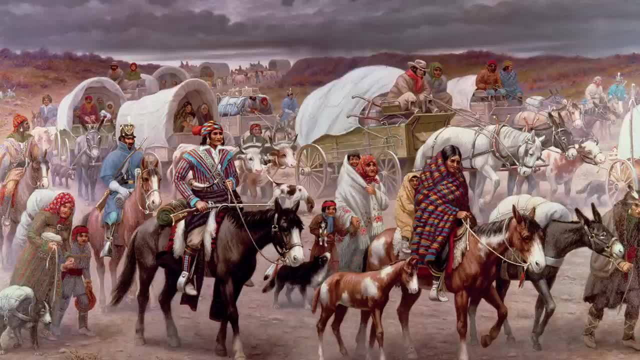 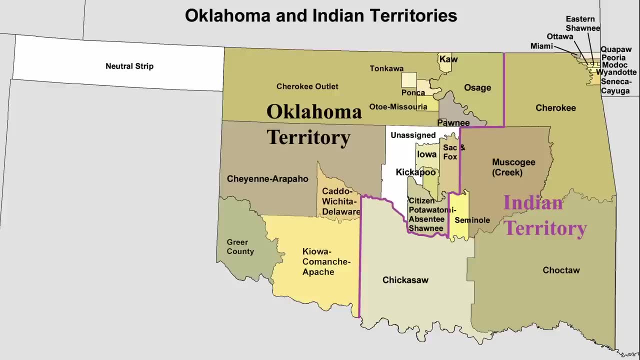 which saw the forced march of the Cherokee, as well as the four other southern tribes who'd adopted an American lifestyle, and the black people that enslaved from the southeast hundreds of miles west to what was then set aside as the Indian Territory now called Oklahoma. 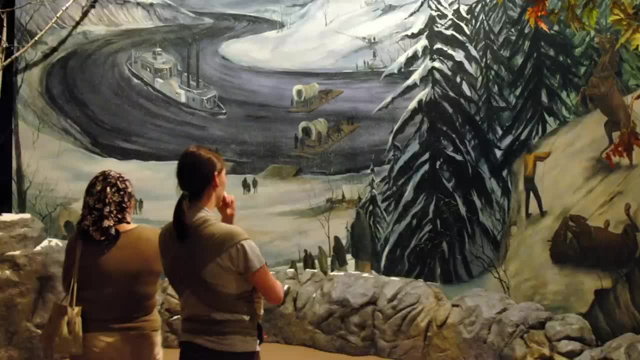 Known as the Trail of Tears. 46,000 people were sent on this forced mass migration. 4,000 Cherokee people alone died on the Trail of Tears, and estimates vary, but thousands more native people died. in total, The Cherokee have today, by far 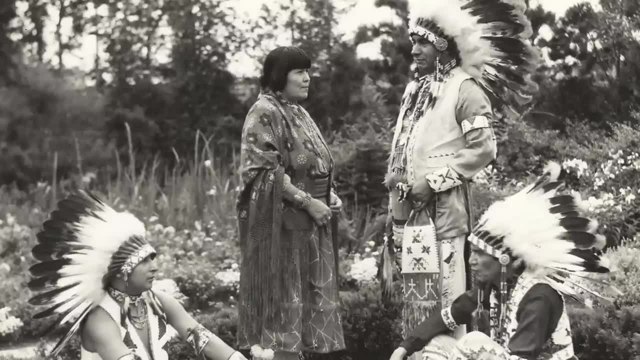 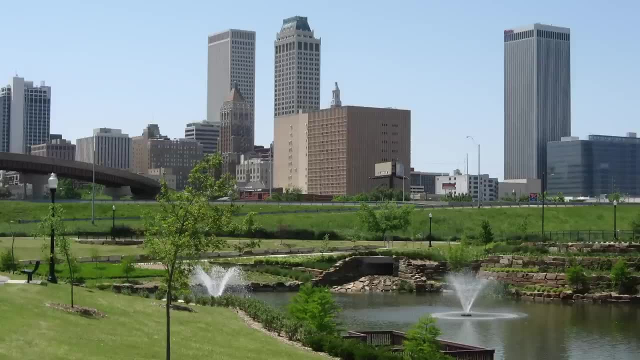 the highest population of any indigenous people in the country, as 819,105 Americans are Cherokee. Today, much of the city of Tulsa, Oklahoma, is part of Cherokee land and 9.2% of Tulsans are native people. 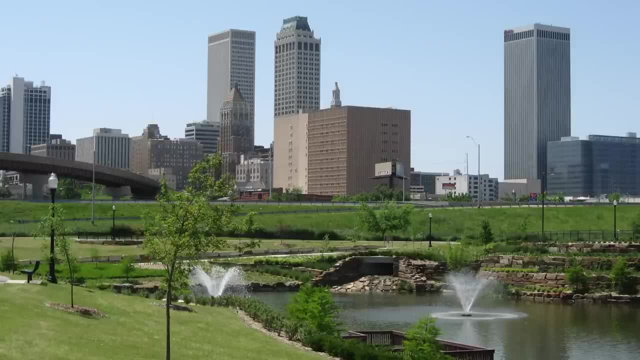 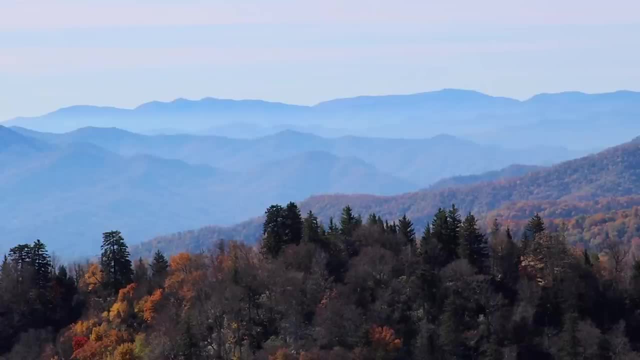 The second highest proportion of any major city in the US after Anchorage, Alaska. A number of Cherokee remained in the south even after the Indian Removal Act, and today they live in the Appalachians in North Carolina, known as the Eastern Band of Cherokee Indians. 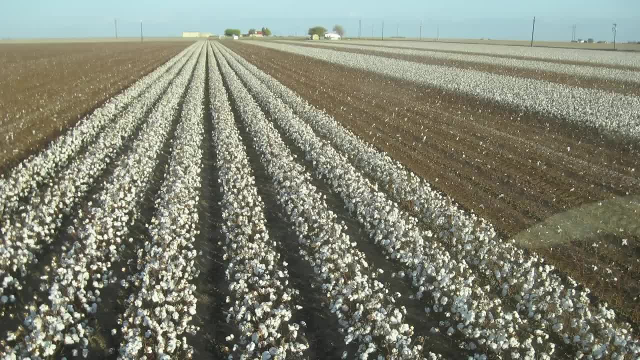 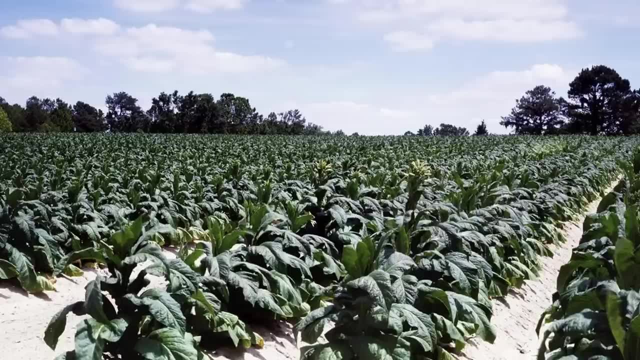 The state remained dominated by agriculture, specifically the cotton and tobacco industries, and the horrible practice of slavery that powered them. In fact, by the time the Civil War broke out, enslaved black people made up a third of North Carolina's population, As tensions grew in the country over slavery. 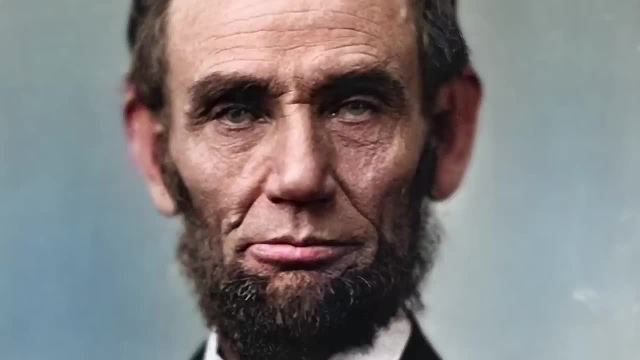 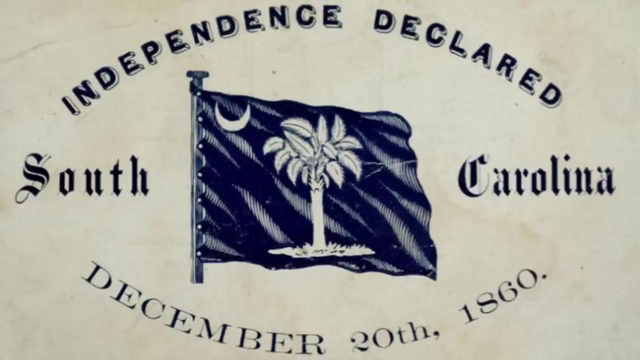 their neighbor to the south was a center of conflict and, following Abraham Lincoln's election as president, South Carolina seceded from the Union on December 20, 1860.. A number of other southern states followed suit, but North Carolina held off. 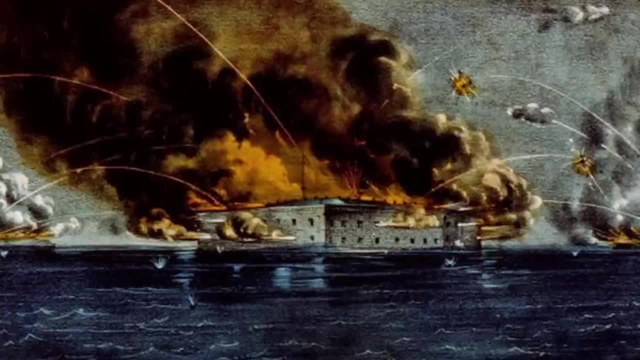 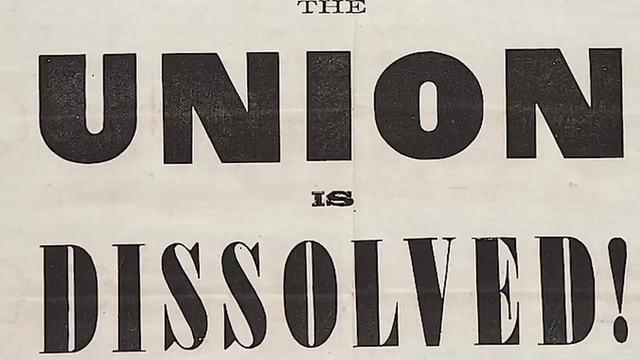 Even when the Civil War broke out at the Battle of Fort Sumter, North Carolina had not yet joined the Confederacy. They were the second to last state to formally secede, doing so on May 20, 1861.. While many North Carolinians supported the Confederacy, 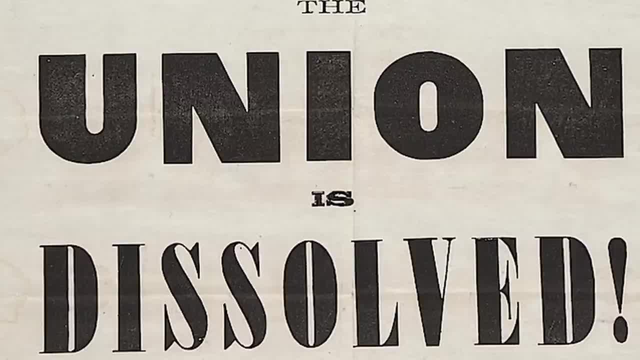 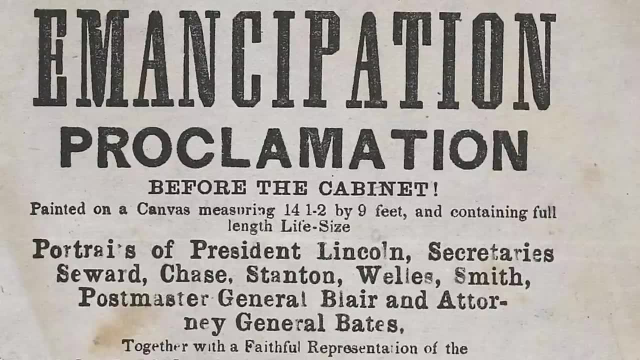 a number supported the Union and no major battles were fought in the state. In 1863, Abraham Lincoln issued the Emancipation Procedure and with the end of the war in 1865, North Carolina's enslaved population was freed. At first things seemed to be going well. 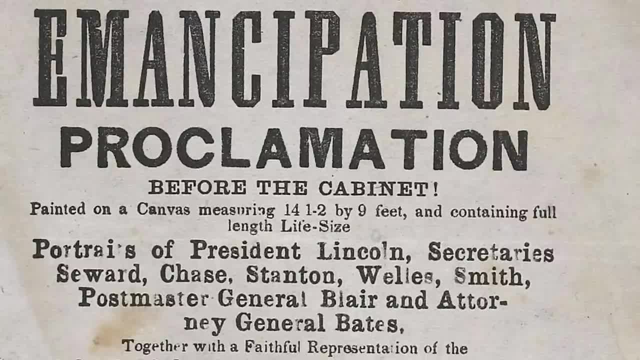 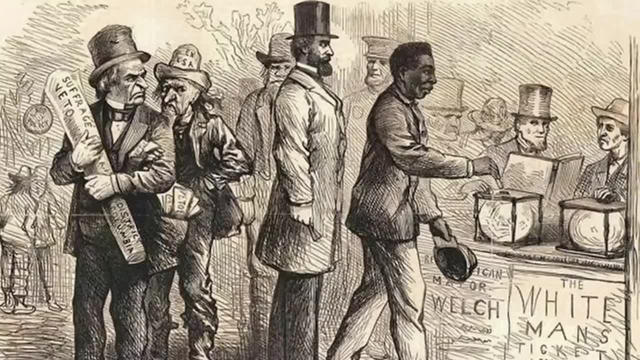 Under Reconstruction, the state elected 19 black people to the state legislature and went on to elect four black representatives to Congress. However, with the withdrawal of Union troops from the south and the end of Reconstruction, racist violence in the state quickly grew worse. 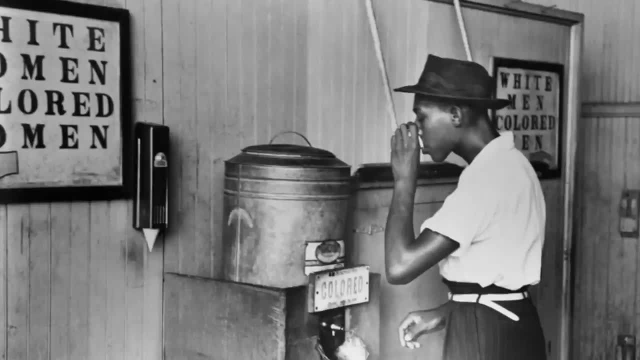 Racist Jim Crow laws were passed that turned racial discrimination and segregation into law and made it near impossible for black people to vote and participate in government. Lynchings were common and many black people had little choice but to work in an exploitive system of farming. 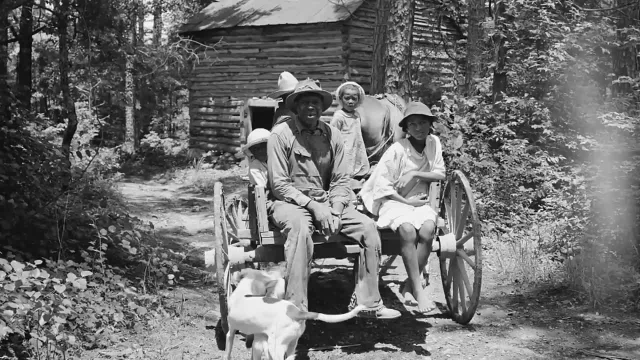 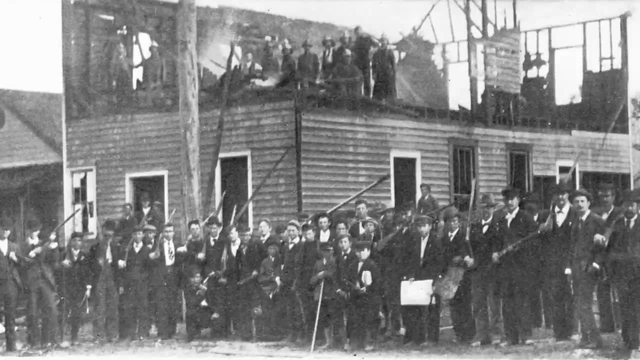 known as sharecropping, essentially slavery by a different name. The epitome of the Jim Crow era in the state was the Wilmington Insurrection of 1898, thought to be the only successful coup d'etat in American history. During the coup, a mob stirred up by a group of white supremacists 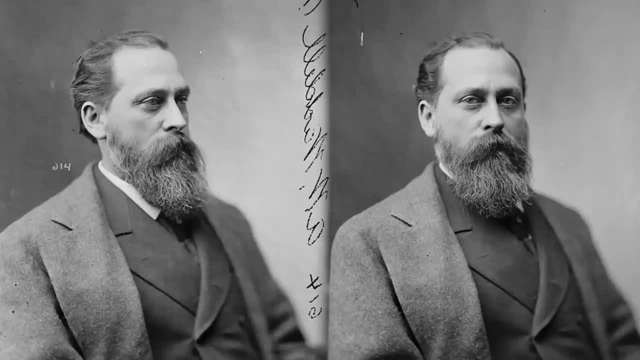 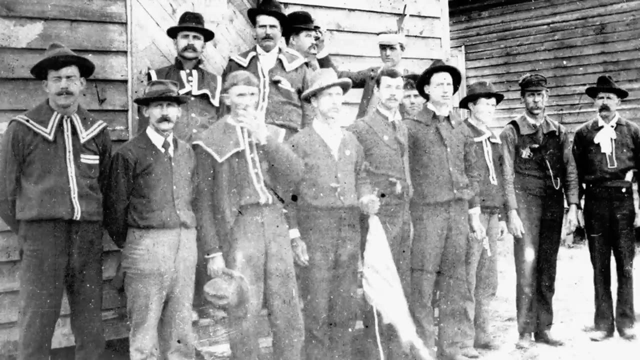 including a man named Alfred Moore Waddell, killed hundreds of black people in Wilmington, which was then the state's largest city, burned down the headquarters of the city's black newspapers and forced out the city's government, which was run by a biracial party known as the Fusionists. 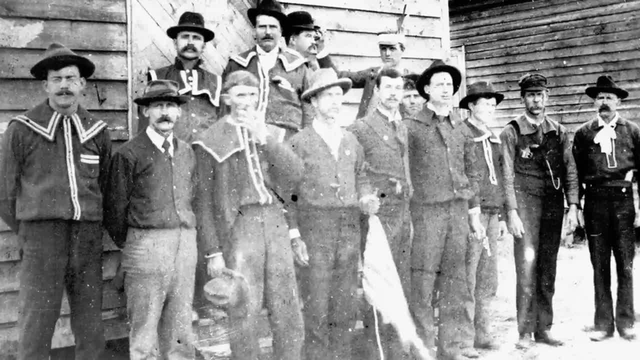 installing their own candidates. with Waddell, the leader of the coup, seizing the mayor's office, Many black people fled the city following the coup. By the time, job opportunities began opening up in northern cities. during the World Wars, many black southerners headed north in what was known as the Great Migration. 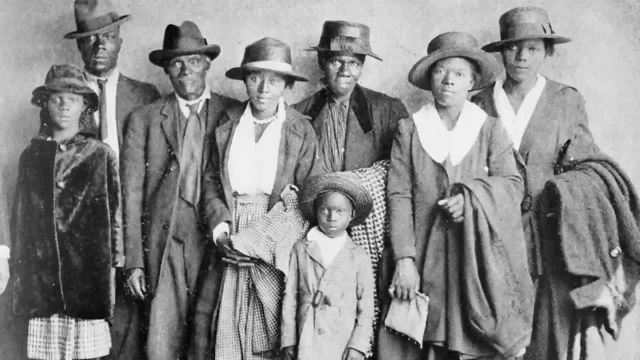 In North Carolina, black people went from making up 33 to 22% of the state's population due to this massive wave of emigration. One of the most prominent events of the Civil Rights Movement occurred in Greensboro in 1960.. 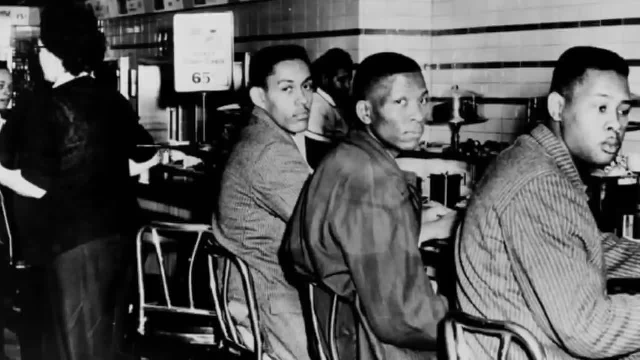 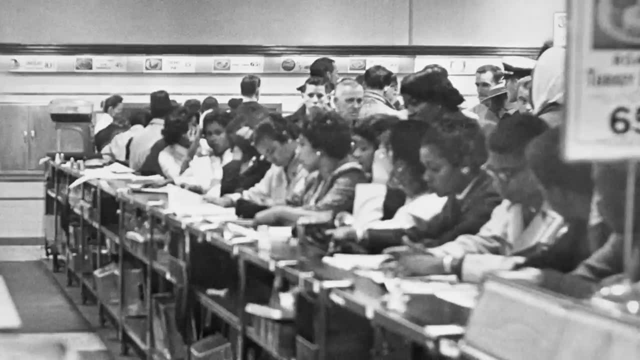 Four black students protested segregation by sitting at a segregated Woolworth's lunch counter. They stayed all day and over the next few months more people joined them, growing into mass protests and boycotts, with thousands of participants helping bring about the foundation of the Student Nonviolent Coordinating Committee. 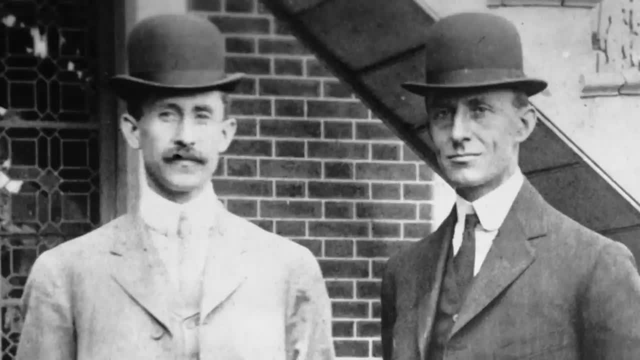 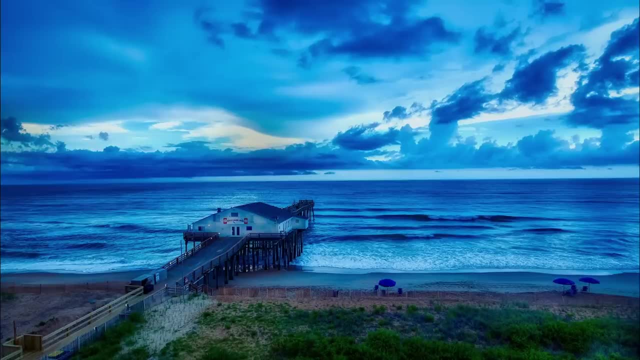 one of the most prominent organizations in the Civil Rights Movement. In 1903,, the Wright brothers made history in North Carolina by carrying out their first successful airplane flight in the Outer Banks town of Kitty Hawk. In the 1800s and 1900s. 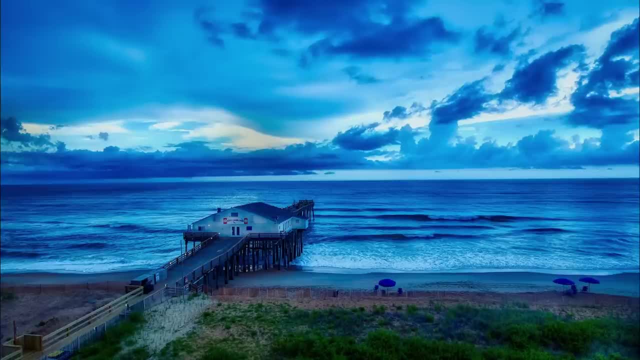 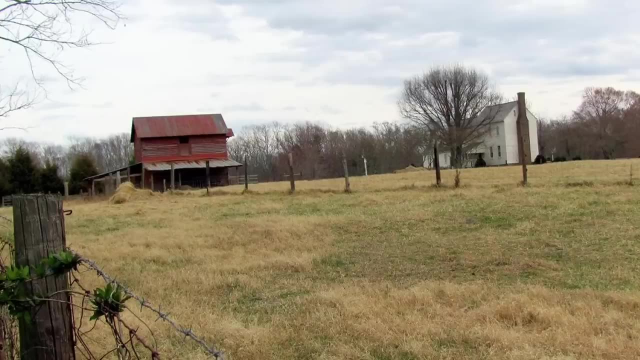 the state's population was still centered on the coast, and its largest cities were coastal ones like Wilmington and New Bern. However, during the 20th century, the Piedmont region grew to the center of population. it is today Mills developed along the fall line. 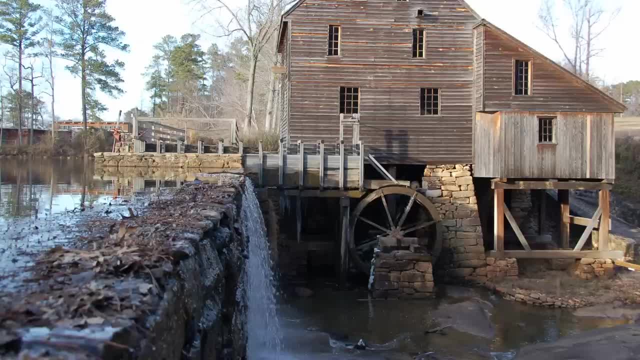 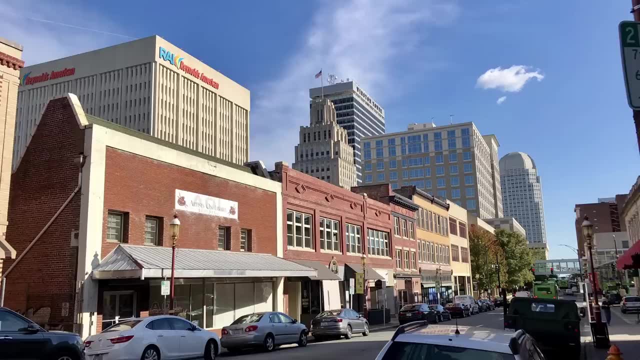 where the tobacco and cotton industries were able to industrialize and a major textile industry developed. Railroads helped fuel the Piedmont's rapid industrial growth, and cities like Charlotte, Winston-Salem, Greensboro, Durham and the planned capital city of Raleigh quickly grew into major urban centers. 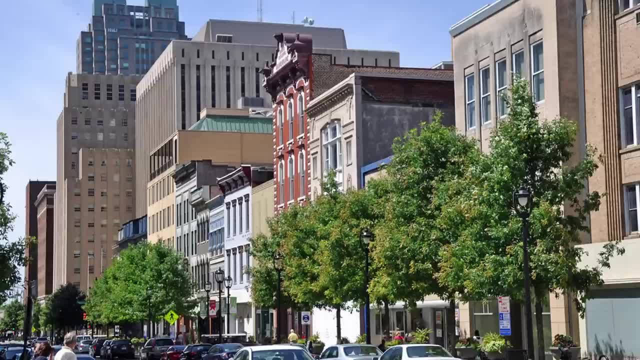 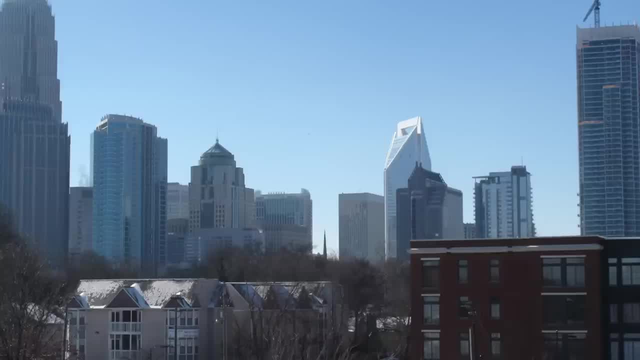 Turning North Carolina into the heavily populated state it is today and solidifying the Piedmont as its urbanized core. Charlotte became one of the country's largest banking centers, growing to be the state's largest city and the area around Raleigh, Durham and Chapel Hill. 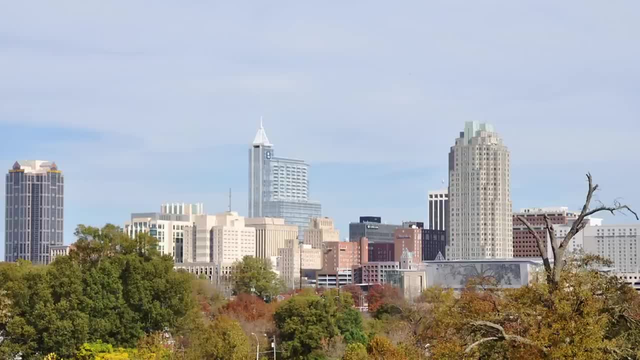 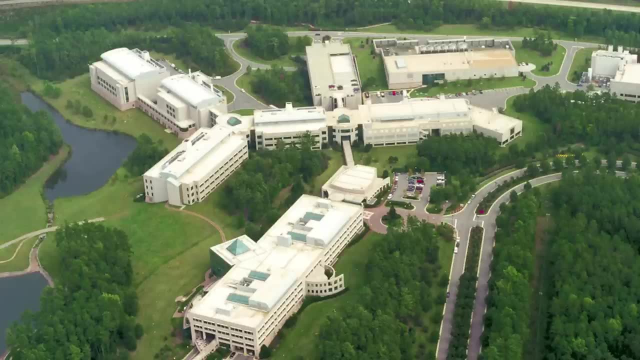 became a major center of research and technology, Thanks to being the home of a number of major universities, such as the University of North Carolina and Duke, as well as Research Triangle Park, the country's largest research park. The region is often just simply referred to as the Research Triangle. 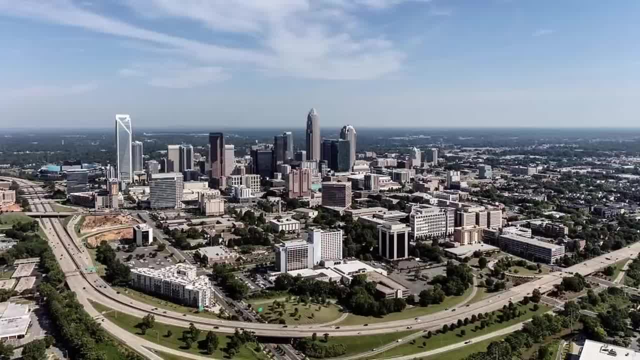 Charlotte is the largest urban area in the state, the 10th largest in the South and the 38th largest in the country, home to 1.2 million people. It's slightly larger than Providence and slightly smaller than Austin, Sitting in the Piedmont, not far from the border with South Carolina. 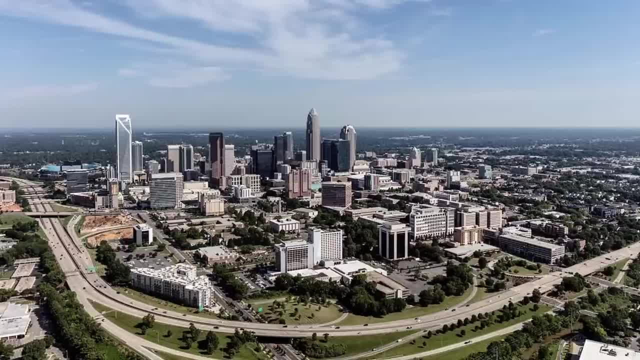 almost 300,000 people live in the Charlotte suburbs across the border, making it almost an urban center for both Carolinas. It's home to a large and beautiful skyline, including the Bank of America Corporate Center, the tallest building in the state. 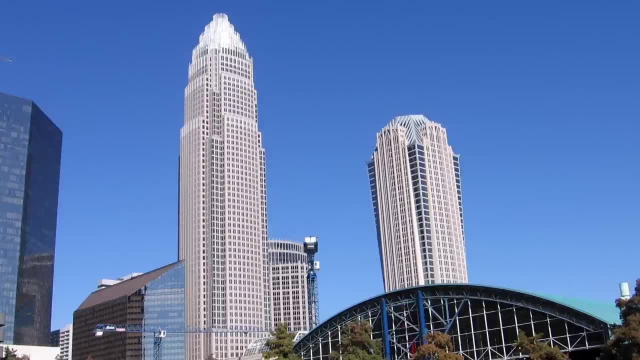 and the tallest in the South, outside Texas or Georgia. It's a national center of banking, the largest banking center in the US outside just New York City, due in large part to it being the headquarters of Bank of America, Other major banks like Wells Fargo and companies like Microsoft. 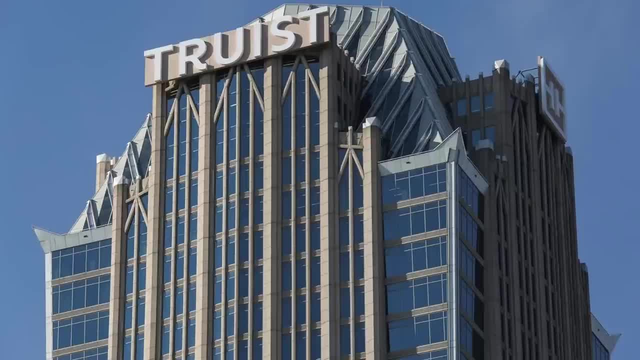 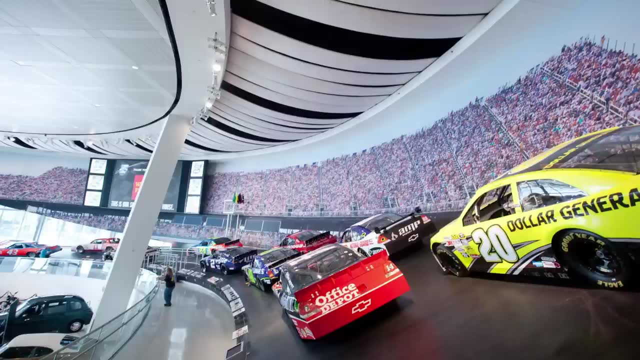 house regional headquarters in the city. Truist Financial, which owns BB&T and SunTrust, is headquartered in Charlotte as well. It's home to the NASCAR Hall of Fame and has in recent years been one of the fastest growing cities in the country. Named for British Queen Charlotte. it's nicknamed the Queen City. The name was given by British General Charles Cornwallis, who called it a hornet's nest of rebellion, which inspired the name of North Carolina's NBA team, the Charlotte Hornets Raleigh, North Carolina's second largest city. 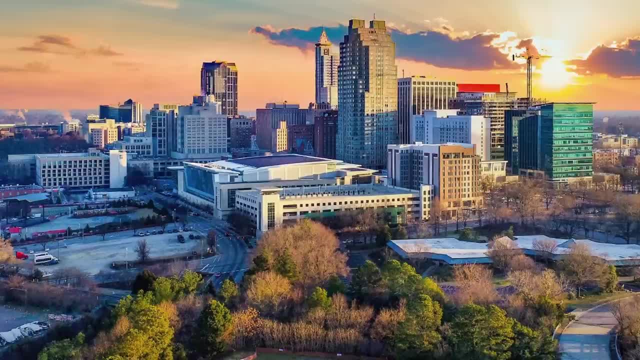 is the 50th largest urban area in the country, home to 885,000 people. It's the state's capital named for Walter Raleigh, the founder of the Roanoke Colony. A planned city, its location was picked out in 1788. 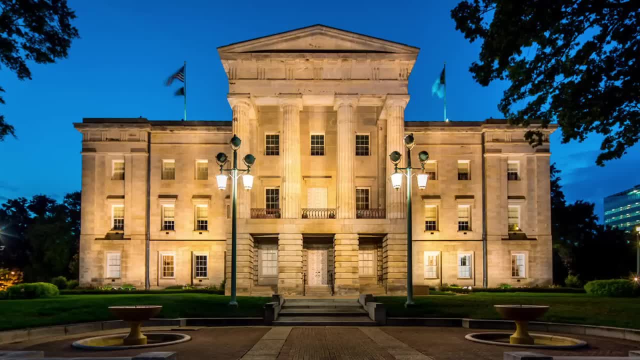 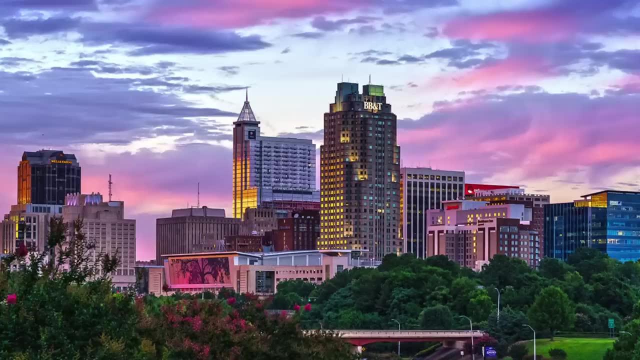 and was built in a grid surrounding the North Carolina Capitol building. If you pay close attention, you'll notice that Raleigh is one of the cities shown in my US Explained intro. It's home to a smaller skyline, not as prominent as Charlotte. 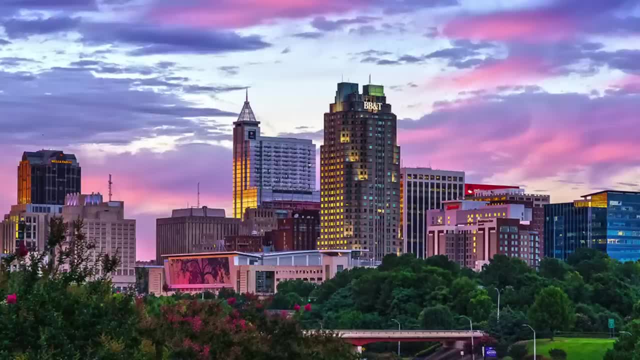 but is an incredibly fast-growing and economically prosperous urban area. The growth is driven by the Research Triangle, which consists of Raleigh and nearby smaller cities of Durham and Chapel Hill. Raleigh is home to North Carolina State University, the largest in the state. Durham is home to Duke University. 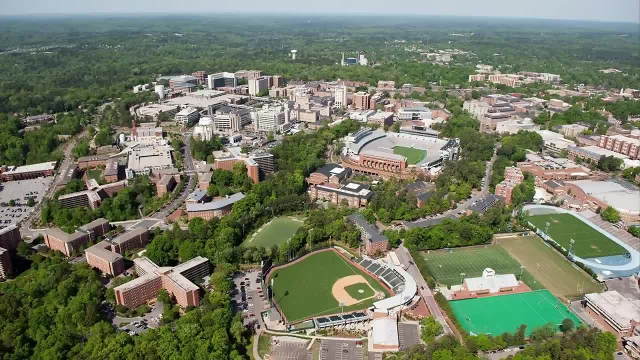 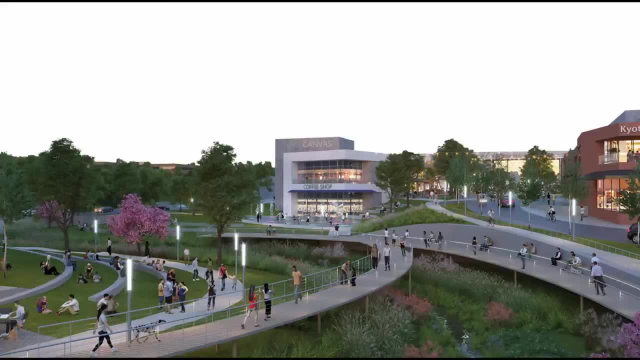 and Chapel Hill is home to the University of North Carolina. Many of these college graduates stay in and around Raleigh and work in high-paying jobs in research and technology. The Research Triangle Park, a research park created between the three cities, is the largest research park in the country and employs 60,000 people. 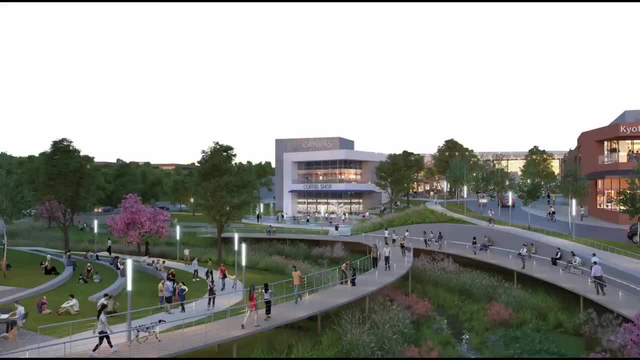 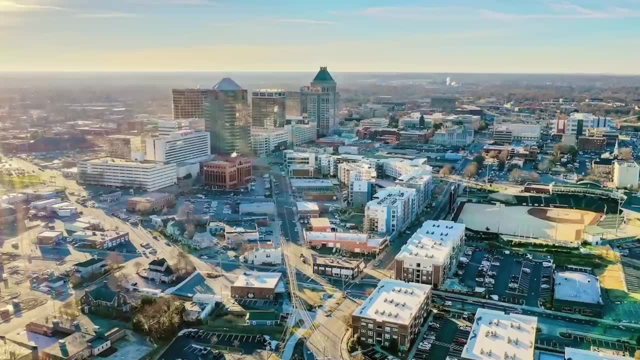 All of this has helped cement Raleigh as one of the most prominent tech hubs in the country. Out of North Carolina's smaller cities, Durham is tied closely to Raleigh and is known as the home of Duke University. Winston-Salem and Greensboro are tied closely to one another. 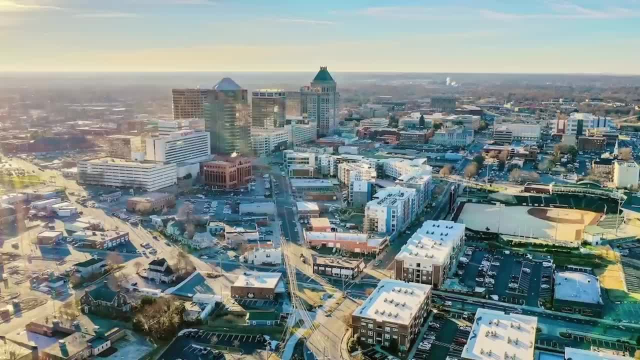 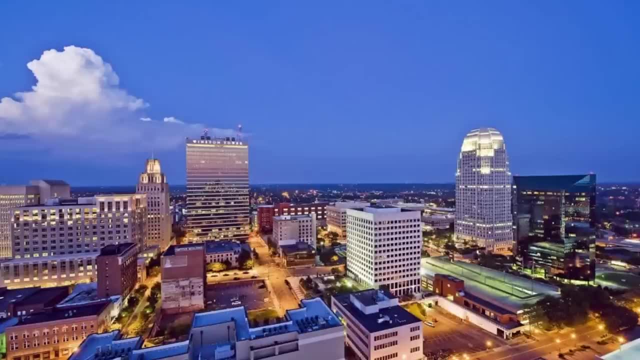 Greensboro is famous for its critical role in the civil rights movement, and Winston-Salem- once two different cities named Winston and Salem that later merged together- is a major center of tobacco manufacturing. home to RJ Reynolds, one of the largest tobacco manufacturers. 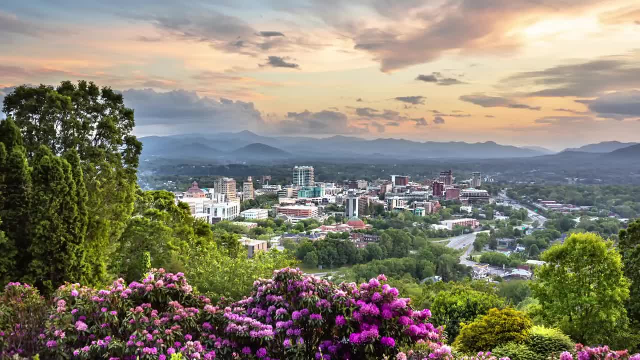 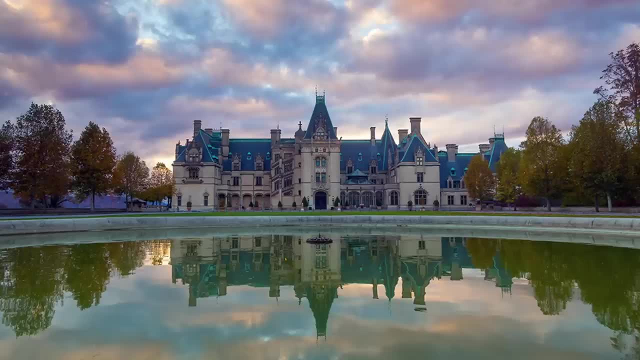 as well as the first Krispy Kreme. Asheville is famous for its arts and music scene and is a beautiful city nestled in the mountains. The Biltmore Estate, the stunning mansion in Asheville of the wealthy Vanderbilt family, is the largest home in the United States and one of the country's most visited houses. 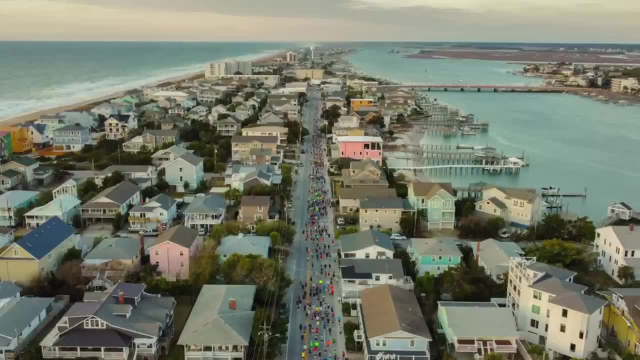 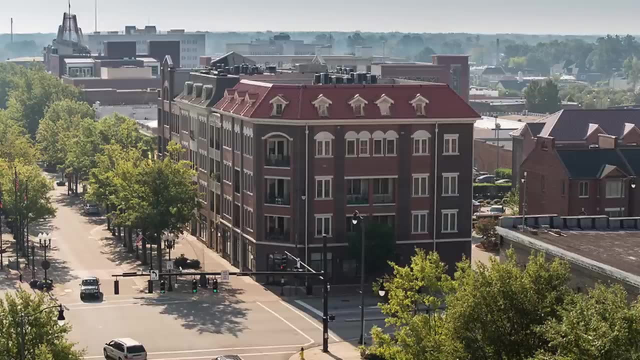 Wilmington is a major port city on the coast at the mouth of the Cape Fear River, and Fayetteville is known for housing the massive military base of Fort Bragg. I'm happy now to introduce a fan of the channel, a member of the- That Is Interesting- Discord group. 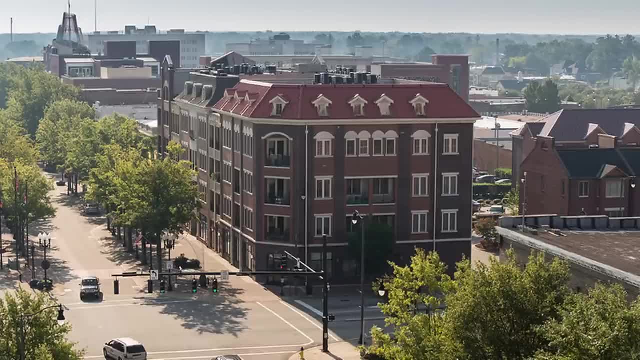 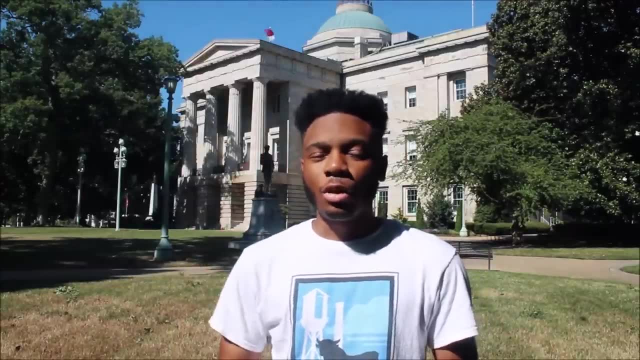 and one of my supporters on Patreon, DJ, to talk more about what it's like to live in North Carolina. Hey guys, my name is DJ and I'm coming at you from the state capital here in Raleigh. I really want to thank Carter for giving me this opportunity to be able to report my experiences growing up here in North Carolina. 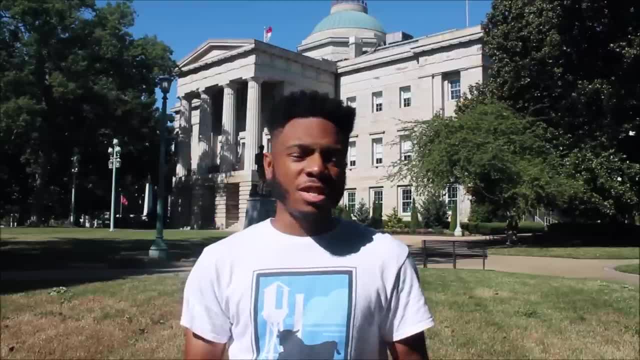 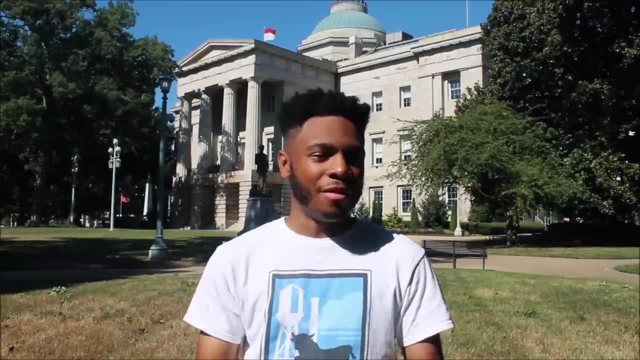 and just what life is like here in North Carolina. So although I spent most of my life in North Carolina, I was actually born in Philadelphia and a lot of the folks in the Discord community understand my Philadelphia roots and I really embrace those. 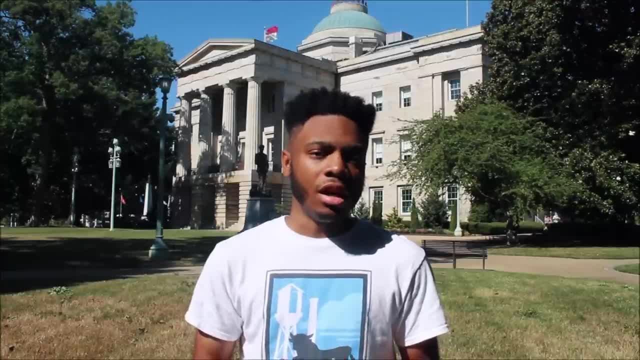 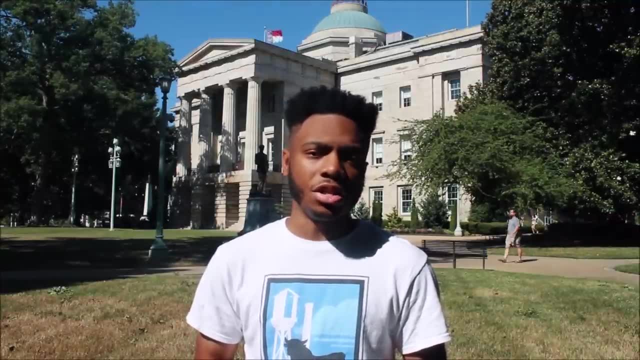 But I've spent 16 years In Durham specifically, And I've also spent some time in Raleigh and Cary, And I also lived for four years in Charlotte while I was getting my undergrad at UNC Charlotte. So growing up here has been, I think, a pretty good experience. 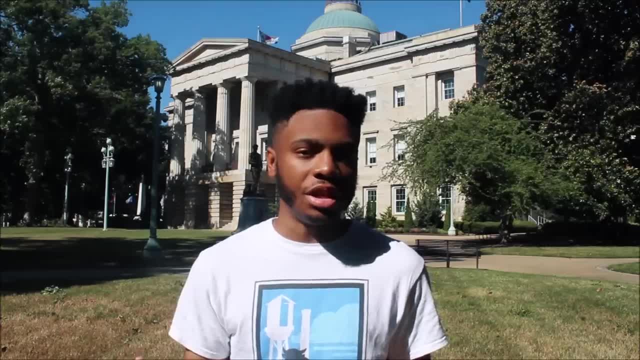 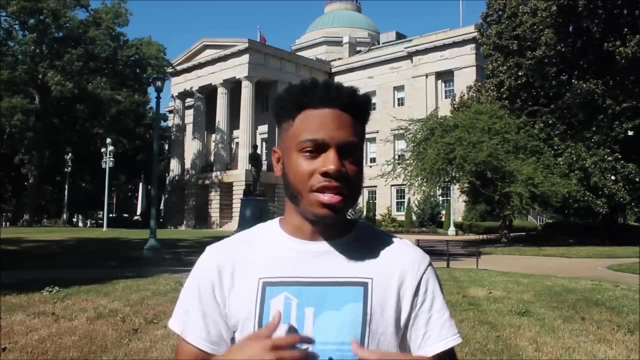 There's a lot of great people that live in North Carolina. No matter what part of the state that you're in, you're going to get that Southern hospitality that North Carolina and much of the South is known for- Two of the biggest things that I guess especially the Triangle region is really acclimated to. 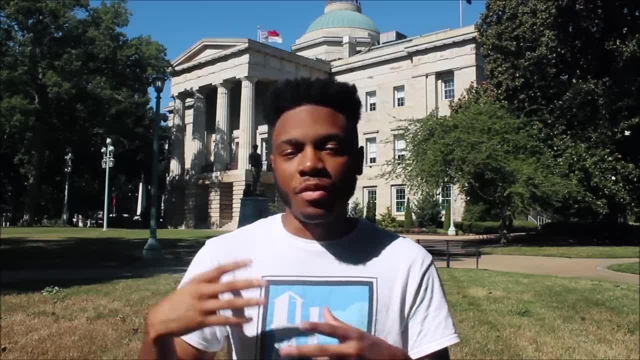 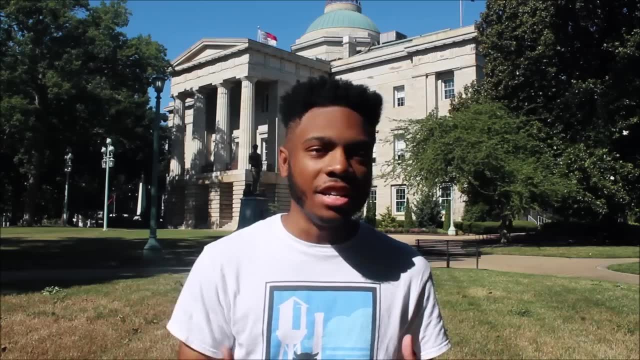 is basketball and barbecue. We have UNC, Chapel Hill, We have Duke University in Durham And then we have North Carolina State in Raleigh. All of the basketball teams are always fighting to be at the top, And no matter where you are, no matter what time of year it is. 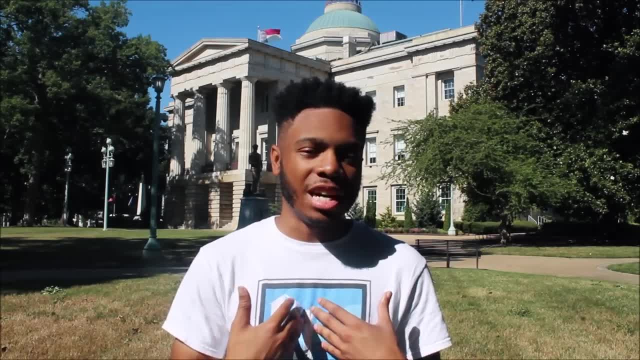 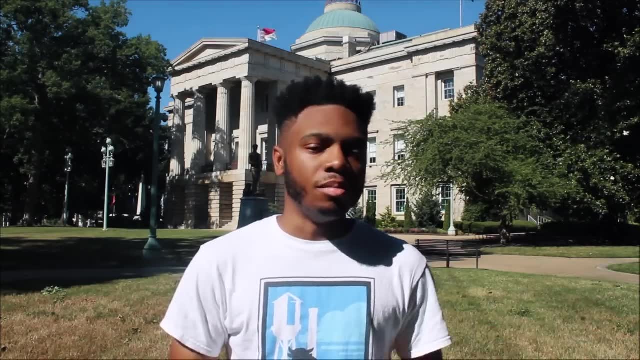 you're always going to get into some kind of argument about which team is better. Me personally, I grew up a UNC Chapel Hill fan. My mom went to school there, got her undergrad there, And I have multiple family members that have gone there as well and gotten their master's degrees and such. 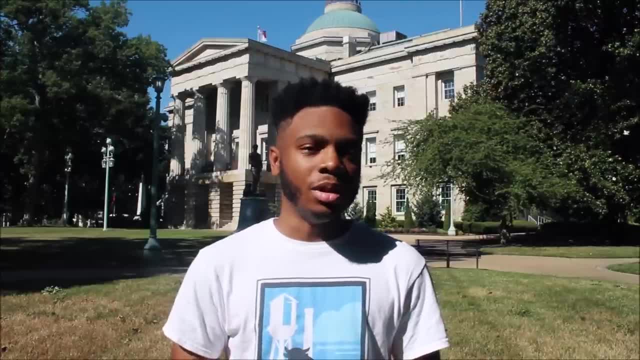 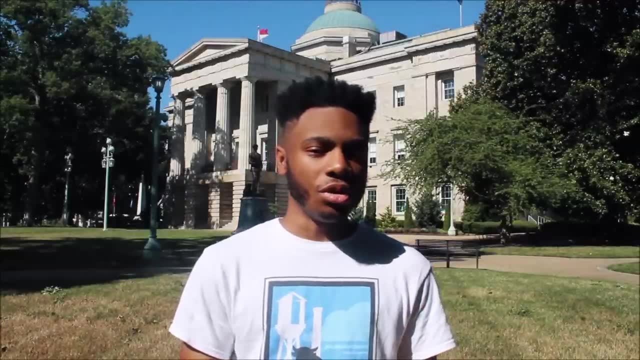 So me personally, I love Chapel Hill, I love Carolina, Carolina Blue, But basketball is such a huge topic here. So another thing about North Carolina is that I feel like we're very spoiled because a lot of our famous tourist destinations and vacation places are all connected. 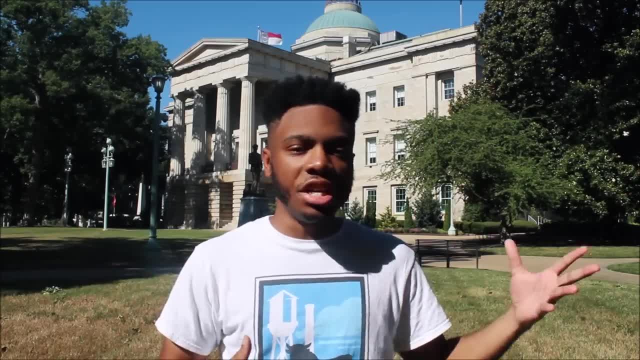 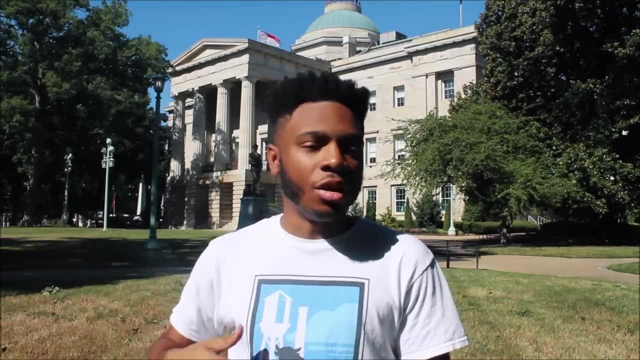 We're all right in the middle of everything. So you have the beach in Wilmington or the Outer Banks, You know. that's no more than a three-hour drive away on I-40.. We can also go in the other direction on I-40 and go to Asheville and the Blue Ridge Parkway. 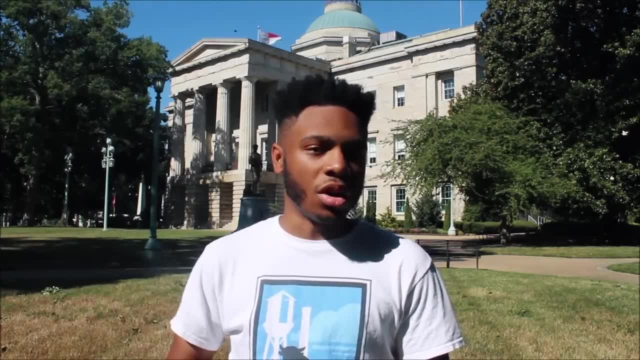 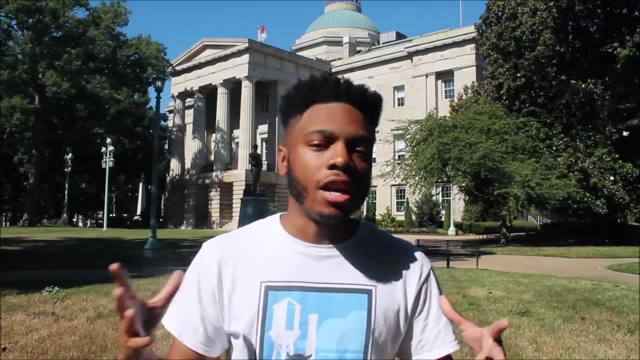 and Grandfather Mountain and all those mountains that are out in the western part of the state, And then right in the middle you have Raleigh and you have all the other cities that are also within the Piedmont and Triangle triad regions of the state. You have Raleigh here, which is like the eastern end of what's called the urban crescent. Go further west, you hit Durham, You hit Greensboro And then, once you get down south, you hit Charlotte. Charlotte's our largest city. 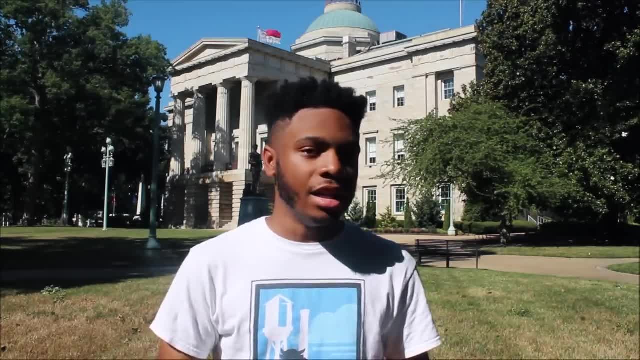 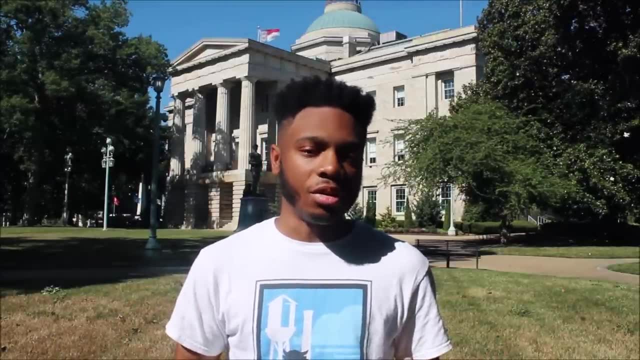 We have professional sports teams in the Carolina Hurricanes playing here in Raleigh. We also have the Charlotte Hornets and the Carolina Panthers down in Charlotte professionally. So anything you want, we've got it here in North Carolina. And one other thing: me being a transportation nerd, I really look at what kind of transportation options we have here. So, growing up in Durham but going to school in Charlotte and coming to see my family here in the Triangle a lot, I would always take Amtrak between Charlotte and Durham and sometimes Raleigh. We have multiple trains a day that go between the two cities and that stop at all the towns in between. 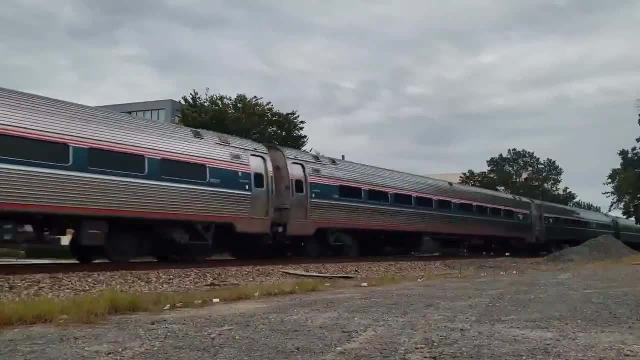 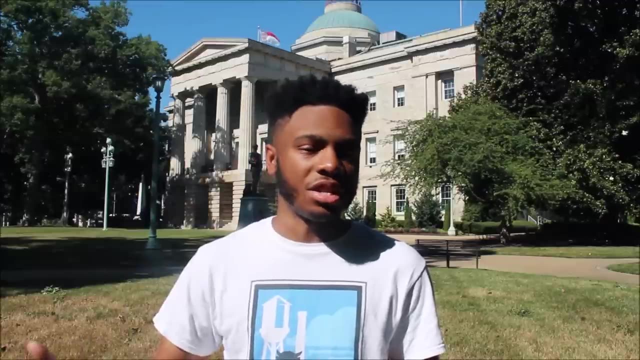 So it's a really good type of service to have, especially here in the state, where we're one of the fastest growing states in the nation And we have two of the fastest growing cities with Raleigh and Charlotte, But also Durham as well, very fast growing. 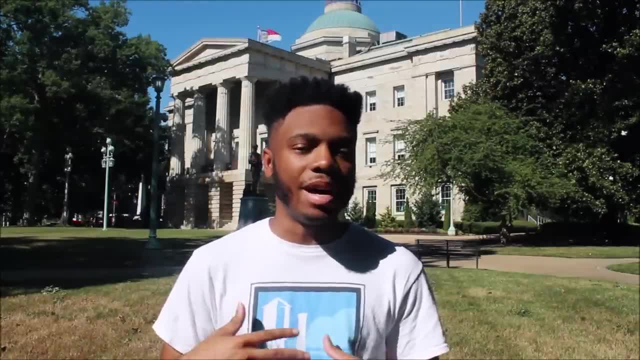 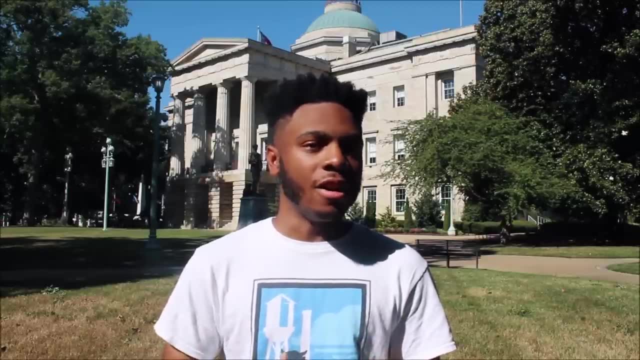 We really have everything here in North Carolina. I'm very excited that I'll be able to share my experiences with you all and hope you enjoy the rest of the video And make sure to join the Discord community. We have a great community of folks that are interested in topics such as geography, but also sports, politics, maps. 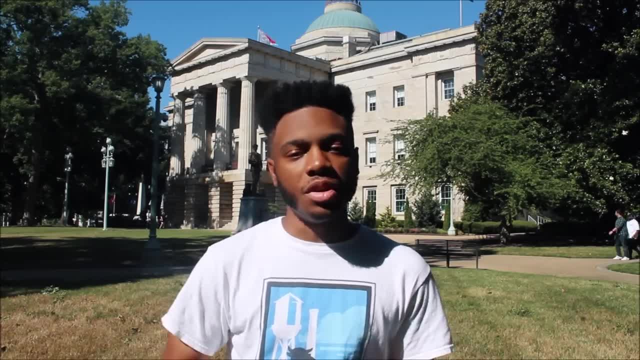 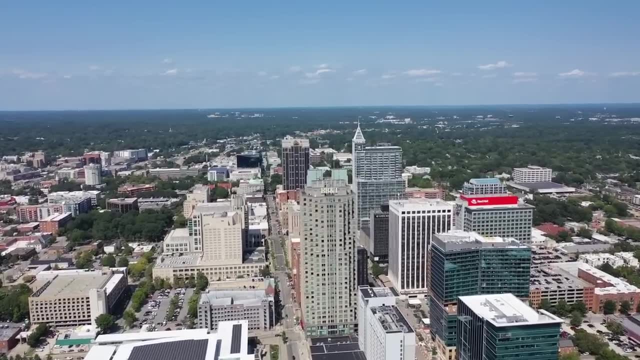 and pretty much anything you want to talk about we have right there in the Discord community, So feel free to join and again enjoy the rest of the video, Thank you. North Carolina is quite racially diverse: 64% of its population is white and 22% are black. 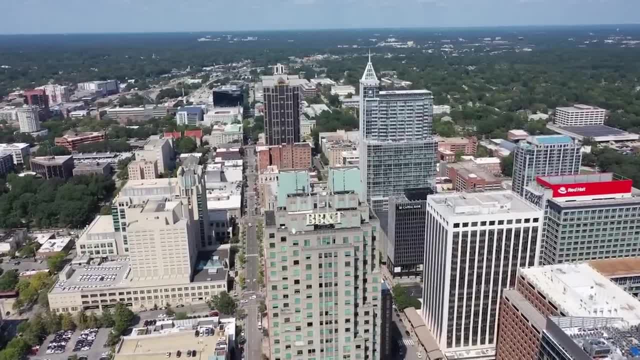 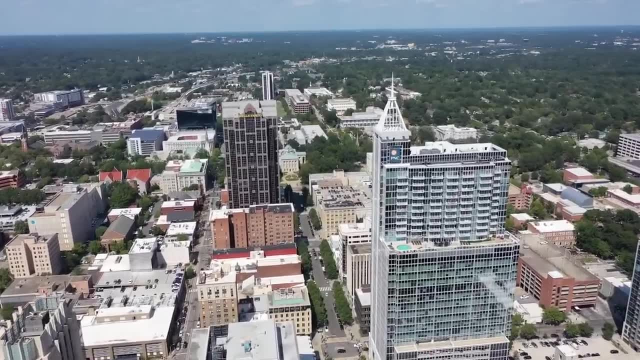 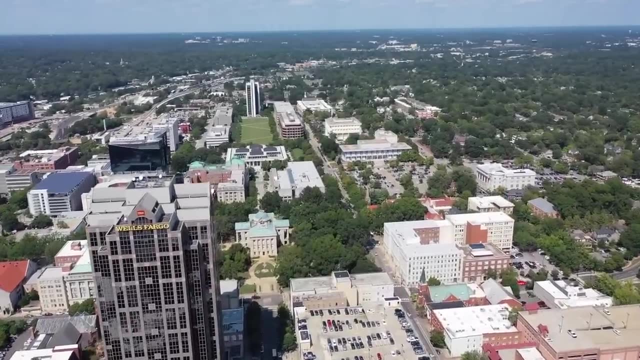 That gives North Carolina the 8th highest percentage of black residents of any state. In terms of sheer numbers, due to the state's large population, it has the 6th most black residents in the country: 10.7% of North Carolinians are Latino, 4% are Asian American and, due to its large Lumbee population, 2.5% are Native American. 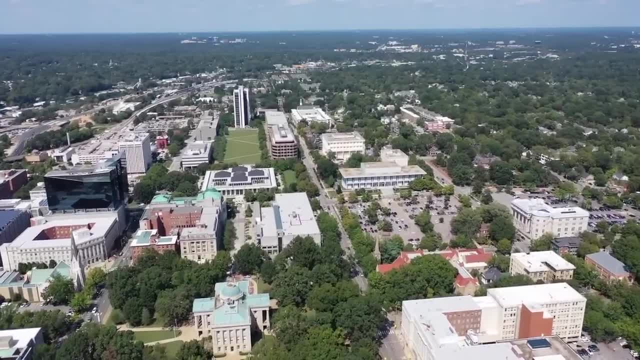 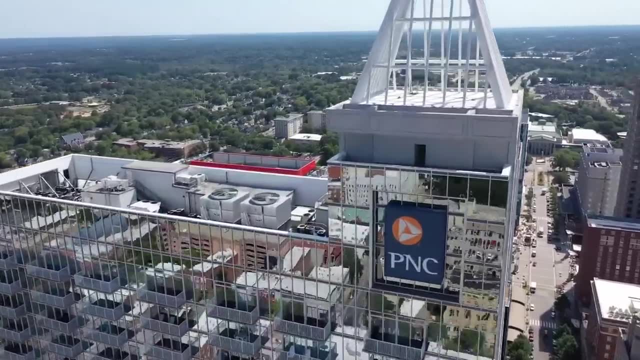 The largest population of any state fully east of the Mississippi. Religiously, Christianity dominates in the state, with 78% of North Carolinians practicing Christianity. 2 thirds of the state's residents are Protestants, About half of whom are Evangelicals, the state's largest religious group. 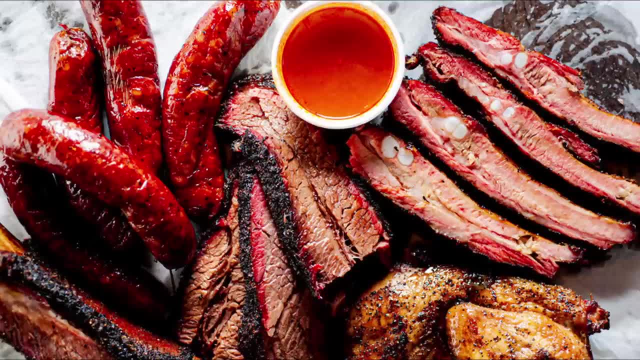 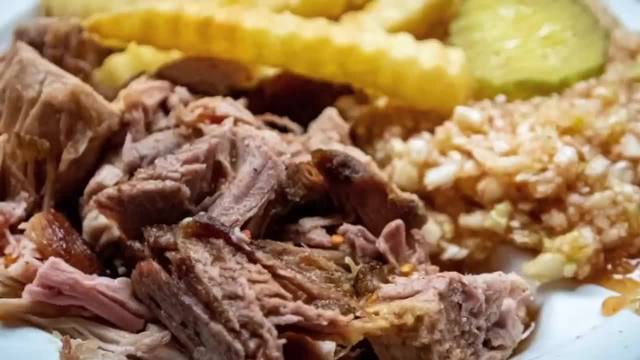 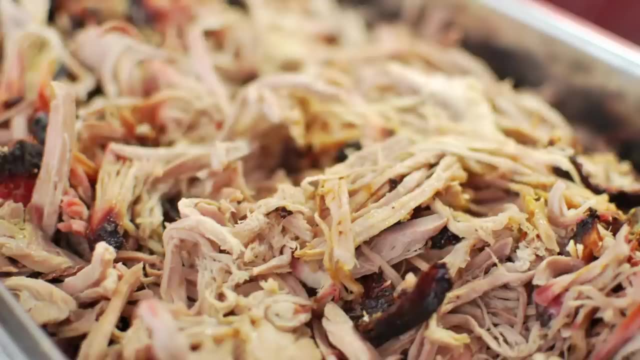 North Carolina is home to two unique styles of barbecue that line up with the state's regional divides. In the Piedmont and Appalachians, Lexington-style barbecue using pork shoulder in a vinegar and tomato-based sauce is common, whereas in the eastern coastal, plain eastern style is used, making use of the entire hog and using a clearer vinegar-based sauce. 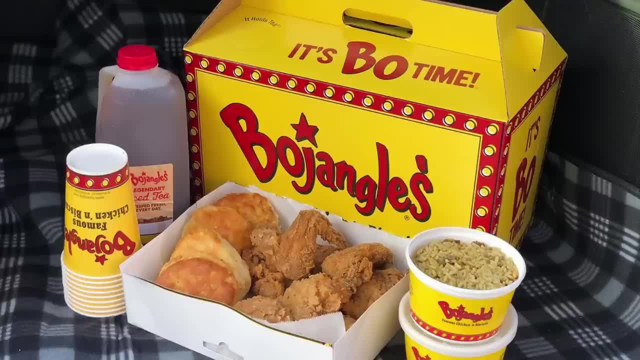 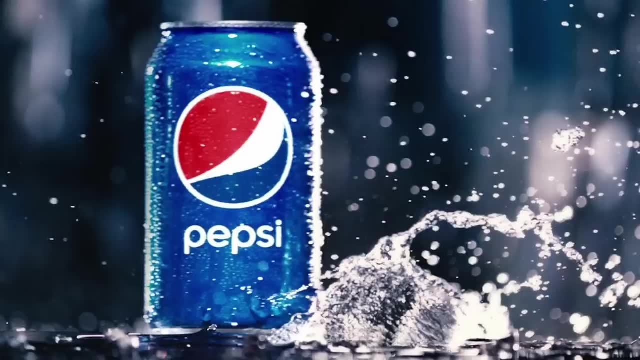 Popular southern fast food restaurant Bojangles is based out of Charlotte and Cheerwine, a cherry-flavored soda, is popular locally. In addition, the fast food chain Hardee's is based out of Greenville and Pepsi was founded in New Bern. 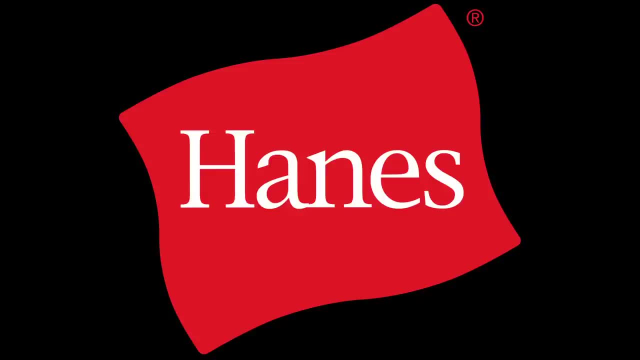 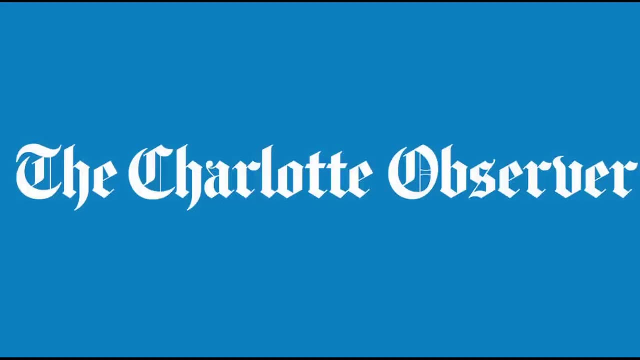 Other major companies like Lowe's and Hanes are based in North Carolina, as well as the North American headquarters of Compass Group, the world's largest food service company. The largest newspaper in the state is the Charlotte Observer, followed by the Raleigh News and Observer. 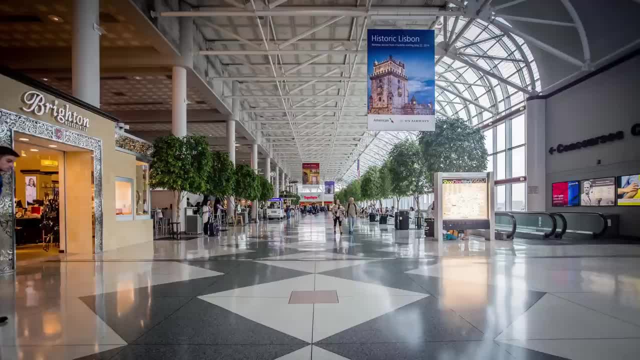 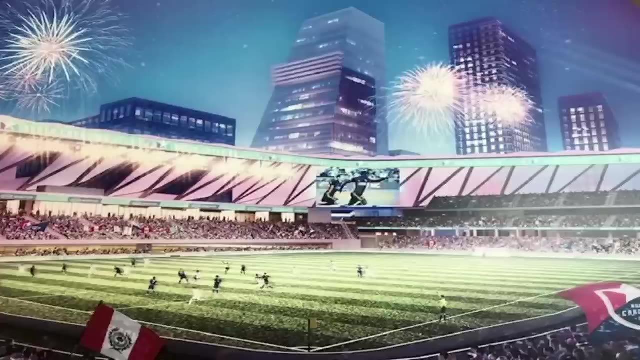 Before COVID, Charlotte had the 11th busiest airport in the US, the Charlotte Douglas International Airport, with 24 million passengers. Raleigh-Durham is also home to an international airport, as are Wilmington and Greensboro. North Carolina has one of each major league football, basketball, hockey and soccer team, but no major league baseball team. 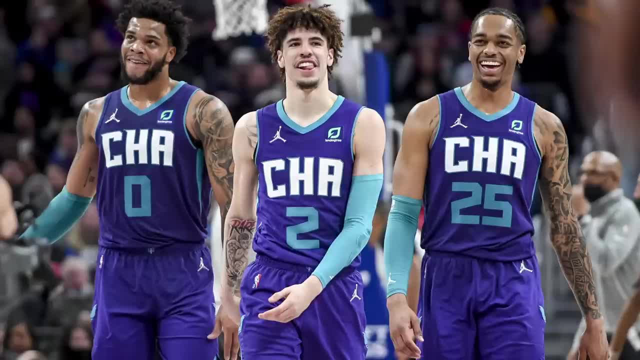 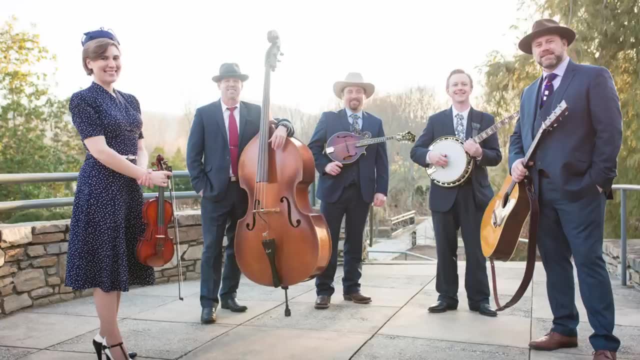 Charlotte is home to the NFL's Carolina Panthers, NBA's Charlotte Hornets and MLS's Charlotte FC. Raleigh, in addition, is home to one major league team, the NHL's Carolina Hurricane Jazz. bluegrass, country blues and country music all have deep history in the state. 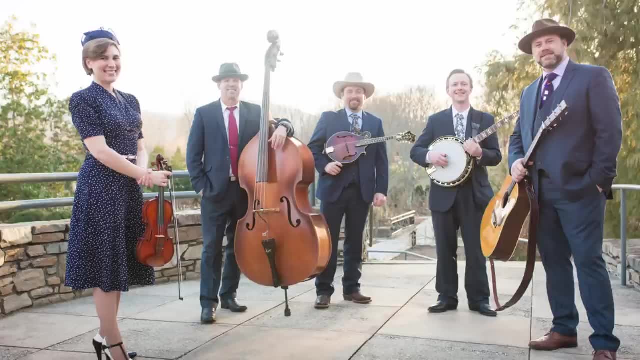 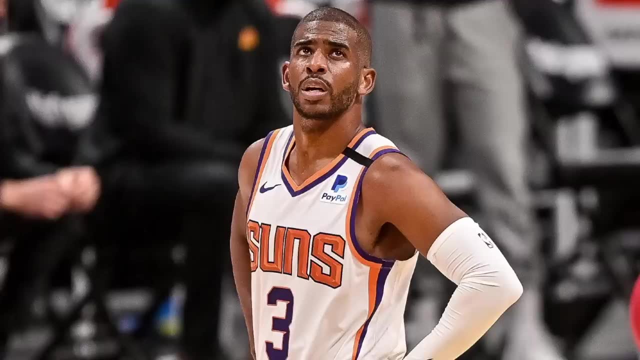 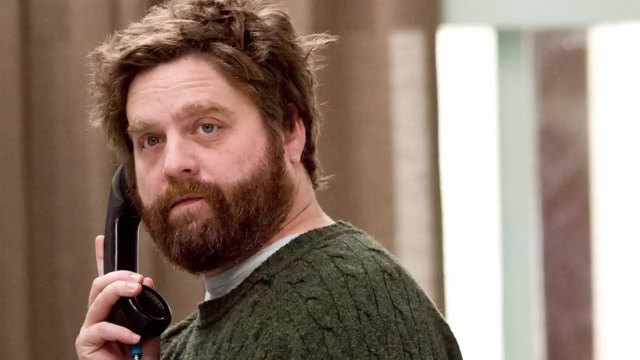 Many famous people were either born or raised in North Carolina, including musicians like J Cole, Luke Combs, Doc Watson and Nina Simone, Basketball players Michael Jordan, Chris Paul and Steph Curry, NASCAR legend Dale Earnhardt, famed evangelist Billy Graham and actors like Andy Griffith, Zach Galifianakis and Ken Jeong. 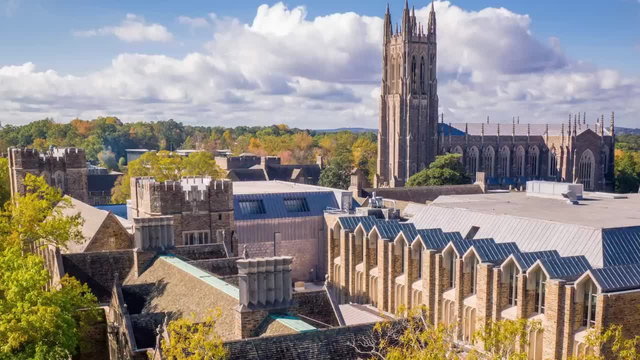 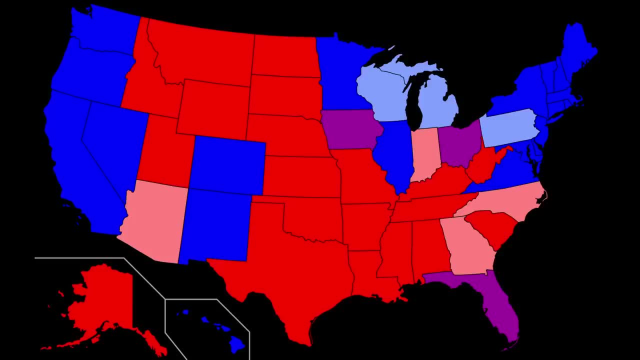 It's home to a number of major colleges and universities, such as Duke in Durham, UNC in Chapel Hill and Wake Forest in Winston-Salem. Politically, North Carolina is a light red state. Two or maybe three presidents were born in North Carolina, but interestingly, all three of them launched their political careers from Tennessee. 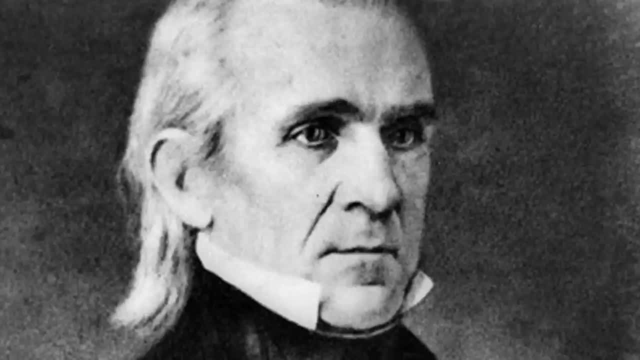 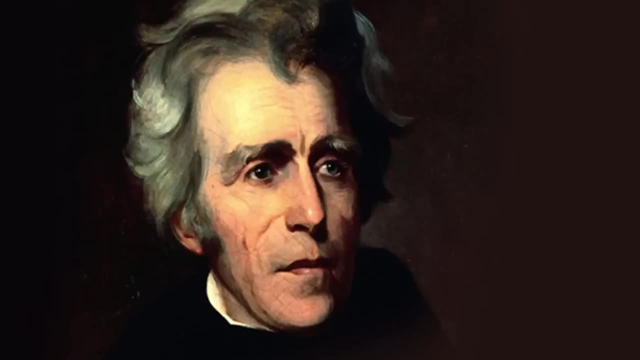 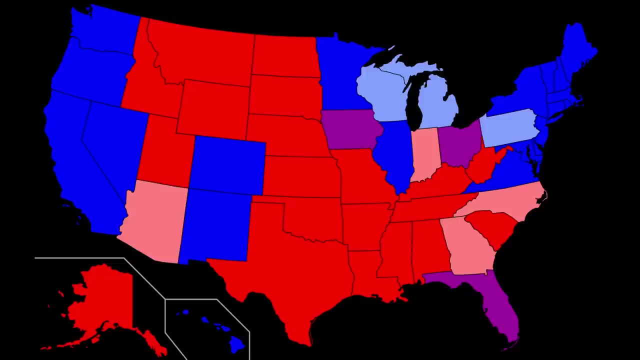 James Knox Polk was born in North Carolina. He was born in the town of Pineville, now a suburb of Charlotte on the South Carolina border, and Andrew Johnson was born in Raleigh. Andrew Jackson was born somewhere along the North and South Carolina border and it's still unclear which state he was actually born in, though he considered himself to be from South Carolina. 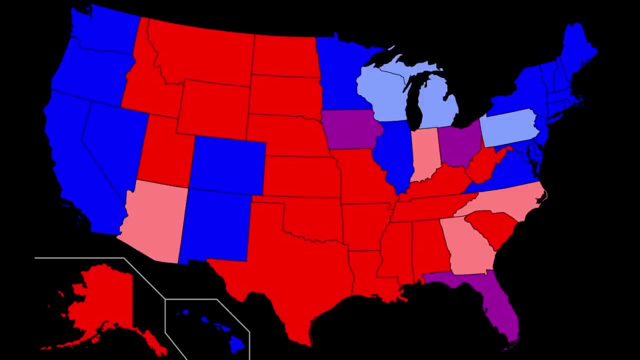 North Carolina has a Cook PVI rating of R plus 3, meaning that in a given election, North Carolina tends to vote for Republican candidates by about 3% more than the US. on average, This is about the same as Georgia, Florida and Arizona. 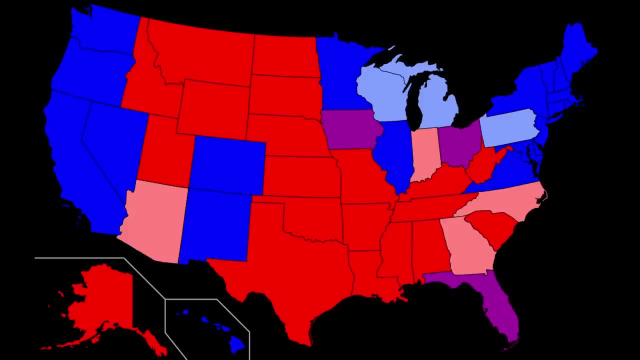 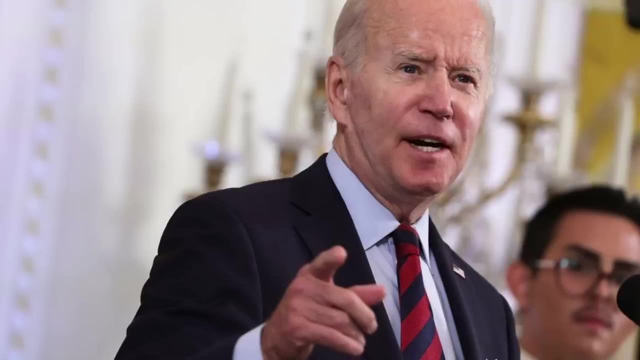 And while North Carolina stands out from the rest of the US, North Carolina is the only state in the US that has the highest vote count And, while North Carolina certainly leans Republican, this makes it a somewhat competitive state In the 2020 election. for example, Donald Trump won the state over Joe Biden by just 1% and Barack Obama won North Carolina in 2008, but lost it in 2012.. 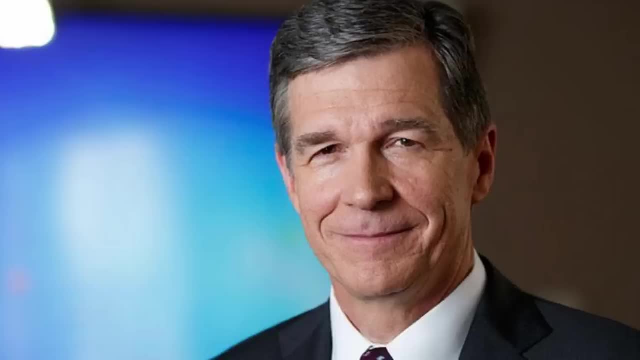 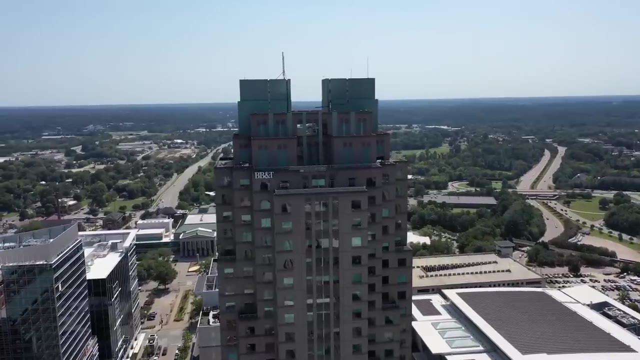 The state has traditionally elected Democrats to be governor. The current governor, Roy Cooper, is a Democrat, and the state's two senators, Tom Tillis and Richard Burr, are both Republicans. That is it for North Carolina. I want to give a big thank you to everyone who has already joined my Patreon. 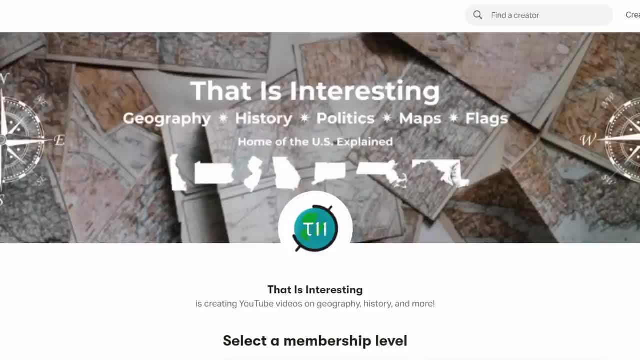 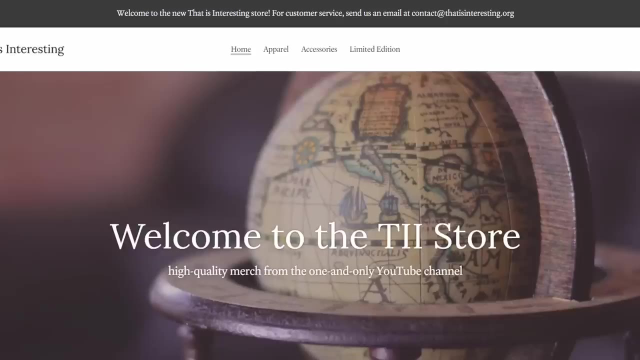 Through it, you can access different things, such as behind-the-scenes videos, early access to maps. I create an exclusive Discord Q&A with me, ad-free content and shoutouts in my videos. Please be sure to check out the TII store, where you'll be able to purchase all sorts of official- That Is, Interesting- products and merchandise, including shirts, hoodies, embroidered beanies, masks, mugs, embroidered backpacks, laptop stickers and sleeves, and so on. 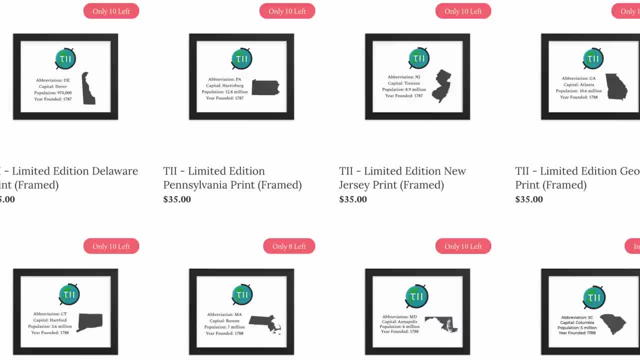 One of the products I'm most excited about are these limited-edition frame-state prints that commemorate each video in The US Explained. These are available as soon as the corresponding US Explained video is uploaded, but only 10 of each will be released, so make sure to buy one before they go out of stock. 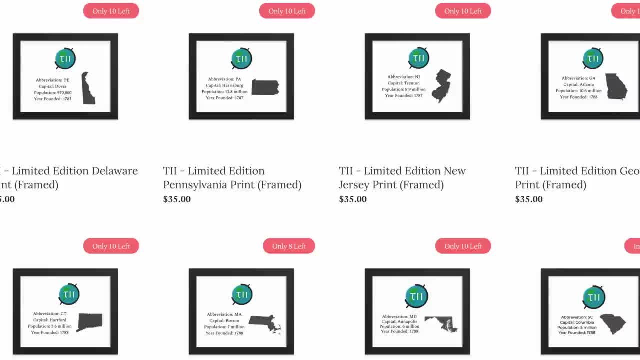 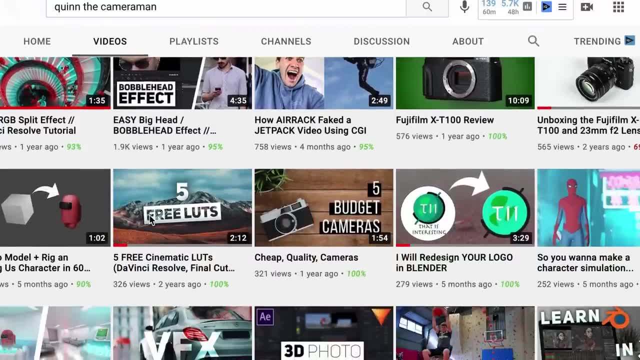 Right now you'll be able to buy a North Carolina state print, so please click the link in the description and go pay a visit to the TII store. Also, please subscribe to my brother's channel, Quinn the Cameraman. He made this great intro at the beginning of this video that I'll use in all of the US Explained videos and to help with the editing. so go show him some support. 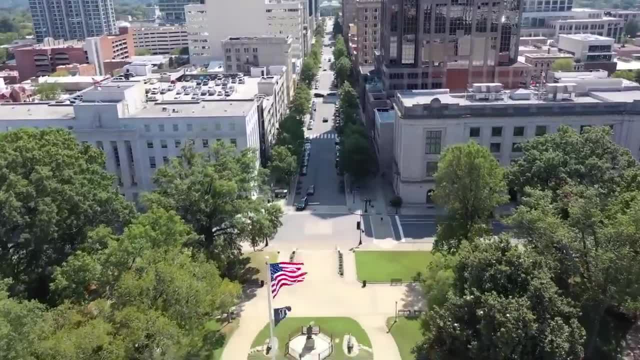 I tried to be pretty thorough with this video, but I know there were definitely things I missed, as there was a lot of stuff I missed. I want to give a big thank you to everyone from North Carolina who helped give me information for this video. 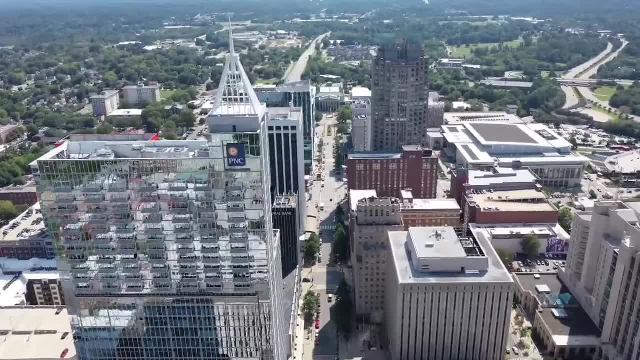 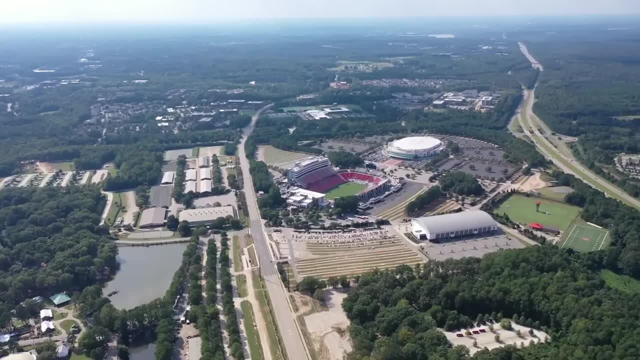 leaving detailed and informative comments on YouTube as well as Discord. I truly would not have been able to make this video without all your help. My next video in this series will be on Rhode Island, the last of the 13 colonies. I've been able to visit Rhode Island, but I'll still need all the help I can get. 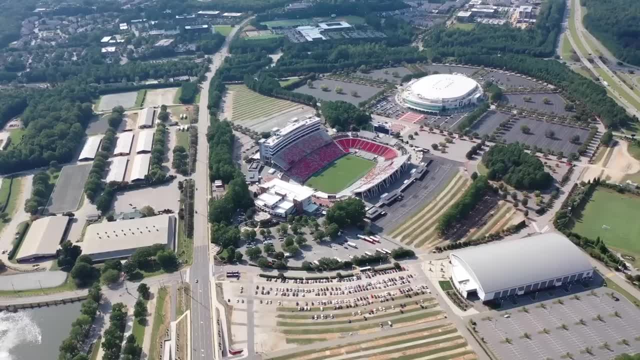 If you're from Rhode Island, please respond to my community post or my comment here, or leave something in the Discord server to let me know what you'd like to see included about your home state. I really appreciate the well over 4,000 subscribers.